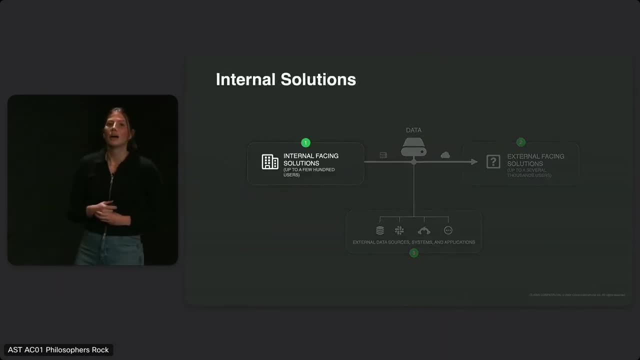 really quickly. So here at Clarus, we do believe that FileMaker is ideal for building solutions that can scale to hundreds of users, that can be deployed wherever work is done and your problems can be solved. You all have proven this to us over the past 35-plus years. 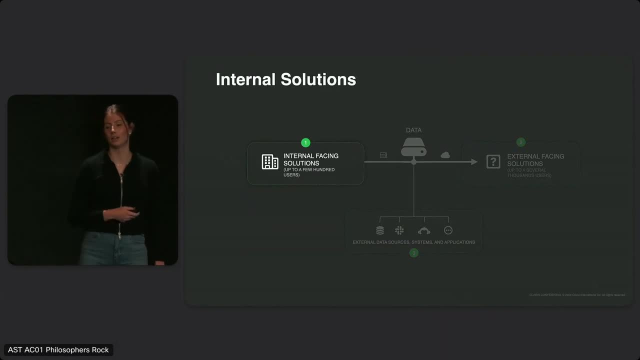 and we'll always continuously make improvements to FileMaker For new requirements. That being said, as Giuliano mentioned in the keynote, there's also an important set of requirements that go to externally facing users that have different requirements from internal. First, they can't rely on operating systems or specific installed. 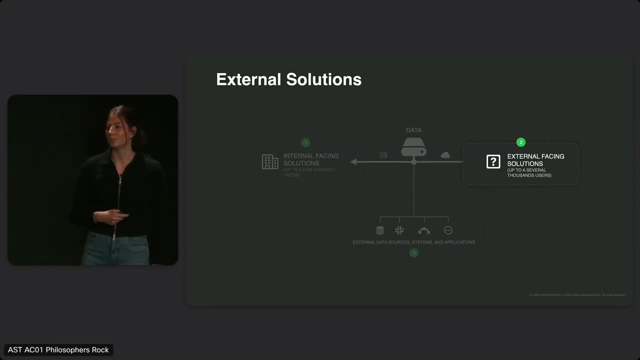 apps. They have to be responsive, native web applications. And second, external audiences can have the opportunity to deliver their own social networks. and then these essential can be of unpredictable size. They might be very large or they may have to scale gracefully. 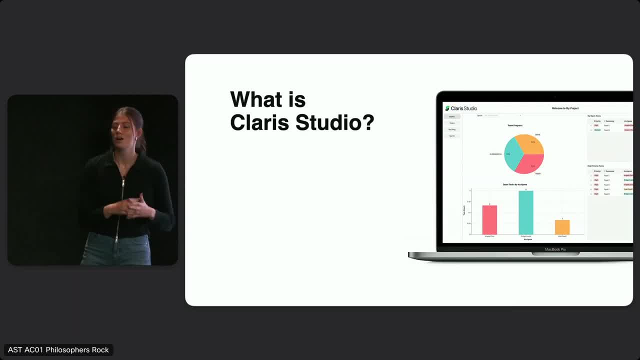 So with that enters Claris Studio. Claris Studio, we want you to have another tool in your developer toolbox. Just like you wouldn't try and saw a piece of wood in half with a hammer, you probably wouldn't use FileMaker to build a responsive native web application. 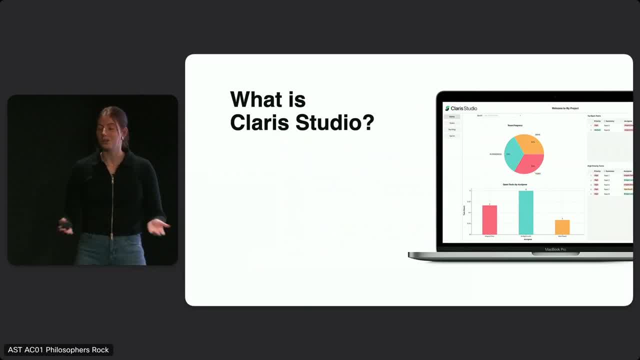 that can scale gracefully Well. you could, and I'm sure a lot of you have, But it may take a very long time. With Claris Studio, we wanted to bring you the developer a modern UI application that's built on an entirely new tech stack. 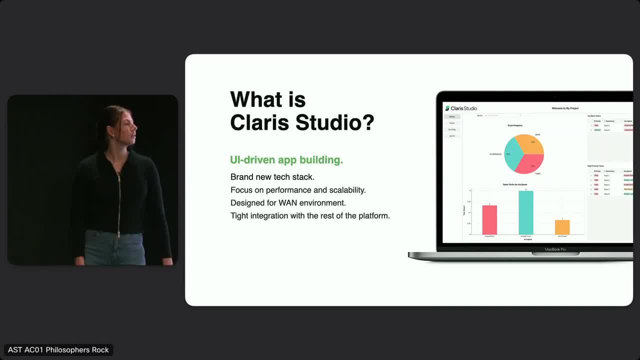 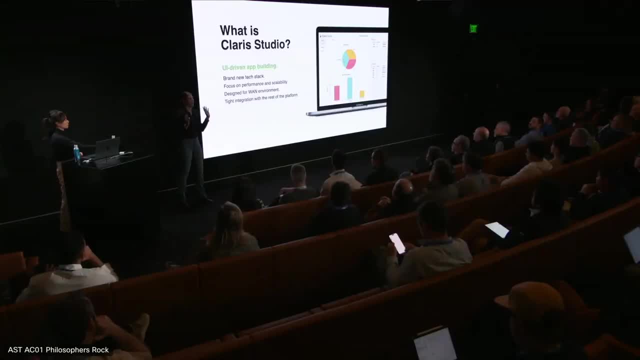 MongoDB and Reactjs. that's focused on performance and scalability and tightly integrated with the rest of our platform. But I know you might be thinking she just threw out a lot of buzzwords. What does that mean? What does that mean to me? 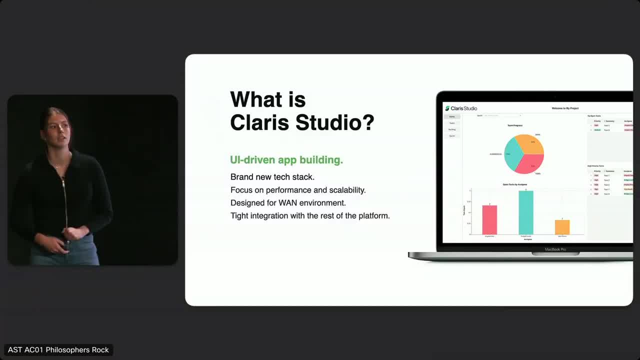 How can I, as a developer, leverage this solution? And I'll answer that question with a story. Remco van Buuren from OpenSea came to Studio with an anonymous data collection use case to get data for his FileMaker solution. But no one tells that story better than Remco van Buuren. 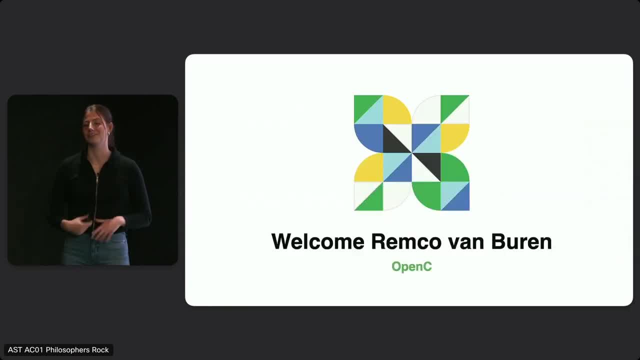 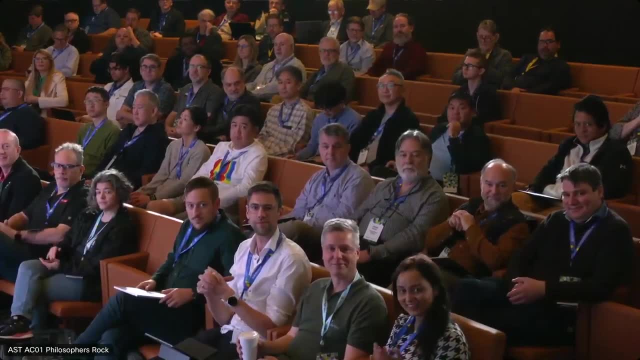 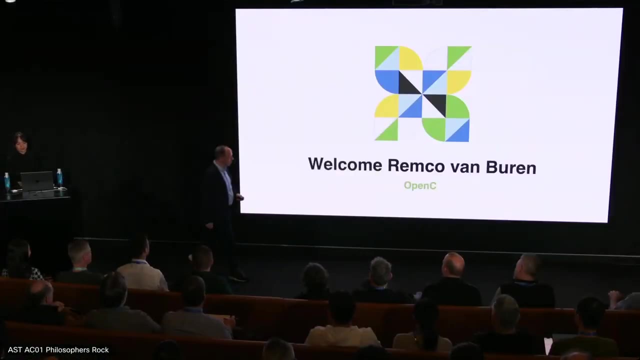 So I'm gonna bring him out right now to tell that story for you all. Thank you, Bridget. My name is Remco van Buuren. I'm from a company called OpenSea. I'm from the Netherlands And for the last 30 years, 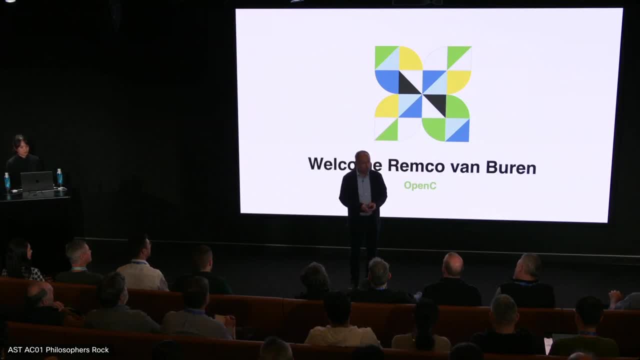 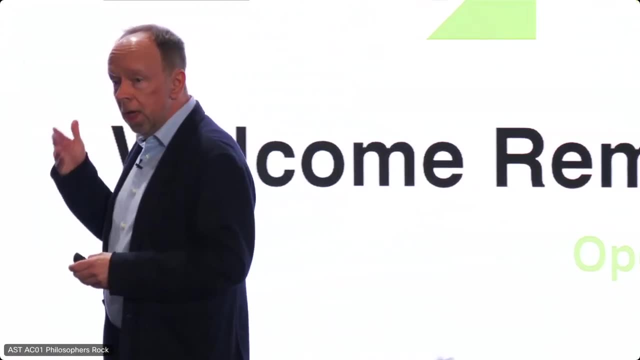 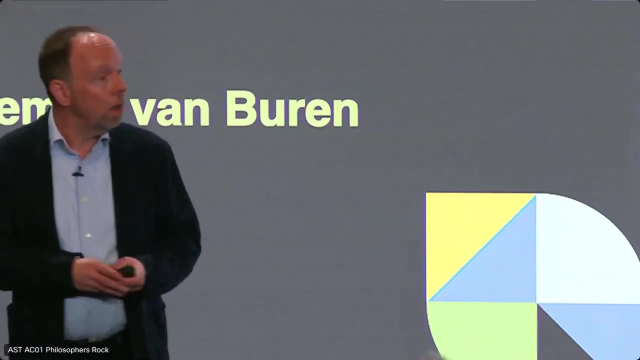 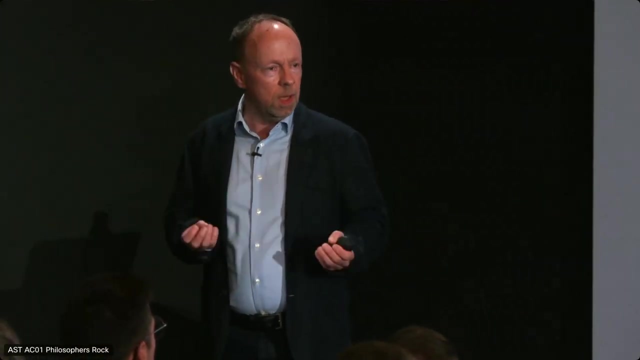 I've been working in senior management position with insurance companies, So insurance is my background, but also always combined with IT, And I have also an IT background in education. So And 10 years ago I founded the company OpenSea that we're working now with in the Netherlands. 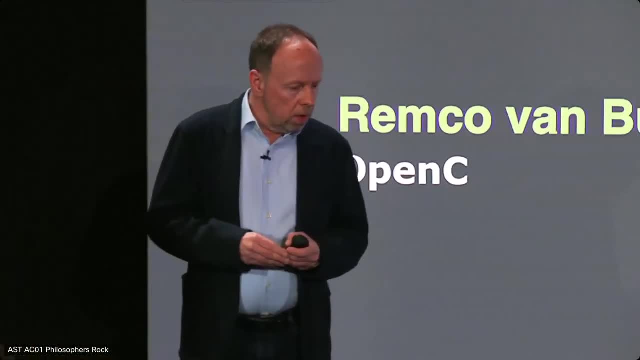 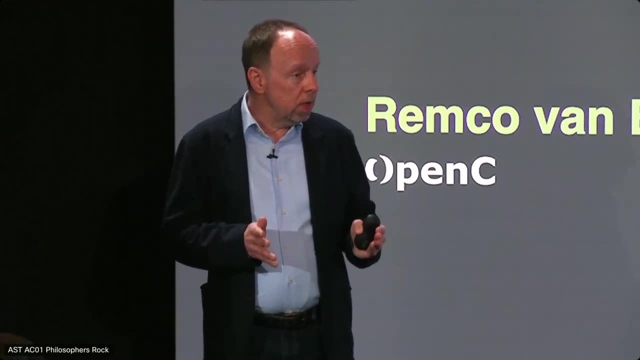 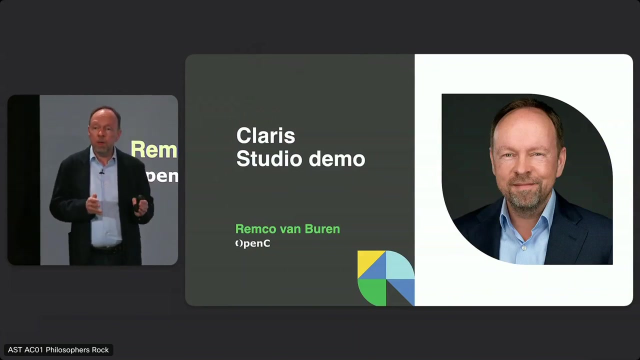 And they have been developing software on the FileMaker platform. that is an insurance system. So- and that's what we did two years ago- We migrated our old real access software to FileMaker. So I'm really a FileMaker guy, But I'm also very enthusiastic about Studio. 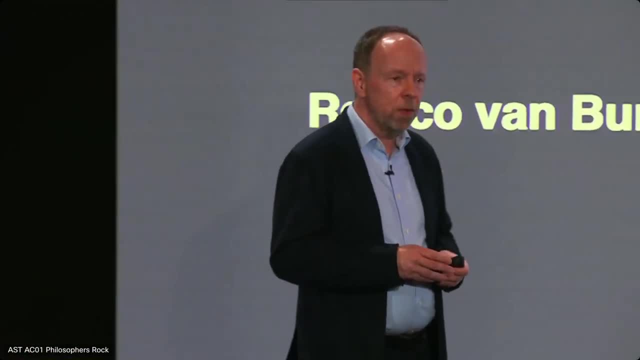 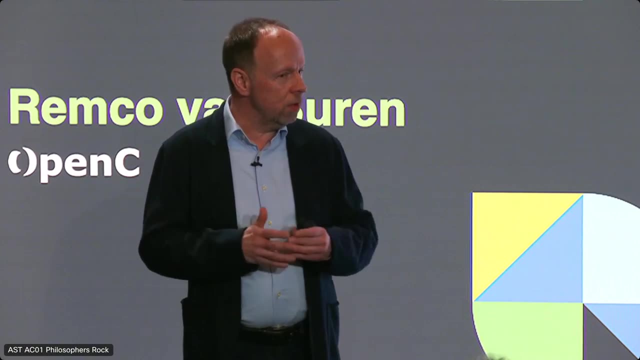 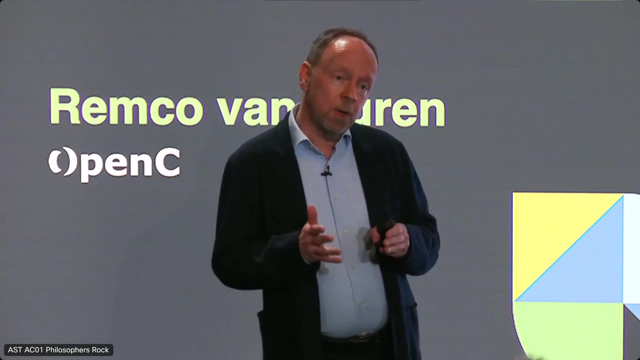 And that's what we're talking about today. So we're a small network company in the Netherlands And our vision is really to make insurance products, insurance processes, insurance solutions far more simple than they are today And, I have to add to that, far more simple for the people who know about insurance. 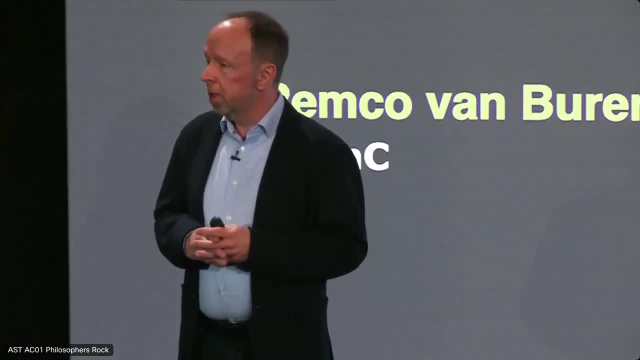 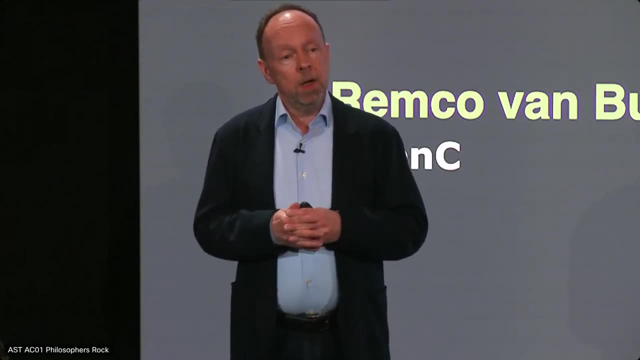 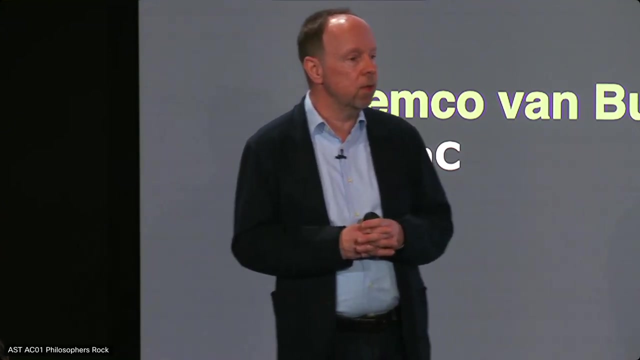 That's important to add to that. Now, our clients are very. most of them are very small companies. We ourself are also a very small company that are highly specialized in typical niche markets, And some of them have access to the largest insurance markets of the world. 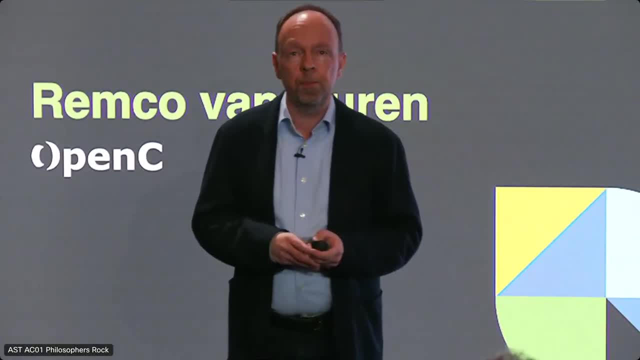 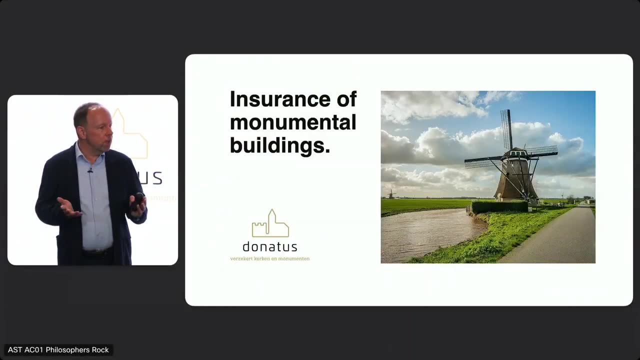 I'll talk about that about a little bit later. So first client, just to give you a few examples of clients. it's important to get some context, And then we'll kick off in the demo of Studio, of course, which is the core of my part. 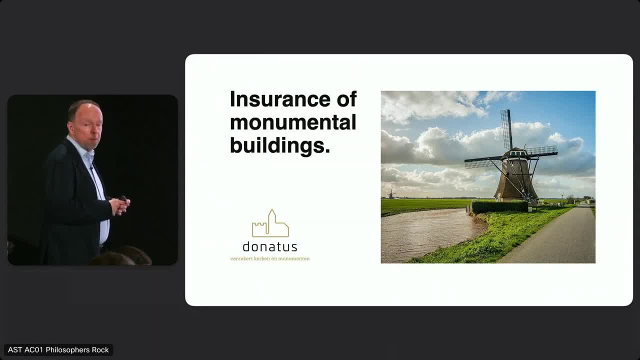 Of the presentation. Donatus, it's a Dutch insurance company, only insures monumental buildings. Most of them are hundreds of years old And they have to be insured because the people who own them are really very keen on preserving that heritage for the future generations. 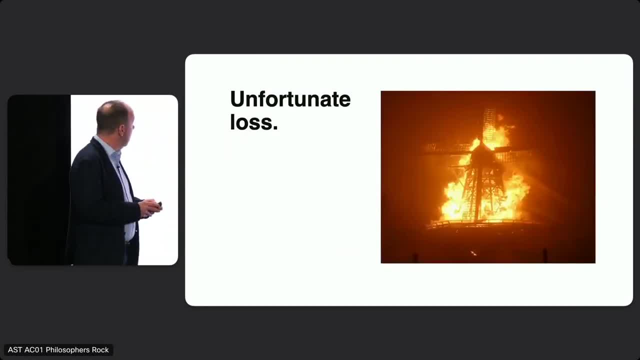 So that's very important to that. But sometimes something like this happens and then you know that insurance is a very important provision. This mill was, by the way, a successful one way rebuilt, so that's a rare case of rebuilding a mill. most of the time they 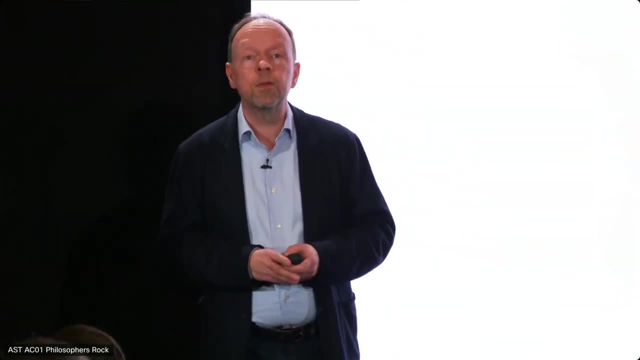 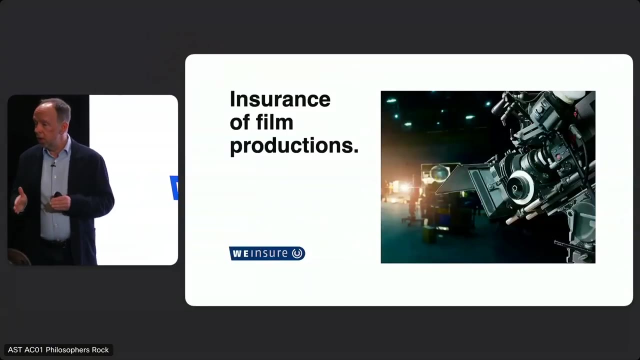 get completely lost when there is some fireworks entering it from the outside. another client, very interesting client we ensure. it's not the we ensure group that we know here in the United States of America, it's a Dutch we ensure group and they ensure films, film productions, and they have some clients I can't 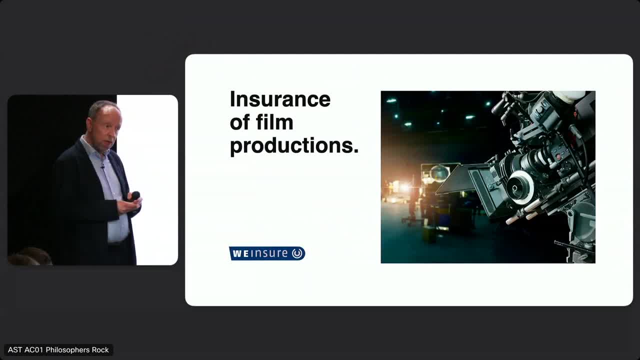 mention them by name, but I'm sure everybody in this room, if I would name a few of them, would absolutely know what I'm talking about, who those clients are. they make feature films, but also smaller production companies and they're a very interesting client for us and they are the first one who have adopted our new 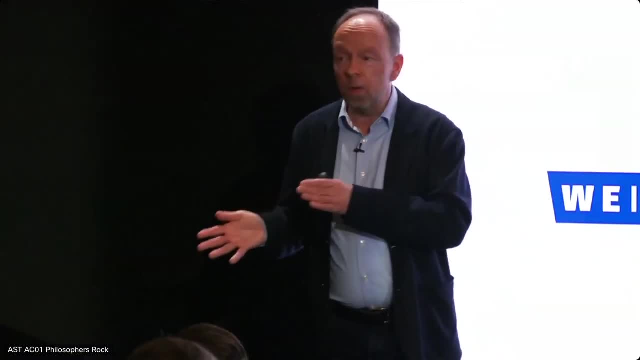 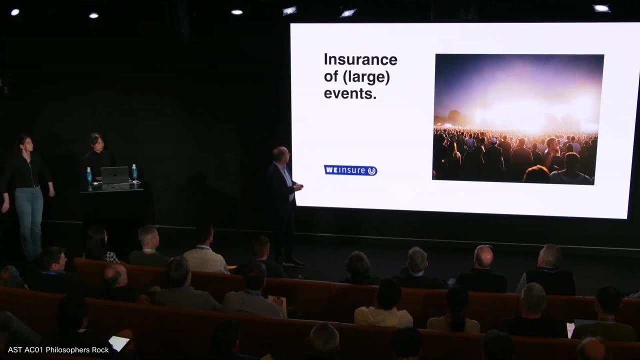 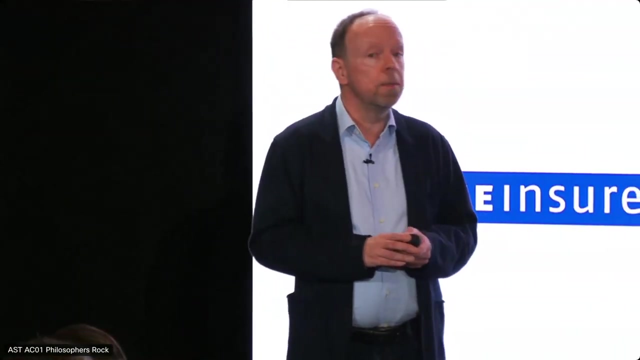 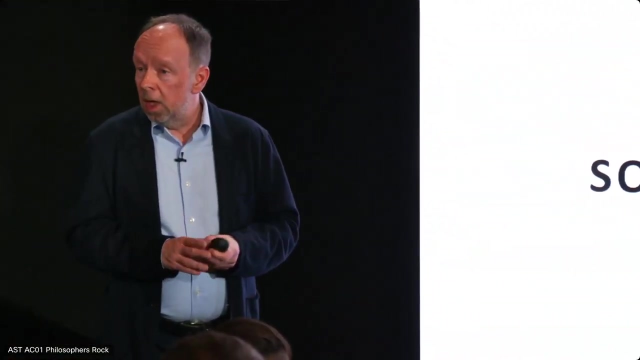 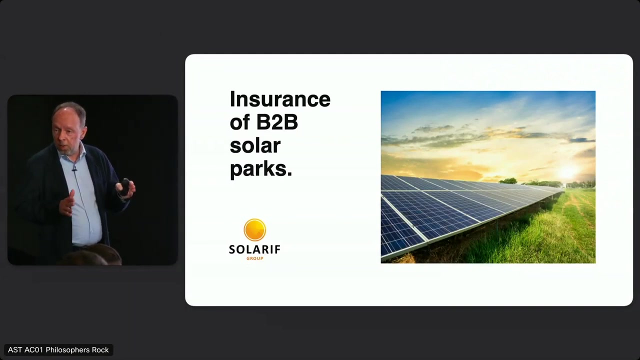 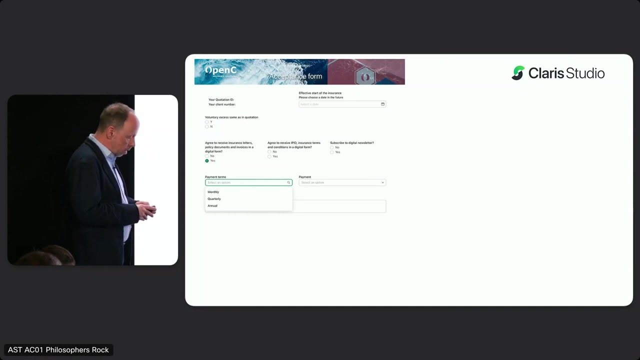 real access insurance system that we have migrated from our old platform to the FileMaker platform. so again, I'm a FileMaker guy. they also do you insurance of it and also the inspection and the certification of those platforms. so then Bridget reached out, and a few of their colleagues and said: why don't you? 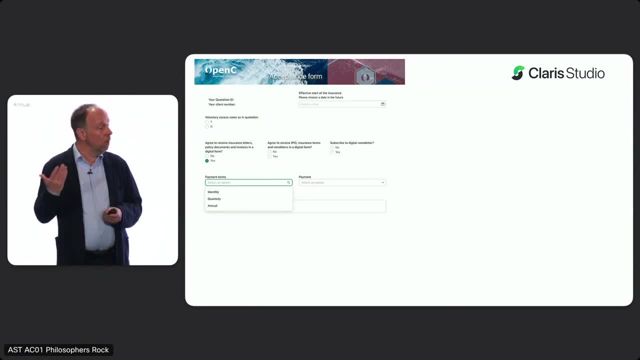 try CleverStudio, because we became a clever partner only last year, so we're kind of a new kid on the block and I said immediately: yes, that's, that's good, let's try it out. because I was following it from a fair distance for the last couple of years. from day one the studio was announced and now I 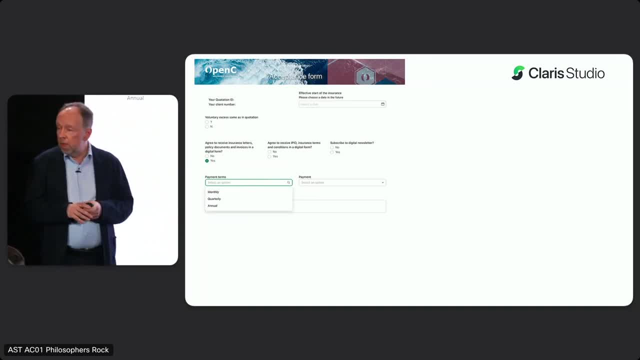 could get my hands on it and immediately it was clear for us that we were working it. literally within an hour, we were developing things and we- that's me, my marketing colleague and my sales manager- so I called them and I said, well, this is great stuff, we have to use this. and since then we have developed an 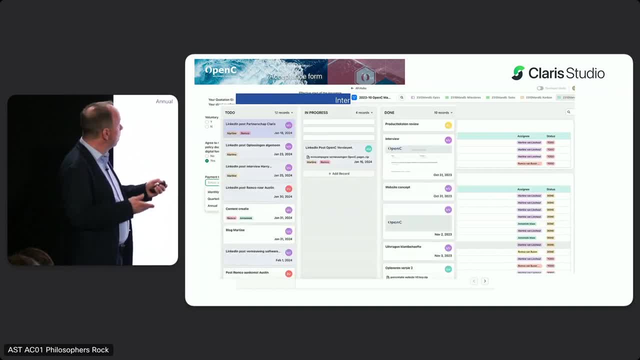 In a few days- all kinds of internal processes, applications, so to speak, to support our internal processes for OpenSea. to get a feel about it: Developing forms- insurance is about forms, of course, and also our marketing efforts, our LinkedIn posts, our sales and lead and prospect generation. 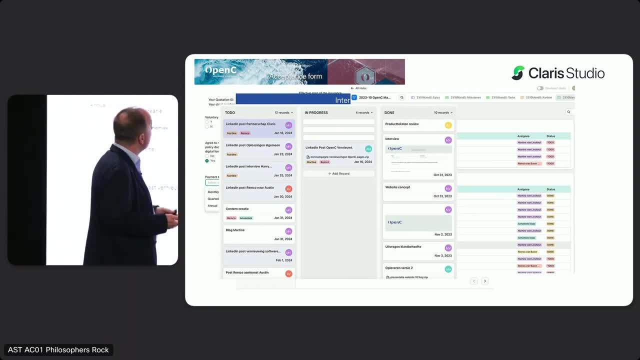 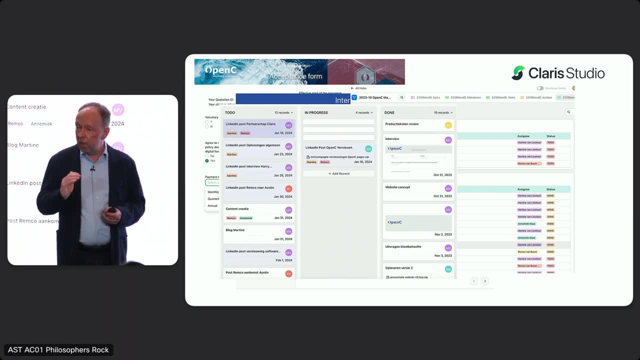 and our task management for all kinds of things. And that was really a surprise to myself how easy and there is no threshold. You can immediately use it and make some applications and get on with it. And then we told that we did. 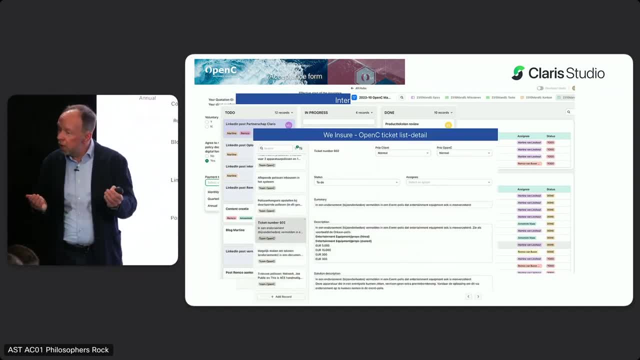 And we also made, by the way, a ticket system for one of our clients. So we tried to involve some of our clients immediately in this nuclear studio And we succeeded in that, So they could get their tickets issued to us And their wishes. 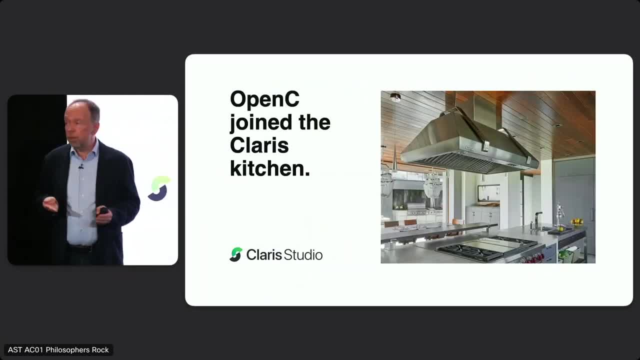 And then we told about this to Claris And then a couple of things happened. We were invited to the Claris kitchen, So then we got access to newer functionalities, And one of them is very important. It's the custom view in Claris Studio. 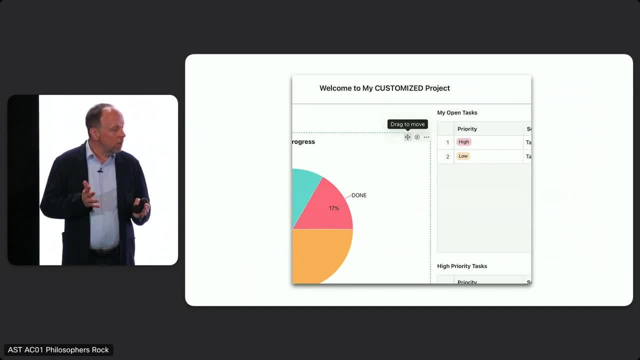 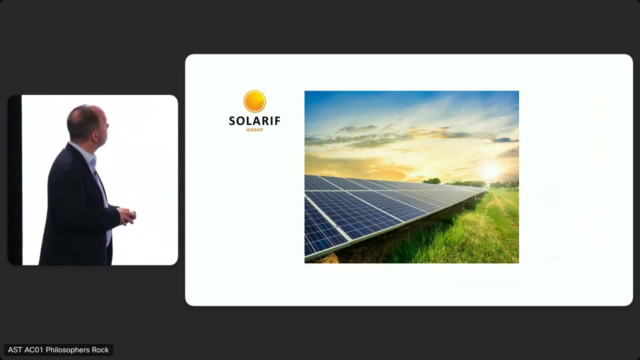 And that gives you a lot of freedom And, at the same time, to start with, it's fairly easy, So there's no threshold there And you can make wonderful stuff with it. So we continued on our journey to using Studio. And then Harry Wolkenfeld: he's the CEO of Solarif Group. 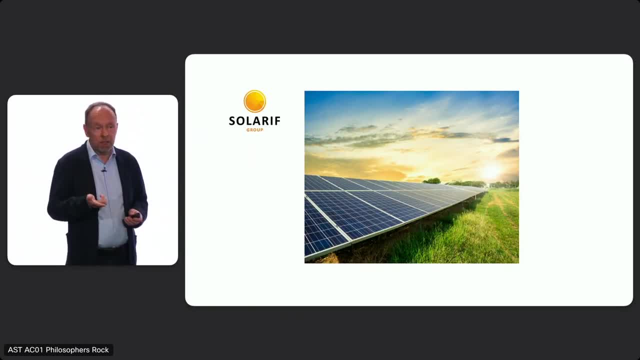 And the surname is very interesting because Wolkenfeld, if you translate that it's something like Cloudfield And he's in Solar. So that's kind of funny, I always think. And he called me and he said: Remco, could you with OpenSea and that Studio thing. 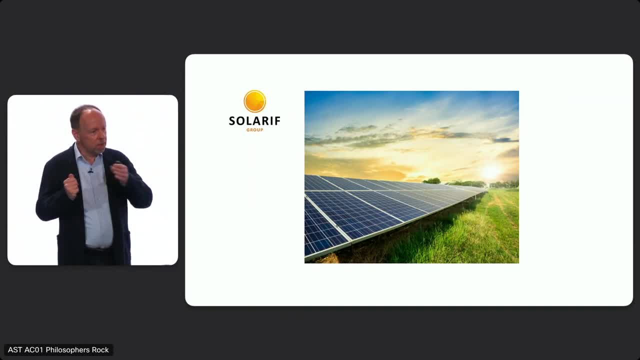 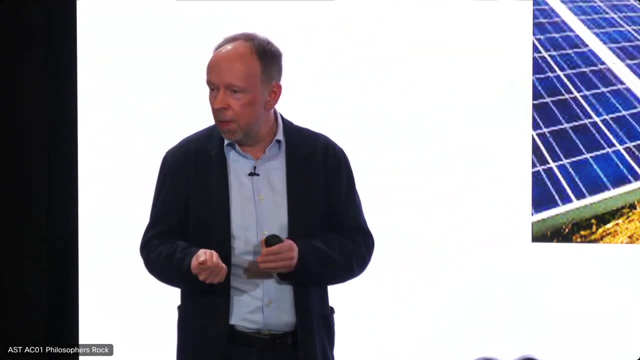 he said literally: can you make a business process, can you support that, Can you automate that with Studio and perhaps also with FileMaker? And two days later we had a proof of concept with the forms in place And we made use of our already existing FileMaker database to generate dynamic documents. 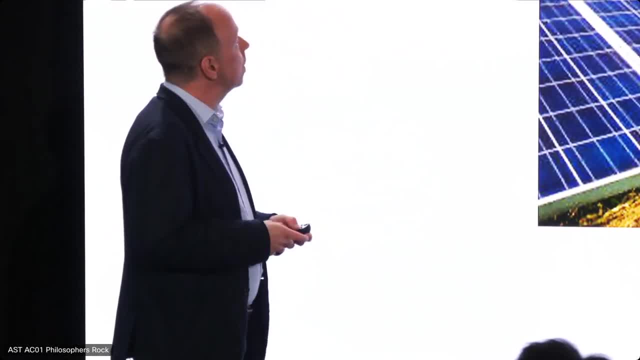 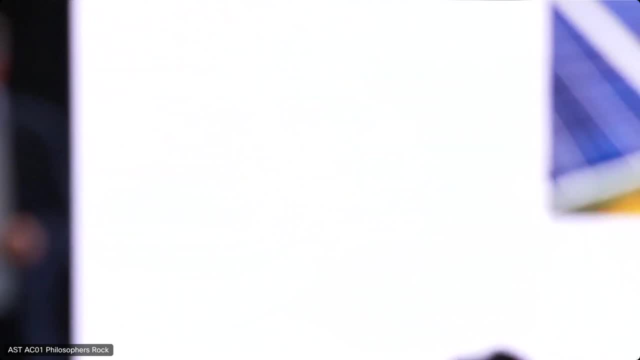 which you also use for the insurance policies and invoices, et cetera. So then they would say, well, go ahead with this project. So we acquired the project thanks to Studio, And then we were in need of a project management dashboard. 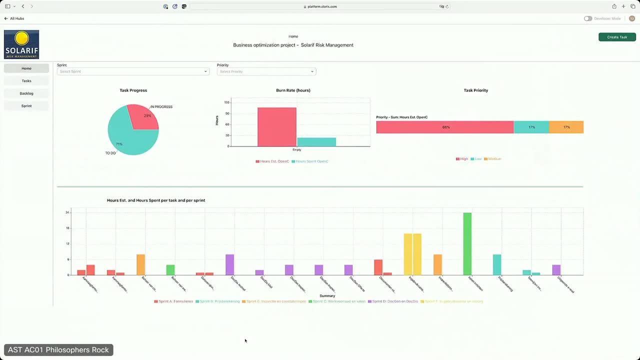 And that's what we have built in Studio, Just to test for ourselves. can we do project management in Studio And how do we do that? And can we develop something that's easy in Studio based upon the preview templates that Studio provides to you? 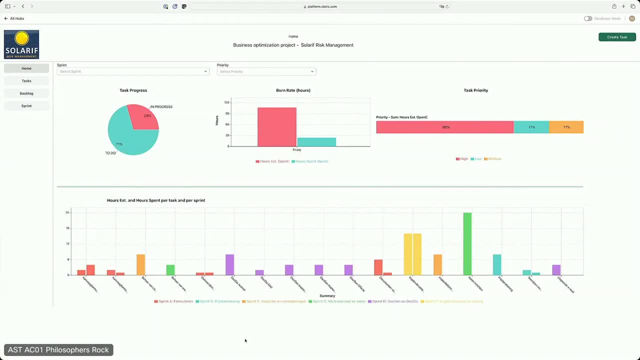 And then so we did. So this is what I developed myself, And if I press a button, the mouse is going to move And on the left-hand side you see, with the pie chart, the tasks that are in progress or to do. 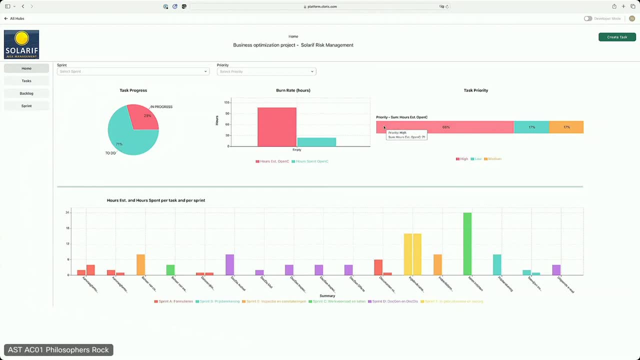 There's not yet any tasks done yet at this stage in the project. In the middle is the burn rate And on the right-hand side you see the priority, the division of tasks in priority. Most of them are high priority. The below bar chart is tasks hours estimate hours spent per task. 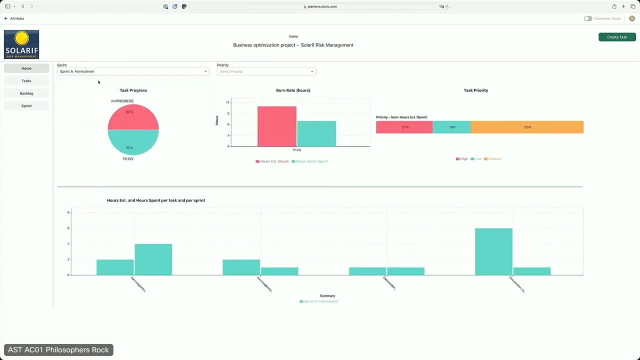 And the color represents the sprint the task is allocated to. So that's what we have developed, And then the hard part was to develop those two filters that are dependent on each other. So you can see, I can choose the task from one sprint and only see the high priority tasks. 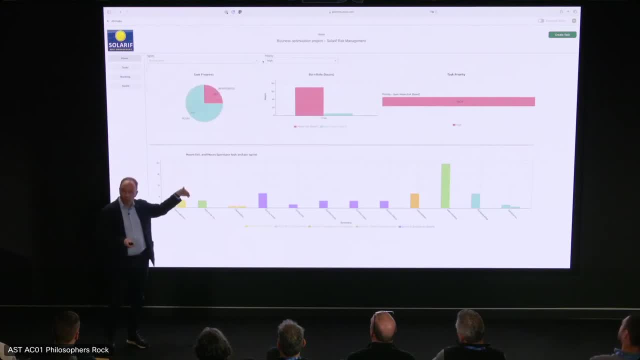 But then if I delete the sprint, I want to see all the high priority tasks, no matter in which sprint they are in. Once we figured that out, that worked very great. And of course the right-hand side shows 100% because I only have the high priority task here. 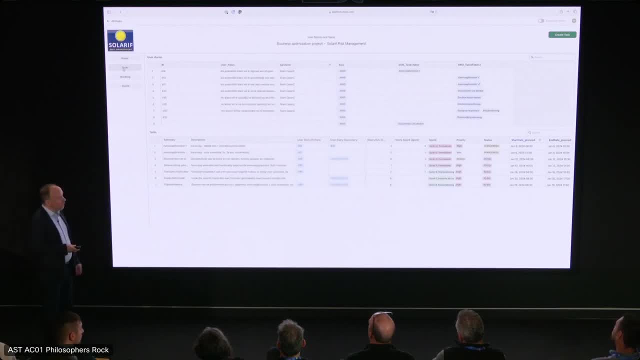 So I'm going to select this one Second case. in the same project dashboard, we came up with this. So, first of all, we developed a spreadsheet and a form to define user stories. As a client, I want to do this and that in order to do that and that, 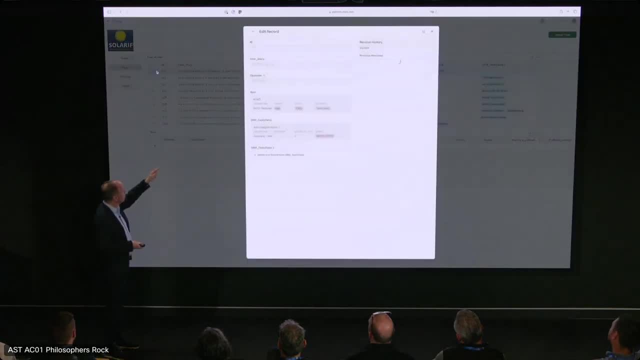 They're in the table. I can change the column width if I want to. I can see or edit the records very easily. And then I discovered something. I can also see the history, The track records, the tracking of the record editing. 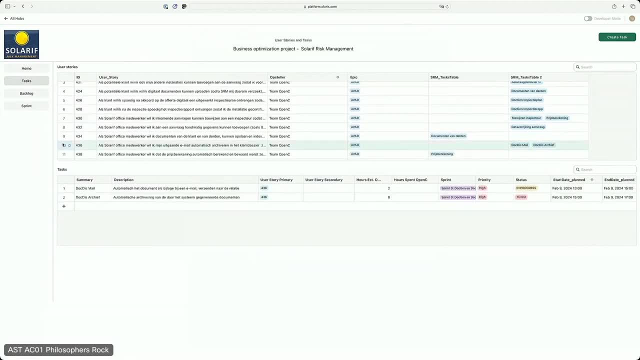 And then if I click on one task, it filters down only the task. I'm sorry, user story- Only the tasks that are part of this user story. So then I can focus And then you can see it. 436 is here. 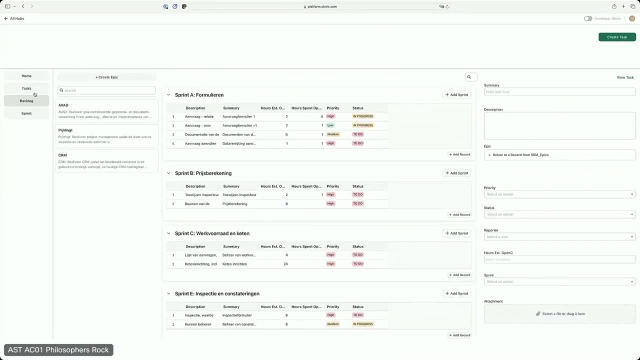 The key for 436, the user story, primary Third, the backlog, Three epics, several sprints, And if I click one task within a sprint on the right-hand side, I can see my details. And this is all a matter of just hours working on it. 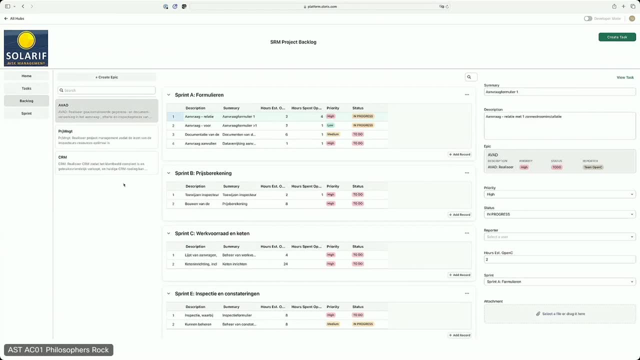 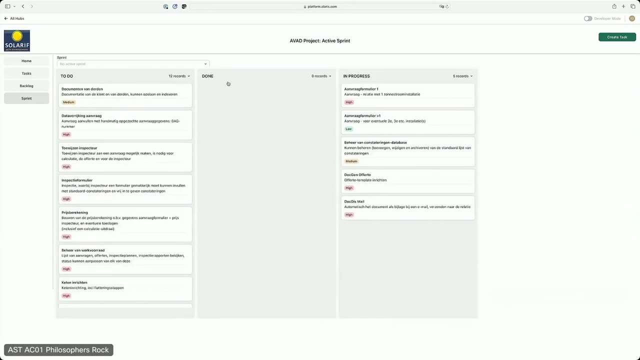 And then you have your project management dashboard And then the sprints We have to do, done and in progress. Might not be the order that you would expect, But for us it's very good the way it works like this. And also you have your details on the right-hand side. 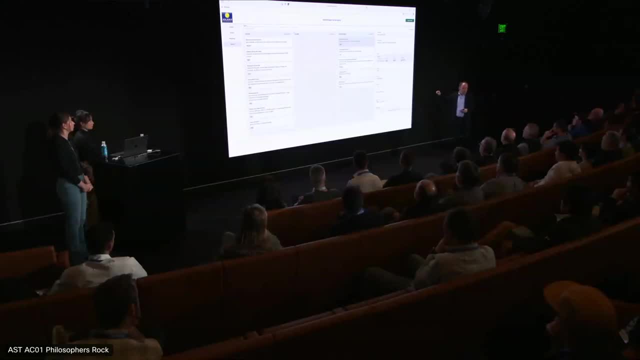 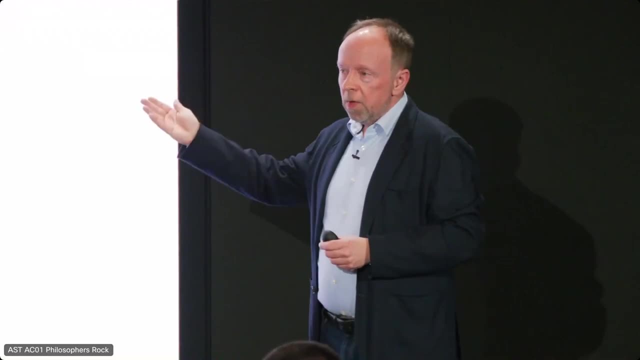 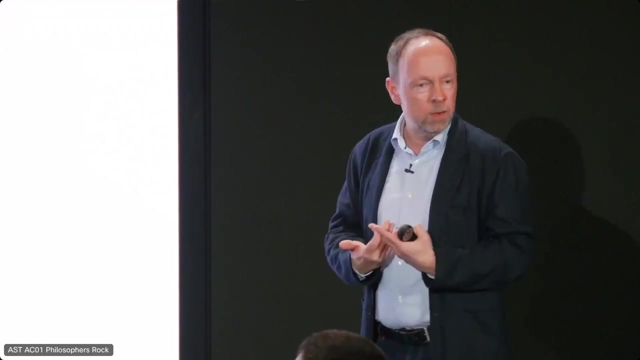 So this is the project management dashboard of the particular project for the inspection process of solar panel, large solar panel platforms And SolarRef. our client can also view this project, So we can together manage that project, which is lovely, Because then you have an extra interaction with your client in the project itself. 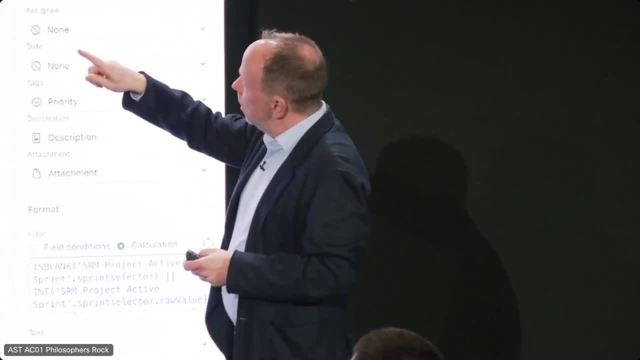 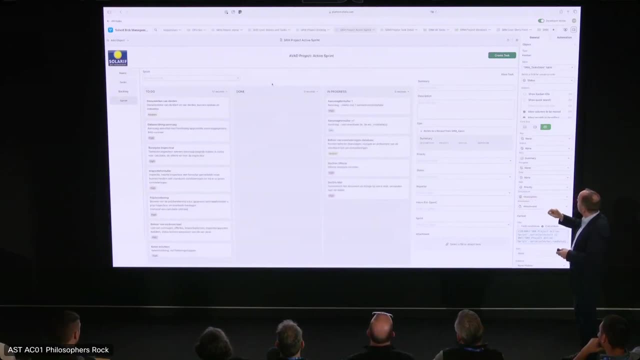 Then I saw a small error, which I'm improving right now. So while I was making this video and then you can see the power of the custom view, Because the sprint button was behind the to-do button And I've just fixed that. 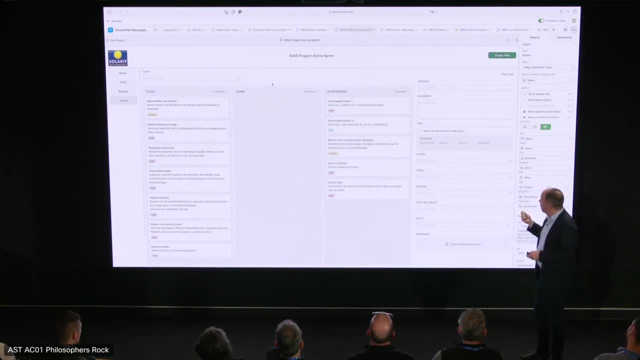 So now I've come to realize that I can do two things at the same time. I didn't know that in my life, but now I do, Thanks to Studio, Thanks to the custom view. So that gives you an impression of what we have done up until so far. 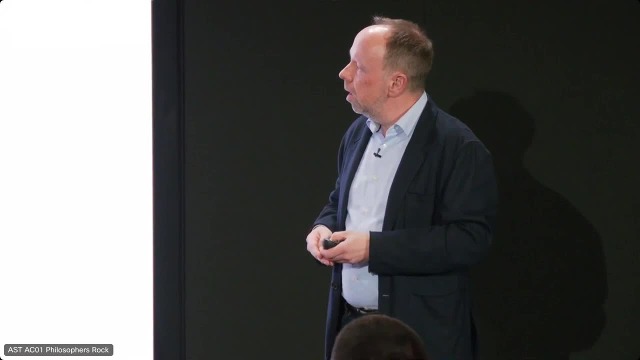 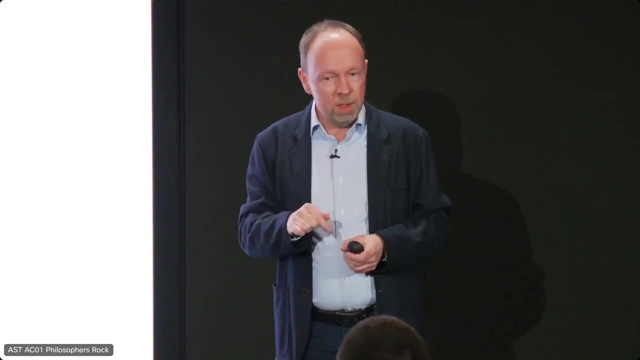 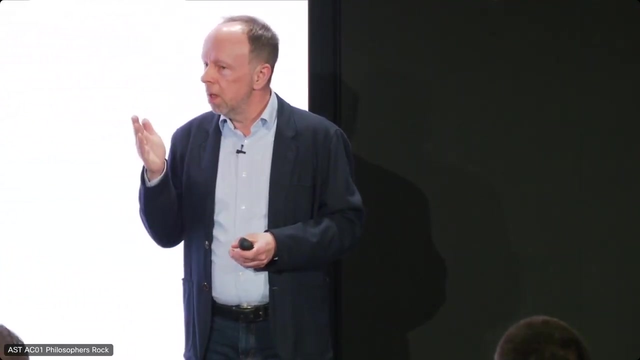 So, to conclude, I'm very sure that every one of you here has one or two clients at this moment, And I say that humble and in a modest way, But I'm dead sure that everybody in this audience has one or two clients that are in need of Studio right now. 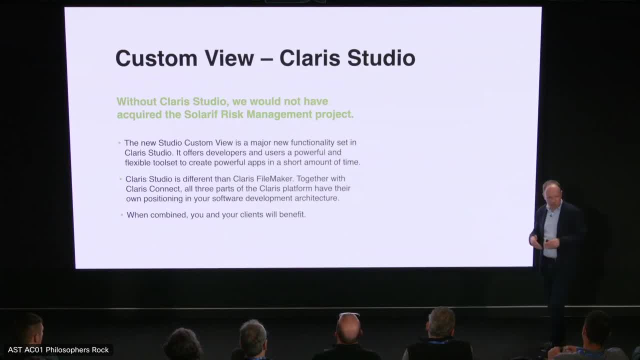 It has to be, Because it's so easy to use, not only for yourself, but for your clients. So please try this out. And for us, it meant that we acquired a new project that we didn't have acquired previously. So we are very committed to go on with Studio, also with FileMaker and also with Claris Connect. 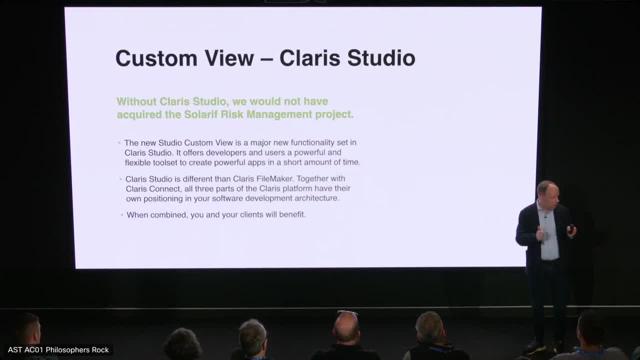 Because they're parts, in our view, of the same architecture And you just have to find the right spot of each application, of each platform In your architecture for the client. So this project will definitely include Claris FileMaker, but it also will include Studio. 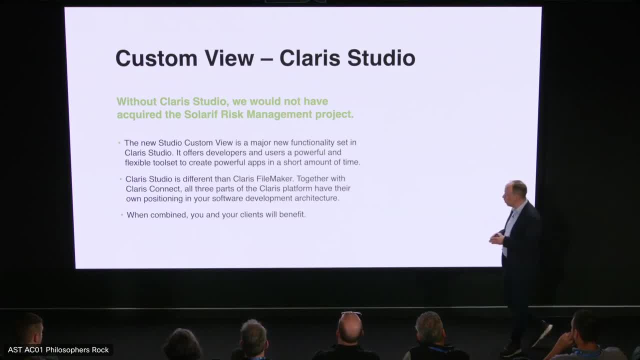 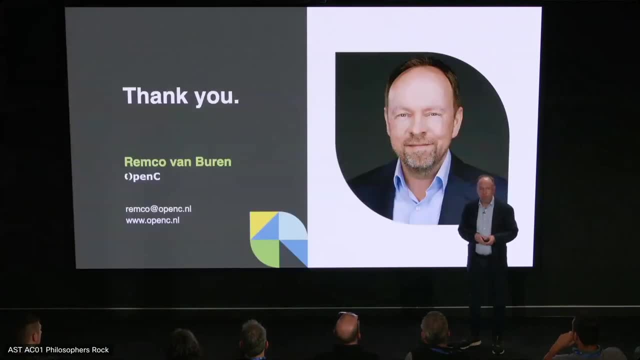 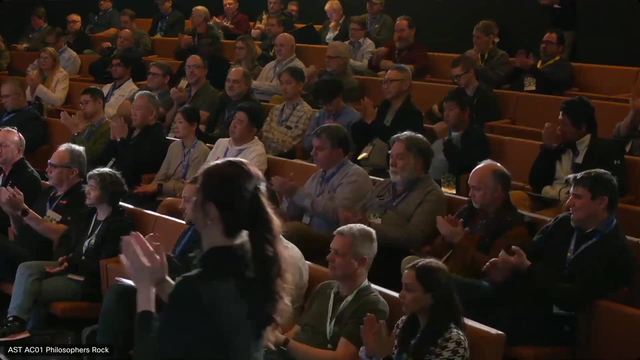 Both of them And Claris Connect, by the way, So all three of them. So I'm convinced that when combined, you and your clients will benefit. So thank you very much And stay awesome. Thank you so much, Remco. 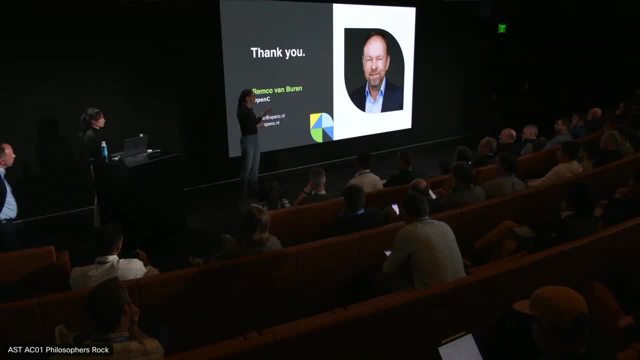 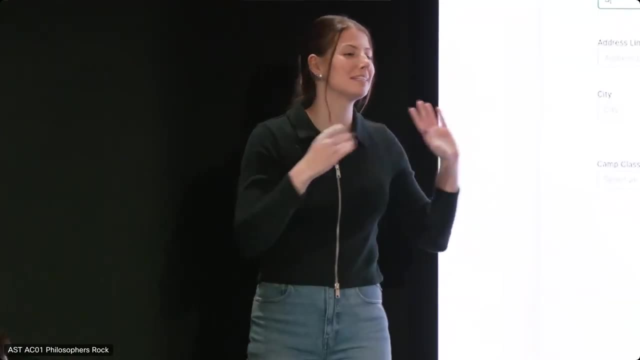 As you can see, Studio has come a long way since its form days. Now, before we jump into some demos, I'm going to take us back to the beginning. real quick Again to set the stage. I know I'm sorry. 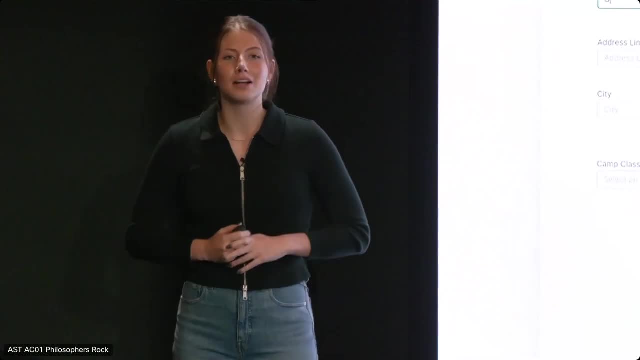 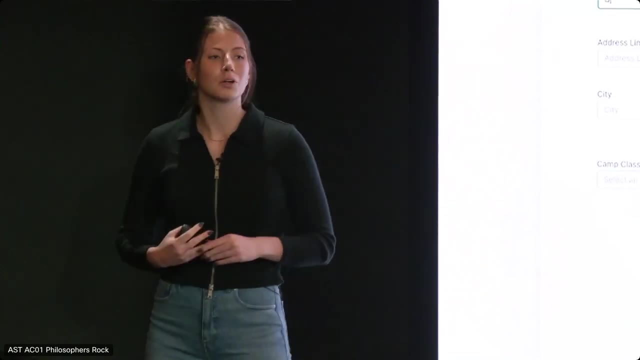 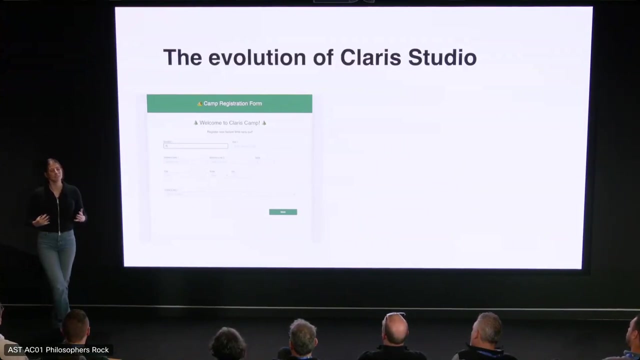 You're here for the demos. But when we started building Claris Studio, we wanted to anchor our development around use cases, To make sure that we're delivering U-value While also providing The right building blocks. And when we first launched Studio, we missed an opportunity to tell us a beautiful story. 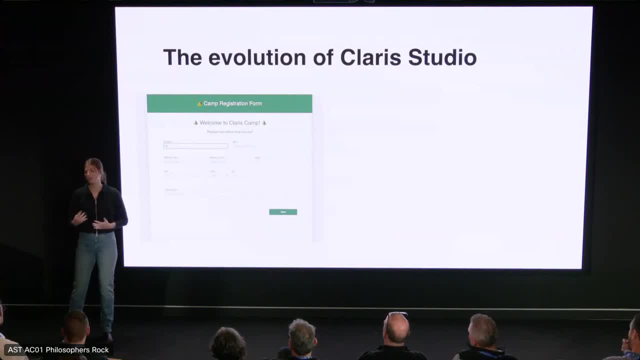 Of how Studio was growing together with the platform Connect and FileMaker. There was confusion that Studio was replacing FileMaker And therefore should have FileMaker equivalent functionality. But let me now tell you the beautiful story of how Studio came to be where it is today. 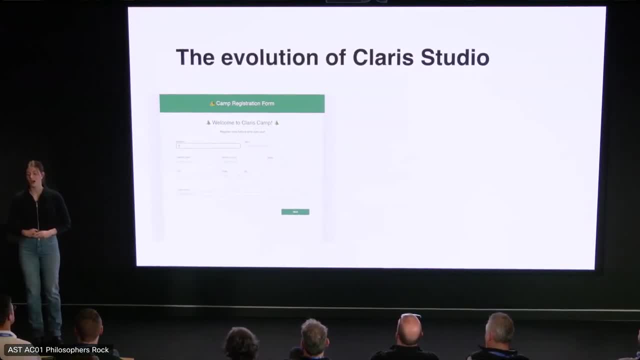 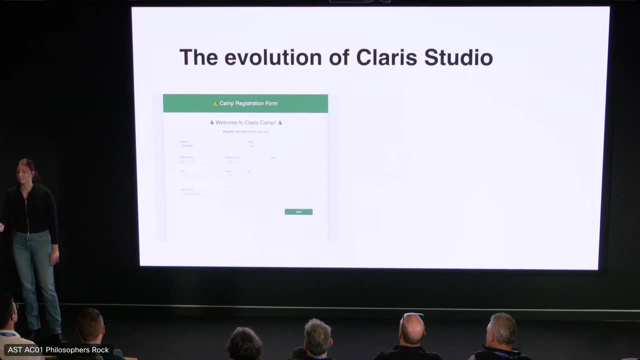 So our first use case, As I mentioned in the keynote, was anonymous data collection. We know that with FileMaker and its current licensing, data collection is difficult to do in FileMaker And we thought this was a great use case to start with. 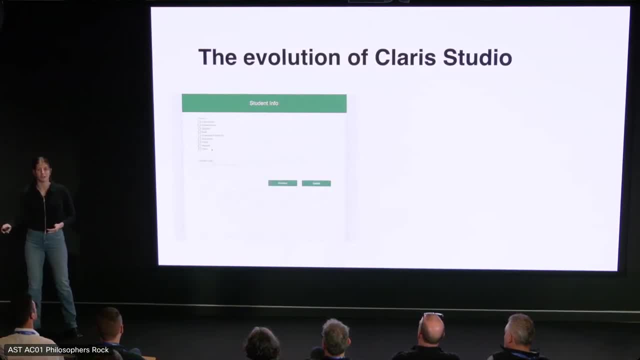 So that, behind the scenes, we could build our entirely new tech stack. From there, the natural next steps was to have a spreadsheet view So you can manipulate your data and view it And from there port it over to FileMaker to actually be able to look at it. 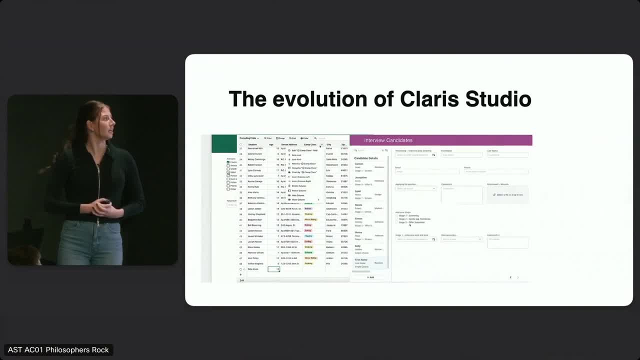 And from there port it over to FileMaker to actually be able to look at it And from there port it over to FileMaker to actually be able to leverage your data. The next use case, Our next use case that we selected, was project management. 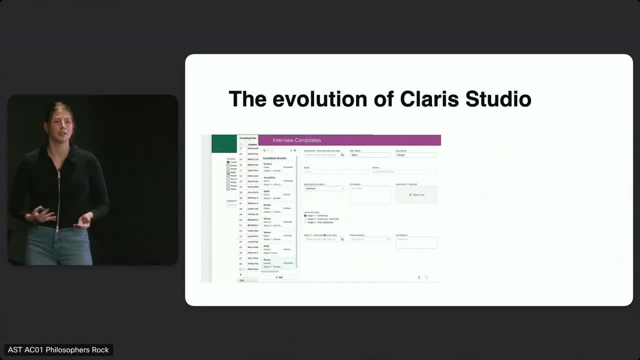 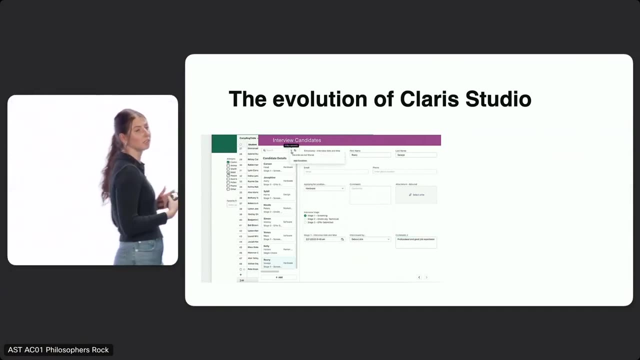 We know that project management is a very complex use case That can vary very widely from company to company. We validated with our partners their pain in sharing their project statuses with their clients And we also wanted to prove internally. And we also wanted to prove internally. 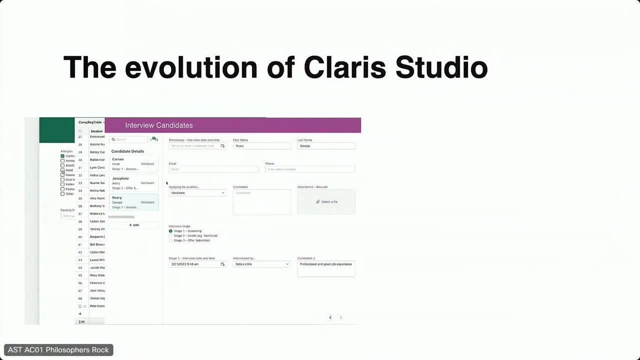 And we also wanted to prove internally To ourselves that we could use Studio And we had pain with project management. So this range is exactly why we chose project management as our next use case. The complexity and depth of the use case allowed us to start building some really interesting building blocks that you saw in Remco's demo. 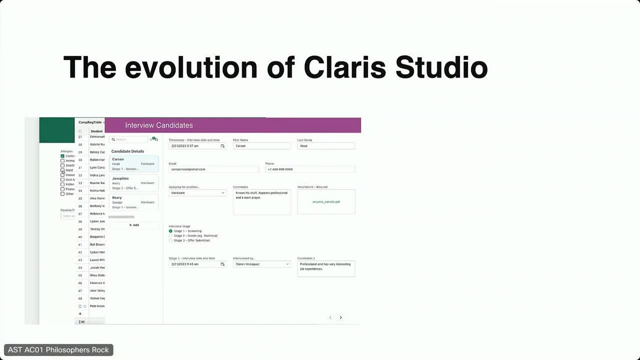 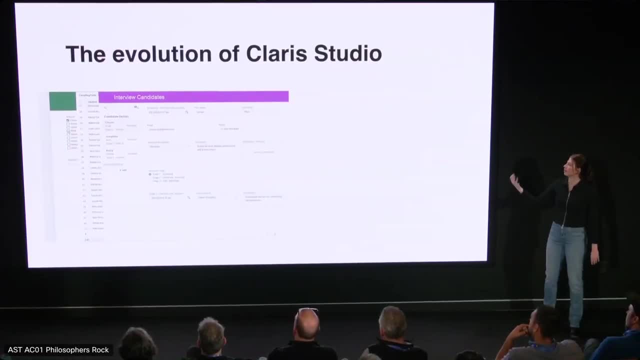 But we had a long way to go before we got there. So next came the list detail view And, as you can see, it has the list of records. Records on the right and on the left populates with the details of the record. 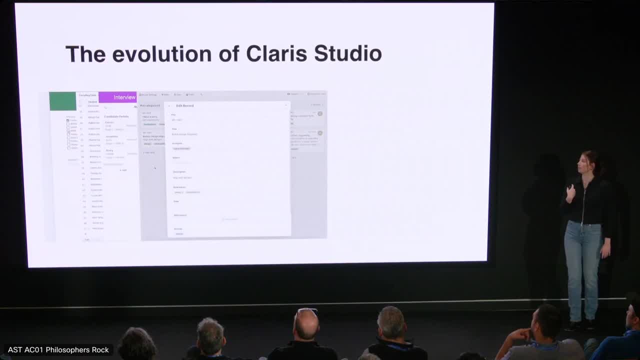 Then came Kanban view, which we use a lot and as Remco showed as well, to visualize the progress of your project. List view came as well to be able to view your data in grouped records. Timeline view came so you're able to visually see how your project. 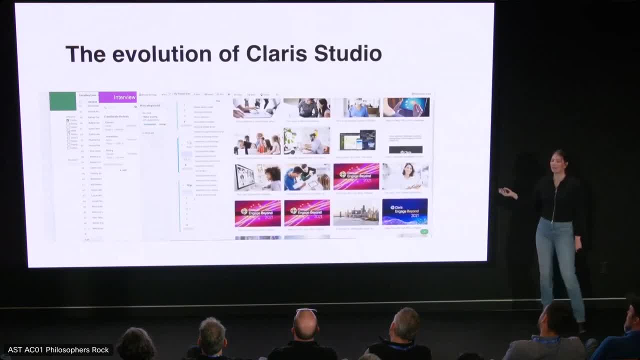 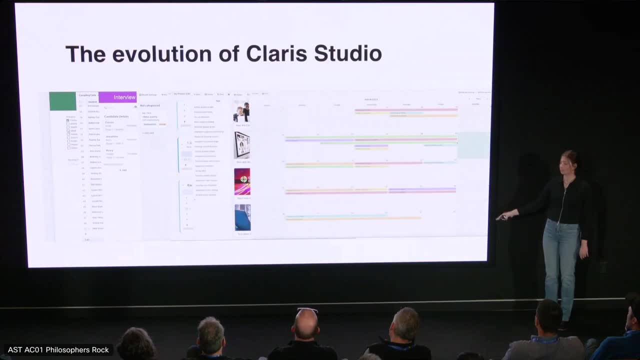 Project is tracking. Gallery view came to view photos and videos easily. And lastly, we had calendar view to be able to manipulate your data in a calendar setting. But all of these views were just stepping stones, And now, as you got a sneak peek of in both Remco's demo and in the keynote, 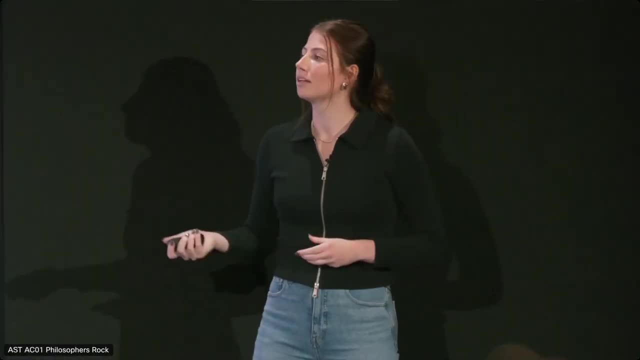 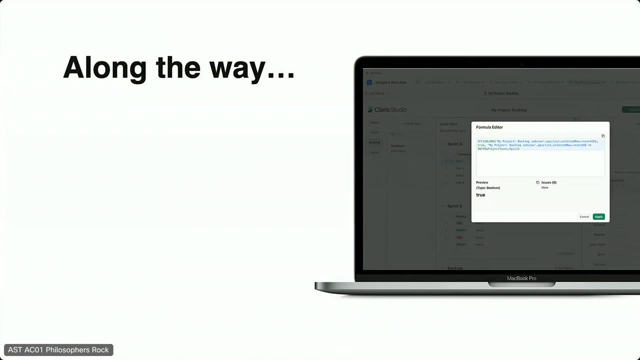 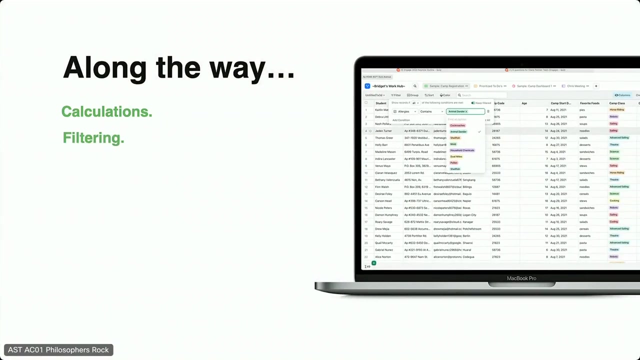 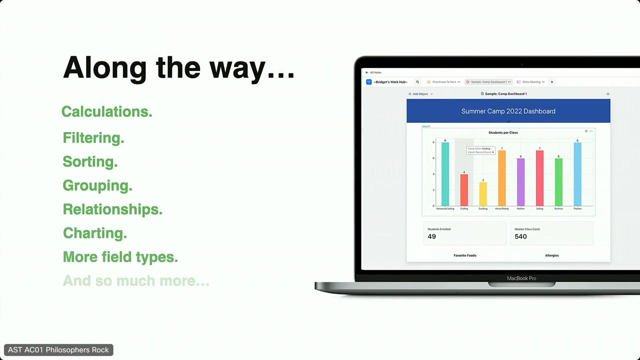 These are now all objects that can be dragged and dropped on to our custom view, But along the way we had to create a rich set of features and functionality as well, Including calculations, filtering, sorting, grouping, relationships, charting, a lot more field types and so much more. 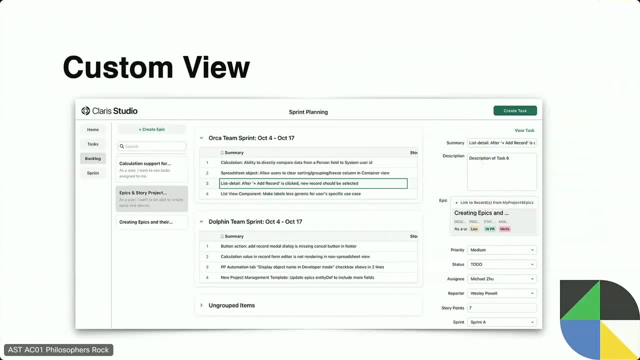 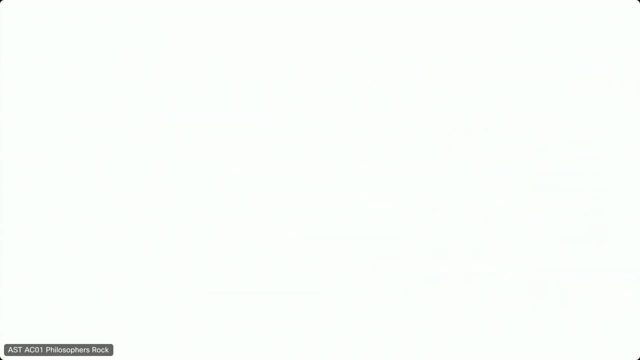 We don't have time to cover all of it today, And that led us to where we are today, which you saw in Remco's demo of custom view, And custom view is exactly what you think it is. It's a completely blank canvas for you all to build on. 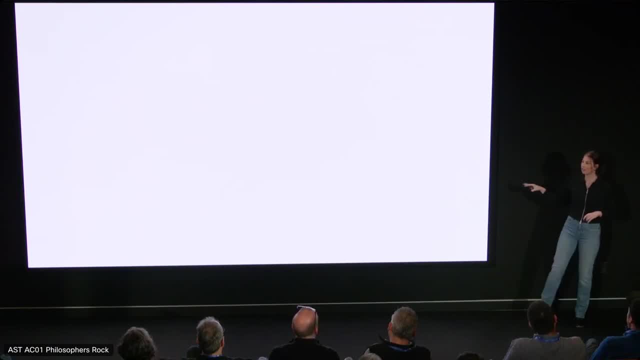 But, like I said before, the real magic is under the hood of how the developer can leverage this canvas. And to show you some of that magic, I'm going to hand it off to Angela Chen now to do some demos. Thank you, Bridget. 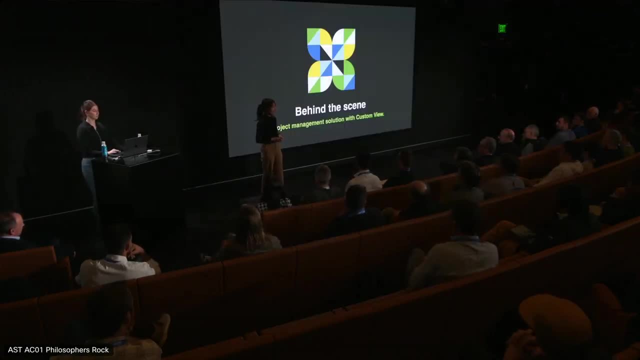 So hello everyone. My name is Angela Chen and I'm a front end software engineer here at Claris Studio, So I'm super excited to meet all of you here, and I can't wait to share with you some cool stuff that we're building. 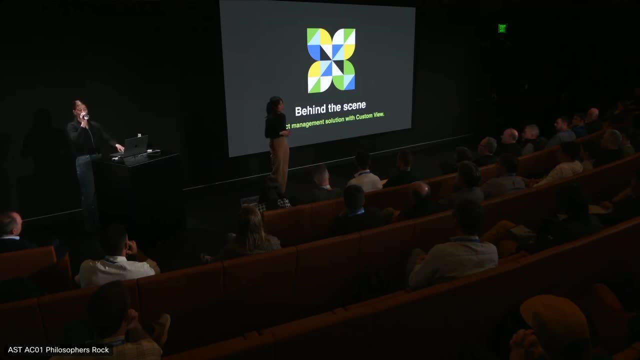 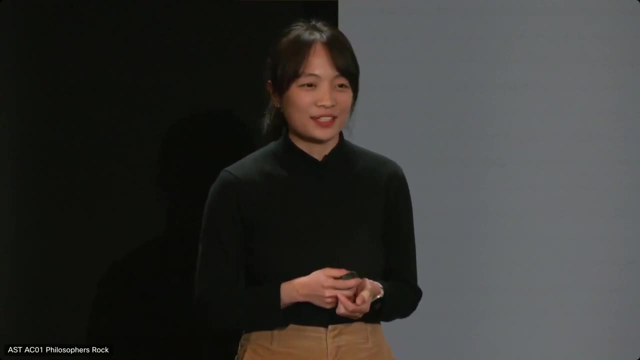 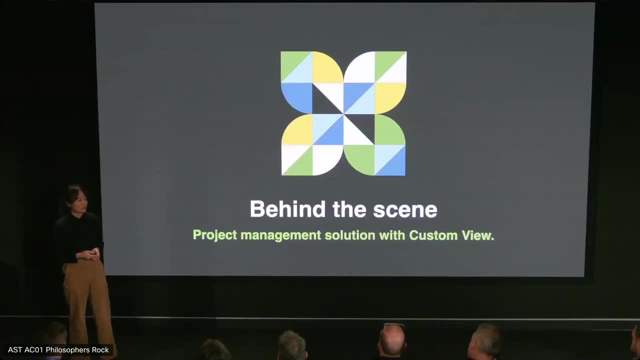 So, and I believe you're as excited as I am, So, and I believe you're as excited as I am, So, and I believe you're as excited as I am. So it's time for us to un-view some behind the scene magics. 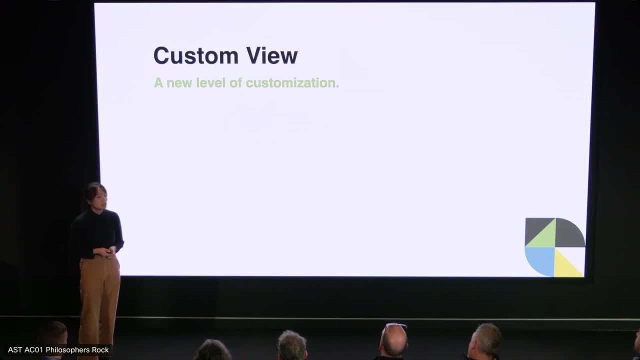 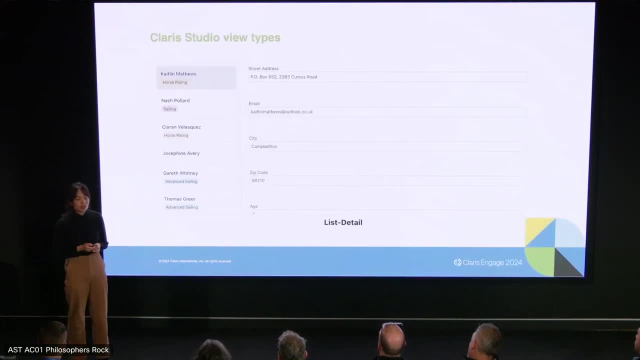 And first I'll do a big expansion on custom view. So why do we build custom view and what does it mean to have a new level of customization? So, through the early stage of Studio, one of the feedback we've got is that we 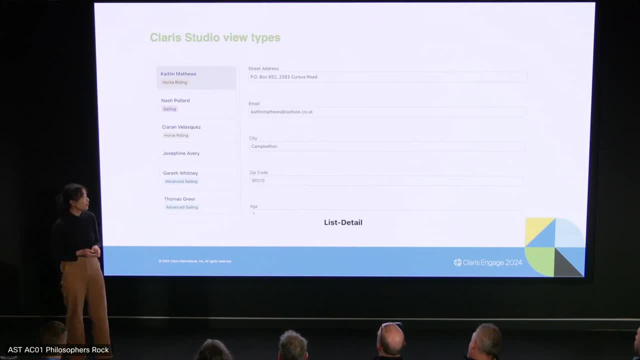 wanted more customization of the existing views. So for example here in list detail, we hope that the data list doesn't always have to be on the left And in the form we want to size and position things in a way that wasn't possible with the three-column grid system. 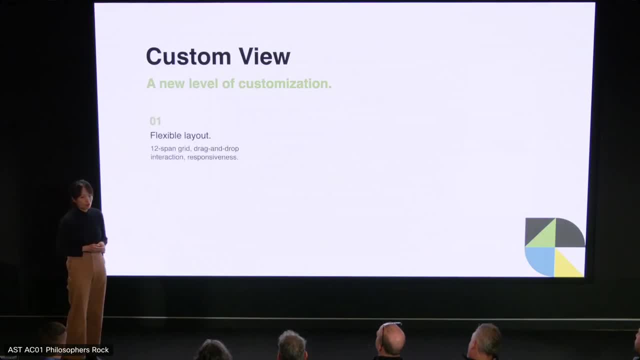 So with all that feedback, we started building a much more flexible layout. So the custom view today support a 12-span grid system, which gave you much more flexibility on how you want to design your own layout, And we also built a seamless drag and drop experience and 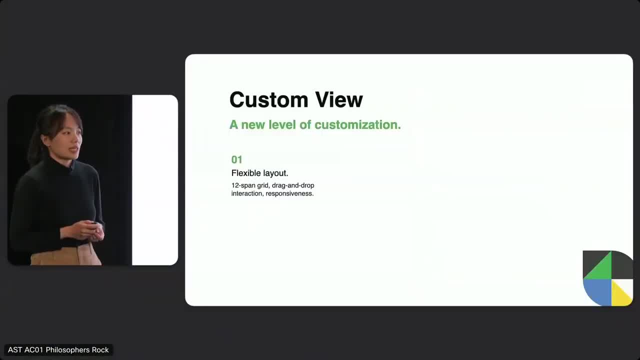 brought the responsiveness to a whole new level. So the expectation here is that Studio behaves as a modern web application, and we always want to stay true to that. So, after we solved the needs of customizing the layout, now the question becomes: what if we want to show multiple views? 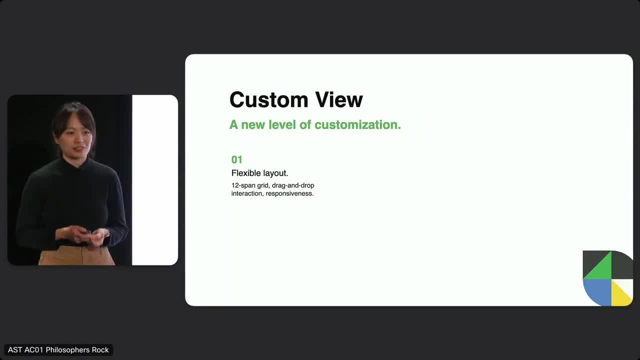 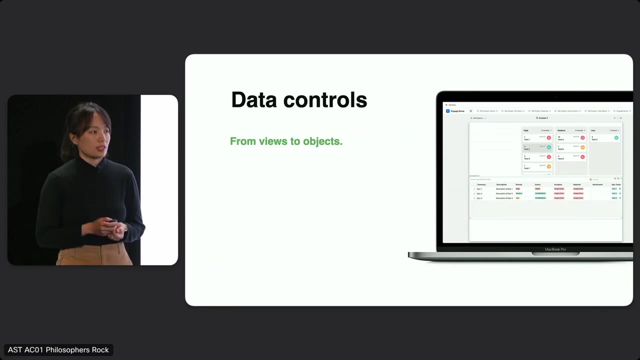 at the same screen or even make the views interact with each other. So the answer to that question is what we call data controls in Studio, as you might have already heard. So yeah, like you see, in Studio we converted all the in-market views into a set of objects in your custom view. 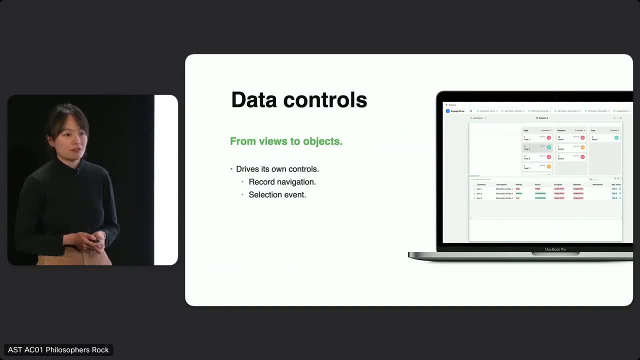 and we call them data controls. So the power of these data controls is in the control. So each data control will now manage its own record navigation and drives its own selection events that will eventually populate the other controls in your application. And, more importantly, a data control is 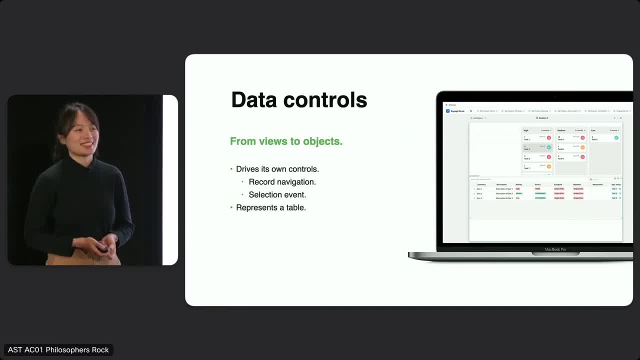 solved- is now bound with a table based on your choice. So, as we know, previously a view is always backed by a table in FileMaker or Studio, which is still true today, But now, on top of that, you can associate a table to your data control objects. 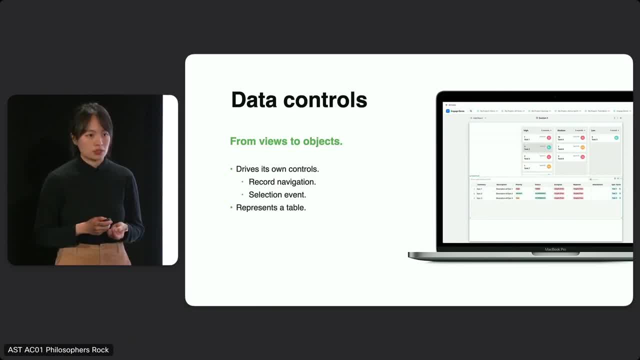 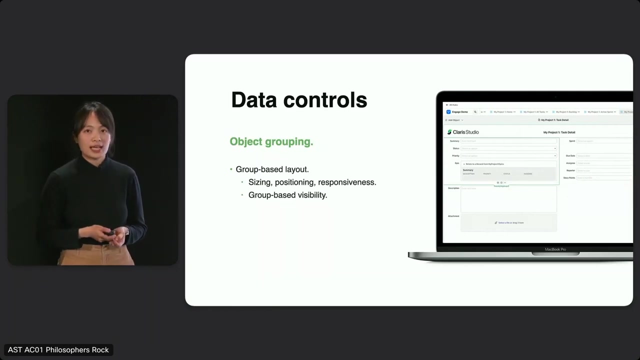 And with that flexibility you can have multiple tables represented at the same view. So the introduction of data control also means that there will be a lot more objects to manage. And to help you do that easily, we introduce object grouping, So object groups. like its name, it provides one more layer of objects. 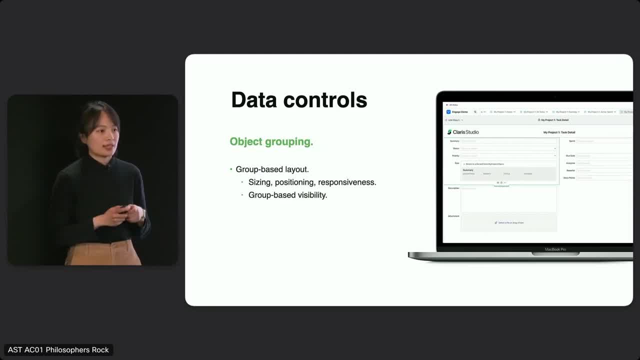 and allow a group-based layout. So you can now create a group of multiple objects, You can size or position the whole group together so that they don't get split up or staggered. Your group can even maintain its own responsiveness so that, for example, 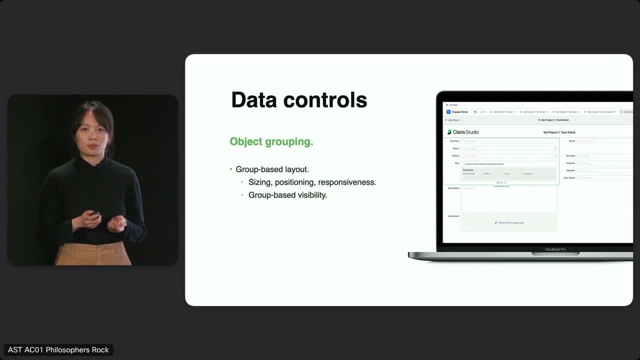 when your window resides, all the objects will stay within the same group, And there's also the ability to control the visibility by groups, which means that you can now show or hide the entire group based on the conditions you set, And beyond that. groups are extremely helpful in regards of the data hierarchy. 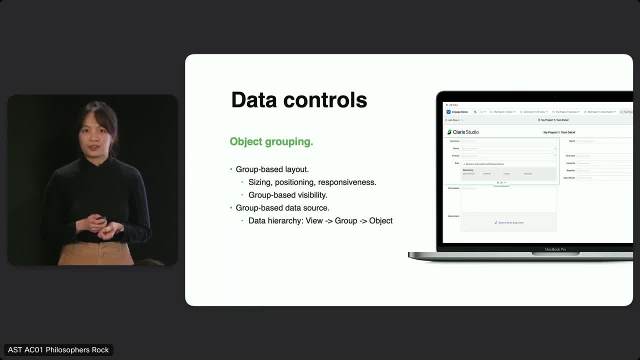 So if you are building a studio view, you can still configure the data source at the view level And, however, if you find yourself needing to overwrite or introduce multiple data sources, you can do that at the group level, And then individual objects will also have the ability to inherit or 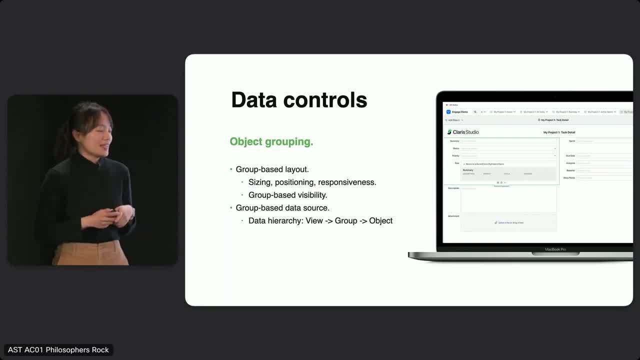 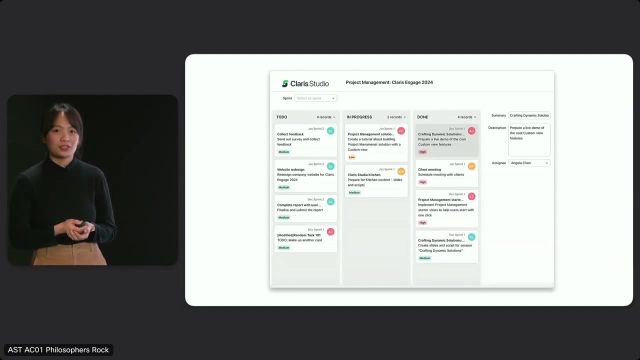 overwrite the group data source. So, yeah, we believe that data controls and object grouping will allow you to build a much more dynamic solution, as you need, with a smaller amount of time. So now it's time for us to go into studio and see some magic ourselves. So we were planning to do a live demo, but we figured that it might not be the time. So we were planning to do a live demo, but we figured that it might not be the time. So now it's time for us to go into studio and see some magic ourselves. 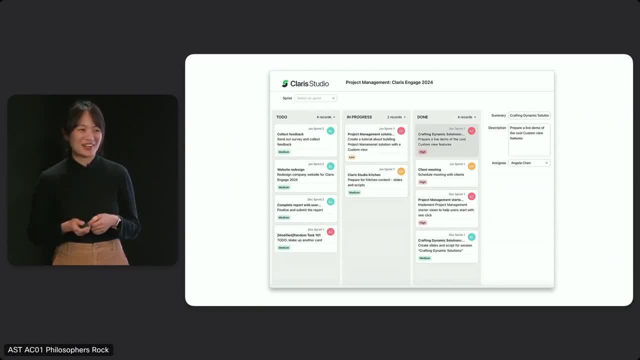 So we figured that it might not be the time, So we figured that it might not be the best idea with 600 people in the same building sharing the same Wi-Fi connection. So I made this: two demo videos of how we can build a solution like this in a few minutes. 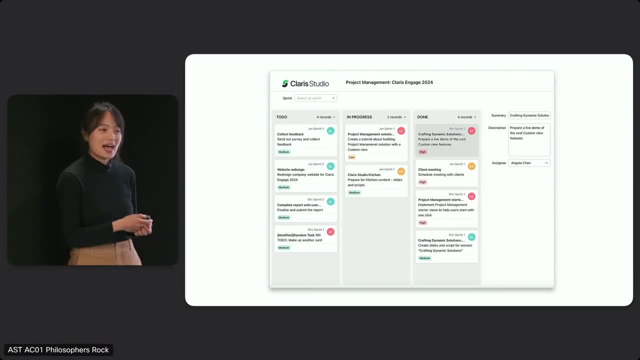 So this is what the end state will look like In this use case. I'm a Studio Product Team Member and I want to build a dynamic task command page for my team member to easily manage our tasks around the preparation of the engage this year. 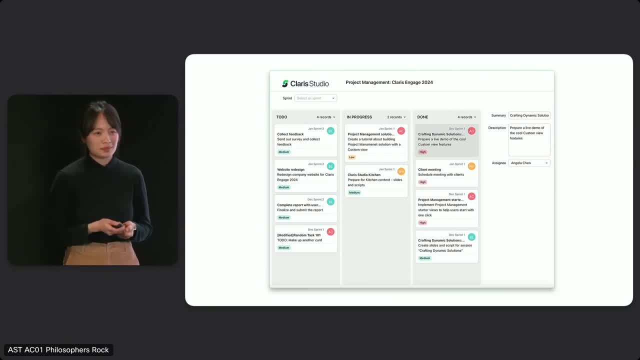 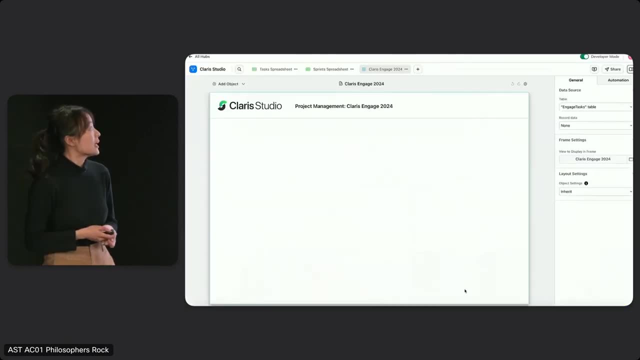 Which is the use case. I leave them brief in. you know, I have to make the changes and I also have to make the changes, and I also have to make the changes and I also have to make the changes, and in every day now. so, yeah, so we are now looking at a studio custom view I gave. 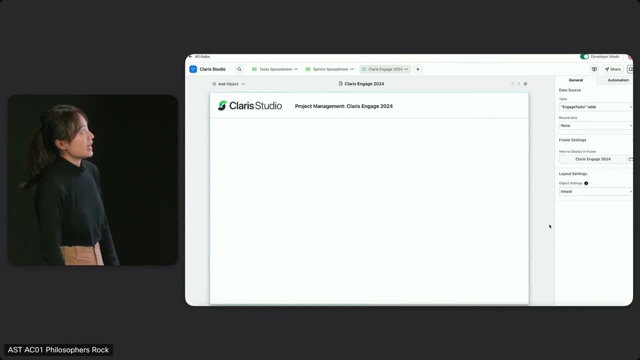 this view a name: Clarisse engage 2024. on the top, and before we start adding stuff into the view, let's look at what we call the properties pane on the right. so this is basically where all the magics happen, and now the properties pane is focusing. 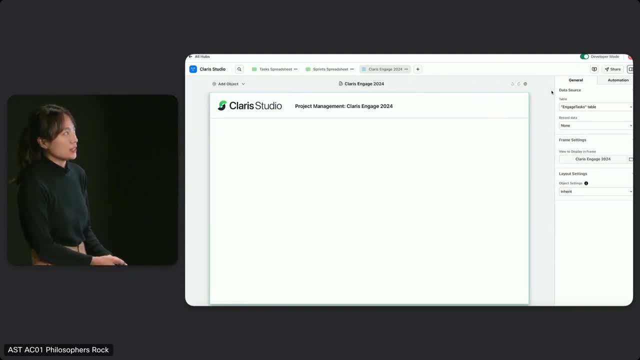 on the view itself and on top of it we saw a data source section. so from here you can actually assign a table and a record to the view, and this settings, as we mentioned, can be inherited and overrided by the groups or objects inside of you, and in this instance, our view is backed by a table called engaged. 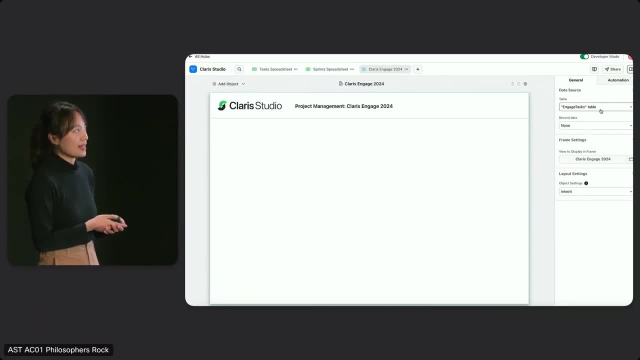 tasks. so I created this table before the demo and added some sample tasks, and the table has some tasks related fields, such as summary description, status assignee and so on. yeah, and by setting this as the views table, we started making assumptions for our app. um, next we will look at the top left side and open the add object menu. so 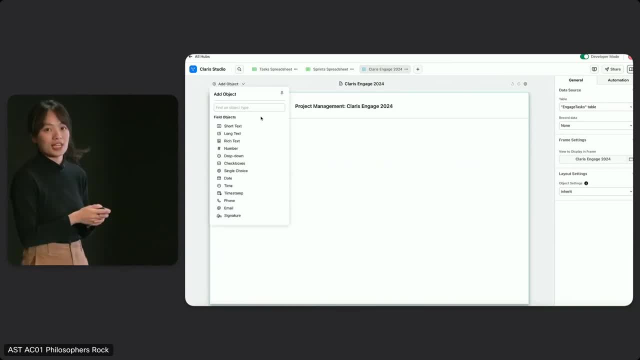 from here, on top of the list, we'll see the field object, which can be used as a representation of the fields in your table, and also you can simply use it as a UI element for your app, and when we scroll down, we will see summary objects, which provides various 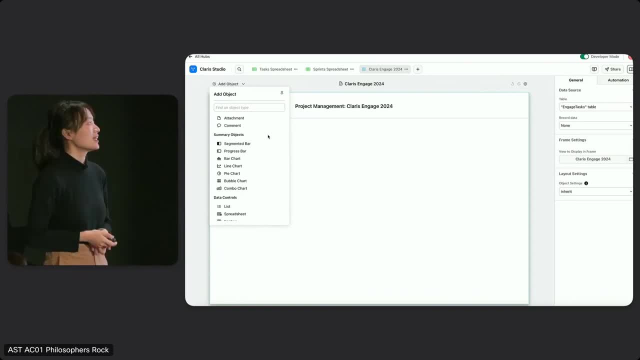 type of beautiful charts that you just saw from Ramco's demo- and if we continue scrolling, I'm here. data control are what we want to focus on first. so, as we mentioned, in the early evolution of studio, we worked really hard to implement a set of different views, such as list details, spreadsheet, Kanban list. 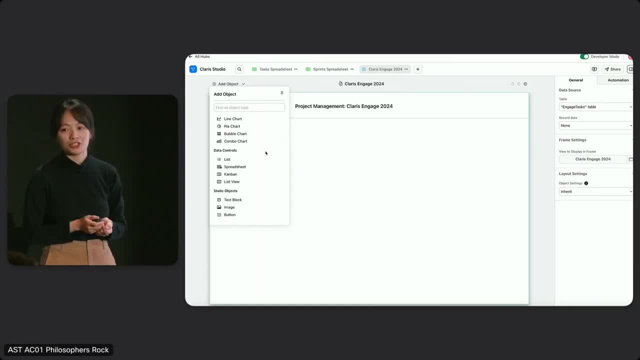 view and so on. so that's what we're going to focus on today, and we're going to focus on the data set, and we're going to talk about that later. but before we move on to the next step, we want to discuss the view that you can always. 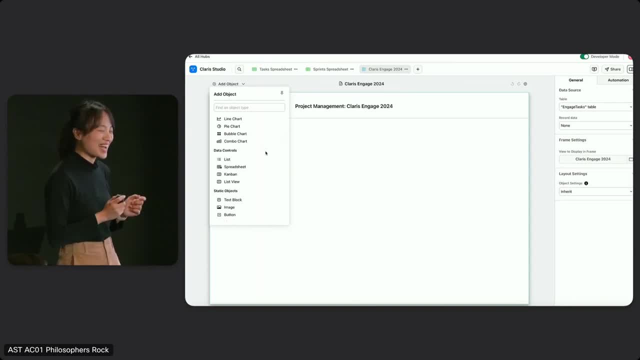 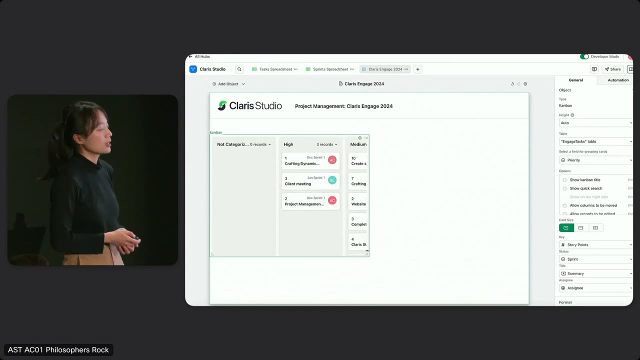 find the best representation for a data set. and now we brought all that power into custom view by componentizing them. yeah, so there, yeah, majority of the views here are now objects ready for you to use. and, for our case, we want to build a Kanban board. so let's drag Kanban into the view so, as you can see, as we drop it. 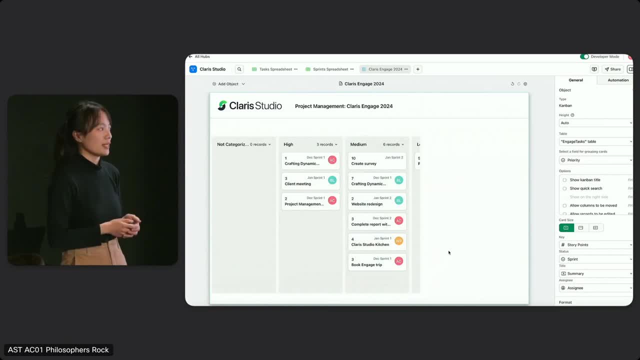 the Kanban is automatically populated with the task record and that's because the view level and next let's make some quick configuration together to make the Kanban board more usable. So for Kanban you can actually change the grouping field which will decide what columns to show on the board. 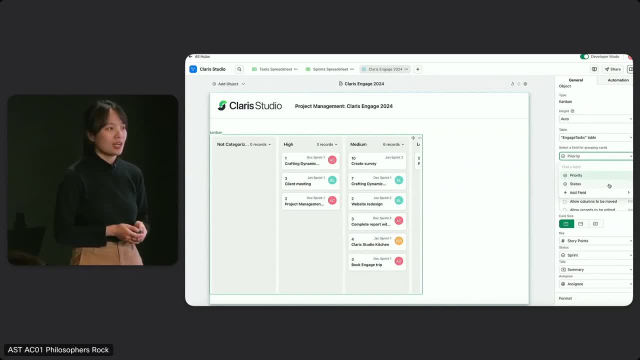 So this setting is also provided in the list view, So like, whenever you want to use group to represent your data and you can change it whenever you need to. And for our case, we want to show to do in progress and done columns, so we change it to status. 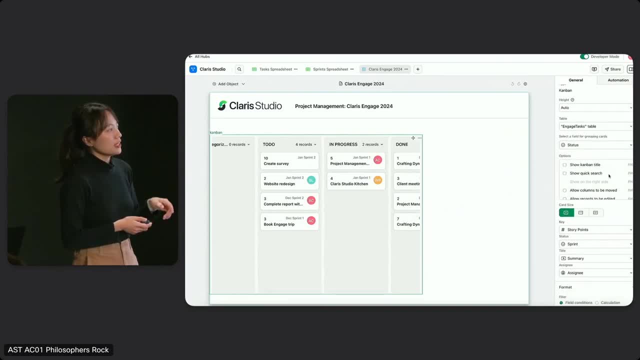 And below that in the options window. here are a few settings we can use to make the objects more customizable, And it might vary based on the needs of different data controls, objects, And for our case, we want to allow the records to be. 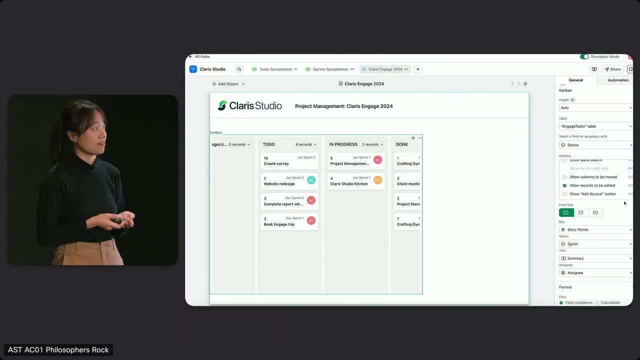 edited because I want my team members to be able to modify their own task, And below here are settings that you can use to customize your Kanban card. Again, the list of settings might vary based on different needs of different types of data controls. 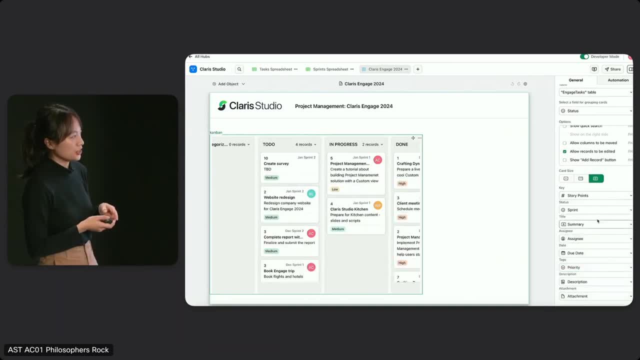 But from here we'll just make the card larger And you're actually able to select whatever information you want to display in your Kanban card. And below is the format section from where you can massage the data that your end user are going to see. 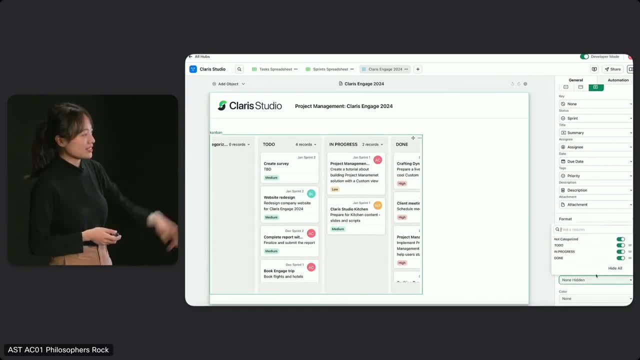 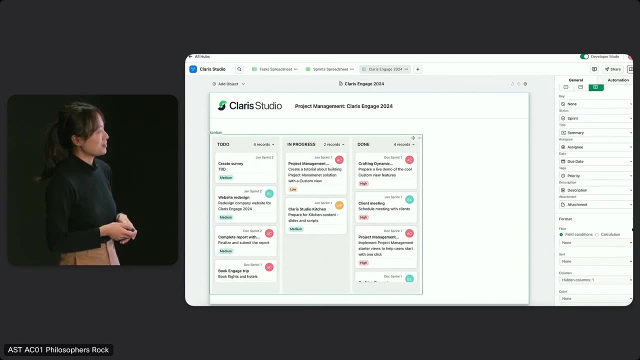 So we're actually going to. we'll be seeing the future settings very soon, But for now we'll just be hiding the not categorized column, since it's not as usable as others. Okay, And then, after configuring the Kanban objects, 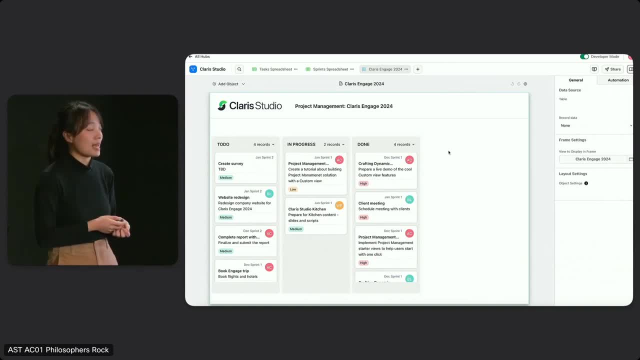 the next thing we want to do is to allow users to see and modify the details of the selected record at the same screen. So the way we're going to do that is to create a group that performs as a record form group. So first we will be adding a group. 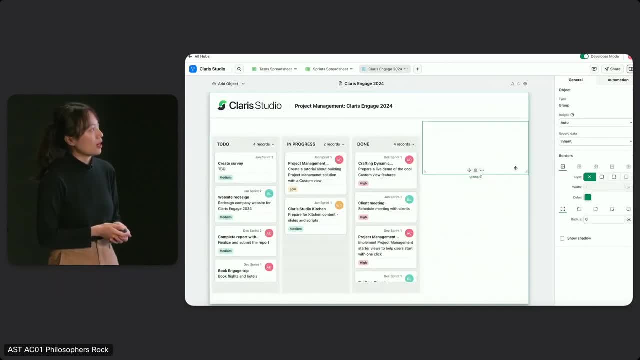 which is on the bottom of the list. We're utilizing the empty space on the right And then we'll be adding the summary object, which is the title you see here from the card, And that is, under the hood, a short text field. 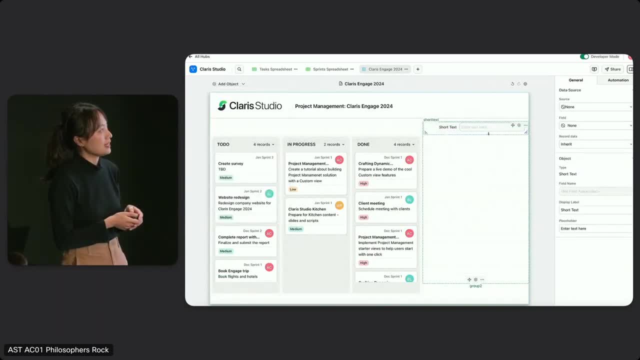 So let's drag a short text field into the group, quick and easy. And then we want to associate this short text object with the summary field in the task table. So we're going to the data source section again and simply assign it with: 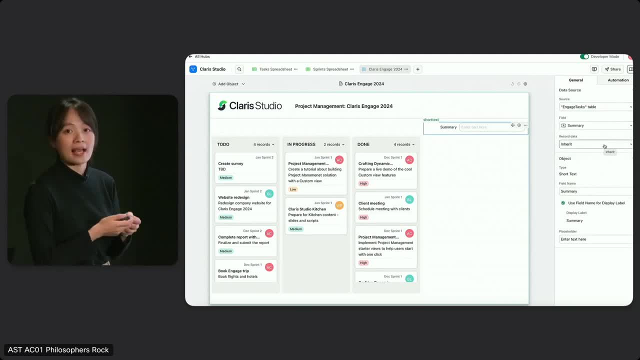 the correct data source we want And for record data, we notice that it's defaulted to be inherit. So what it means is that the objects will get the record ID from one level higher And in this case, it will get it from the group. 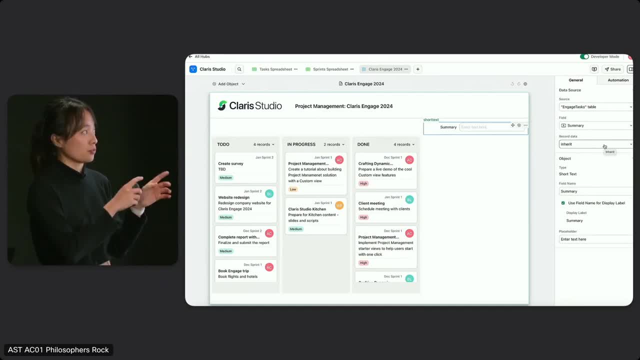 And later we'll actually be assigning the record ID to the group, because we want the whole group to be representing the same record. So we're going to do the same step for the description field, which are the text you saw here. 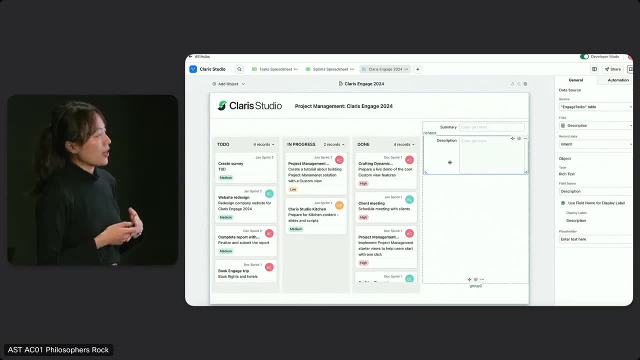 it's essentially a rich text field And we also, let's say we want a assigning field because we want to easily reassign a task. Okay, same step, quick and easy. Okay. and, as we mentioned earlier, since these objects are now belong to the same group, 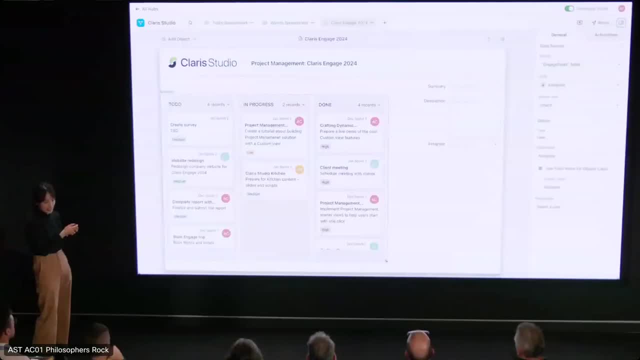 we're actually able to cite and position them all together instead of doing it one by one. So I want to get more space for my Kanban. I want them to align better. I can do that. So next, what we still need to do is to: 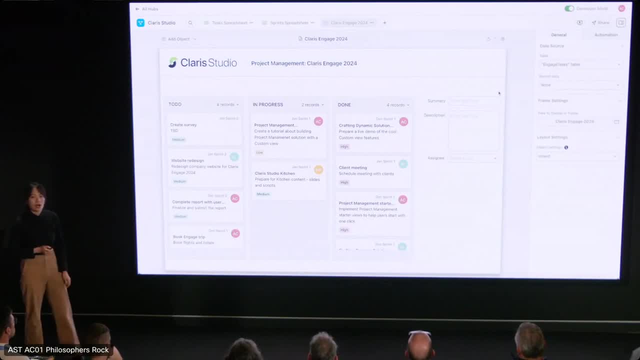 link the record form group and the Kanban. So the missing piece here is to calculate the record ID for the form group. So let's focus on the form group And then in the record data drop-down on the right we will switch to from calculation. 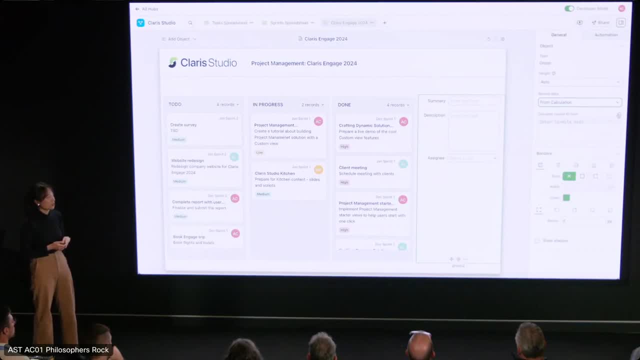 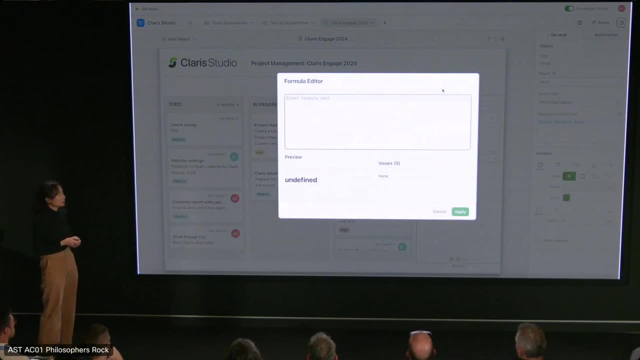 And from here we can open the formula editor, where we'll be using the calculation engine. Okay, cool. So from here, from the calculation engine, we can actually call the current view by its name. So we have this beautiful auto-completion to save your time. 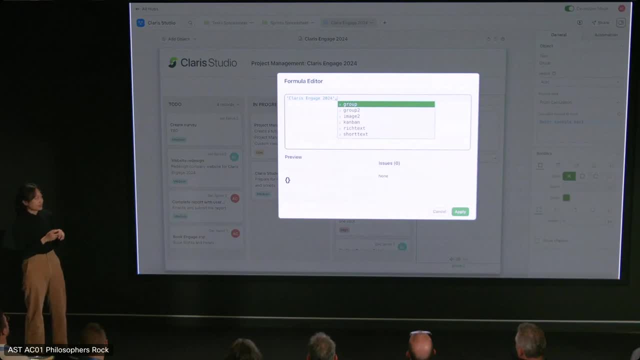 And then, with a dot notation, you're actually able to assess all the existing objects in this view. So for our case, we want to assess the Kanban objects, So let's do that. By default, the object names will be its type. 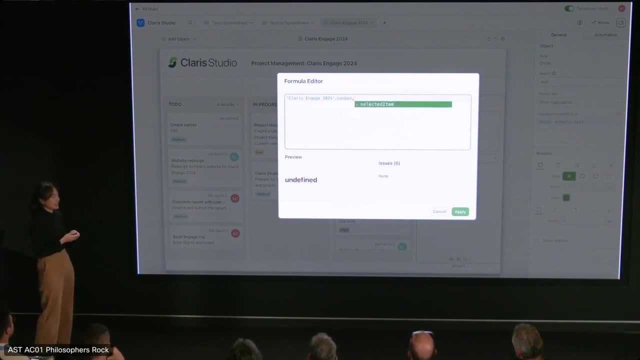 And inside Kanban objects we have this selected item property, Which is exactly what we want. And from here let's do one more layer. So from here we're actually able to assess all the field data as long as the record ID of that selected record. 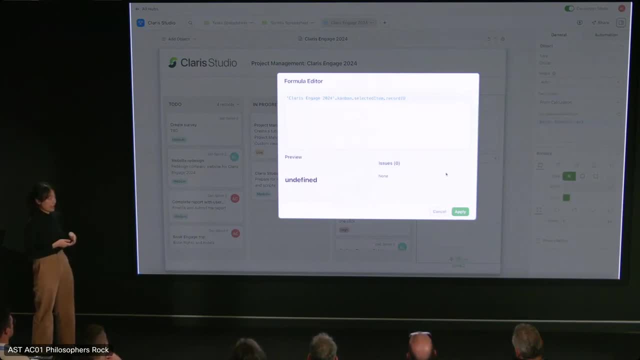 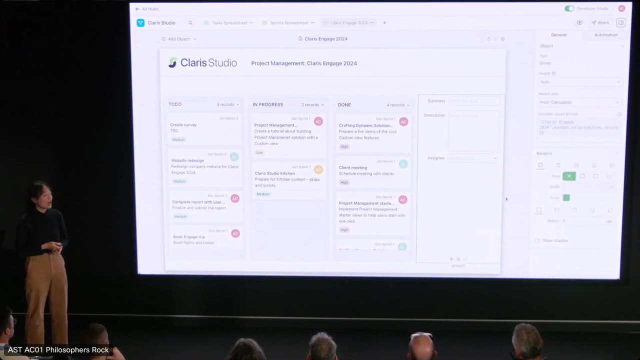 So for our case, we want the record ID And that's it. We can go ahead and apply it. So yeah, with the expression we just wrote, the group now is linked to the Kanban board And in Studio whenever. 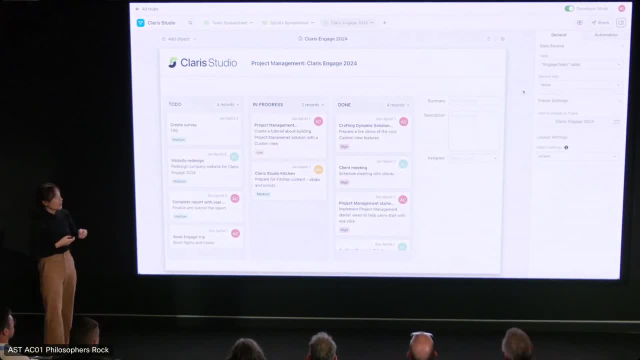 you're ready to test some changes you just made. you normally go to the top right, where we have a preview button, And then you will just open your app in a separate tab, So within a few seconds, okay, cool. 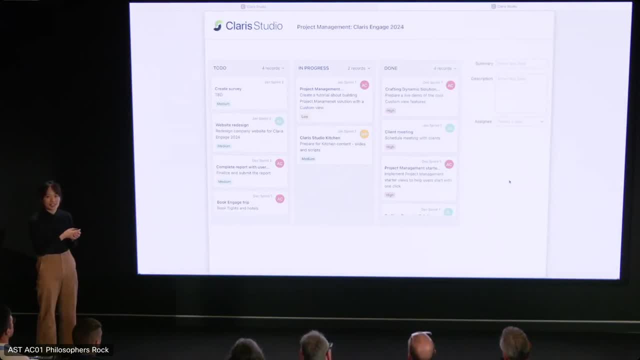 So, as you can see, now we've got a Kanban object displaying all the tasks from the table And we also got a record form group on the right. So whenever I click on a card, I will see the record being shown on the right side. 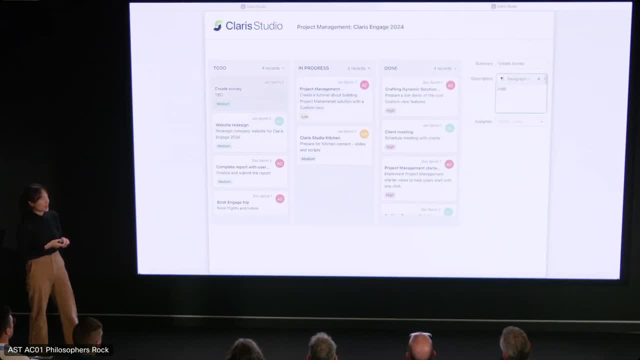 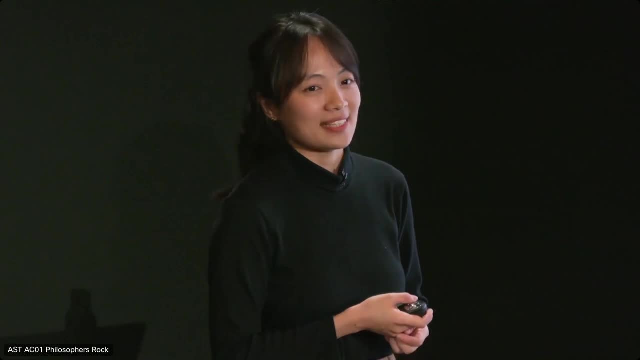 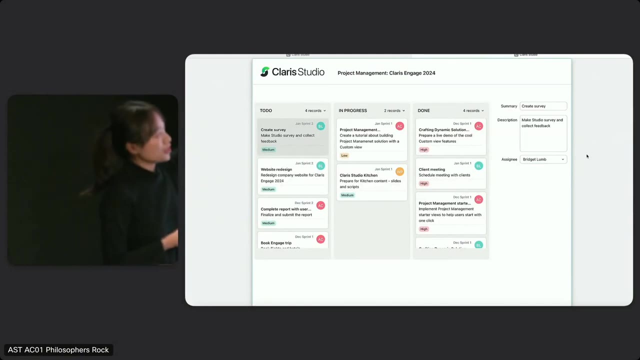 And I can also modify the records, Like here. I will give the task more description of creating a survey, And then I will reassign this ticket to Bridget, because she's the survey expert in the team. And, done You will see that all the changes we just made. 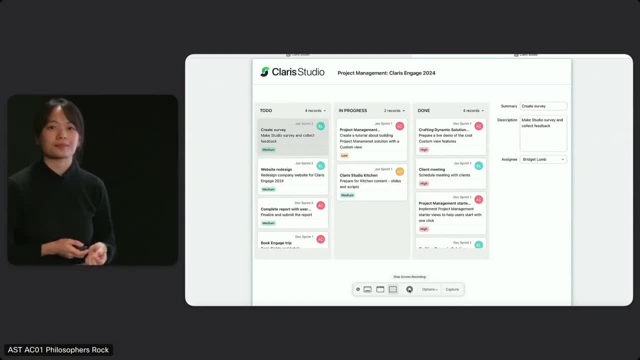 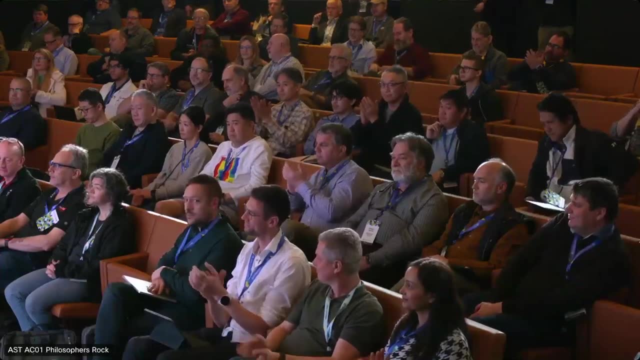 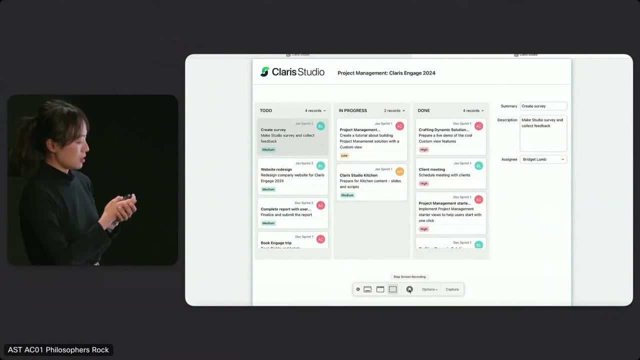 will be saved and reflected on the table. Okay, So now let's-. Thank you, Yeah, Thank you very much. Yeah, Thank you so much. So, yeah, Now let's take a step back and talk more about the calculation engine. 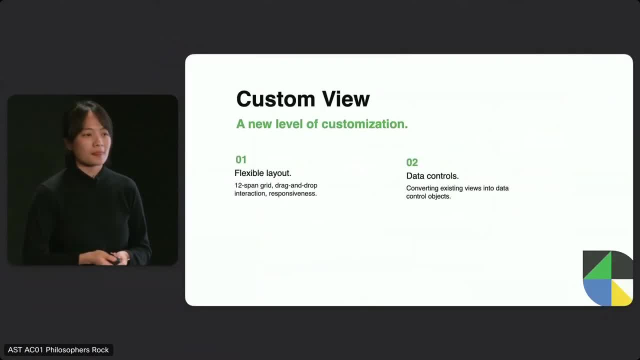 Oh, wrong button. Okay, So the association you just saw between the Kanban object record form group actually demonstrated the next critical power of a Studio Custom View, which is the power to control your own business logic. And yeah, 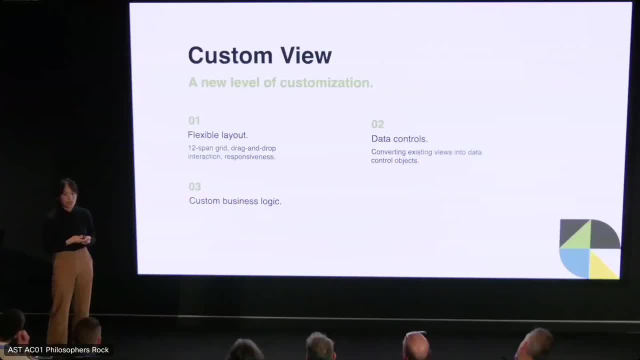 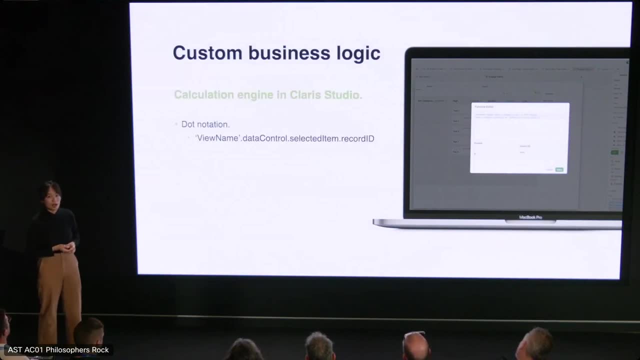 And the ability to program how your apps behave. And the way Studio gives entry point to that is through a calculation engine. So yeah, In the previous demo also sorry. So the calculation engine in Studio provides a functional programming language. 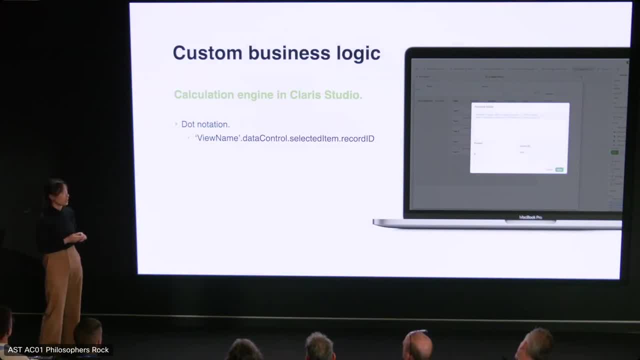 And in the previous demo you're actually seeing what we call the dot notation And with the dot notation you can easily reach into a view or any object properties that you might need for a business logic And, for example, for all the data control objects. 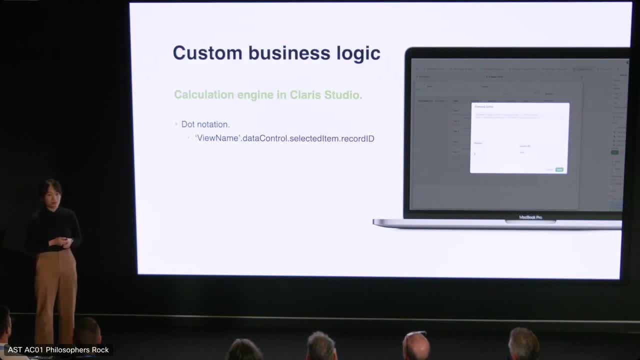 we actually provide this selected item property, which gave you access to all the record ID and field data within the selected record. And, yeah, Similar to FileMaker Studio, introduced object names. So by default, when you create an object, the object name will be populated as: 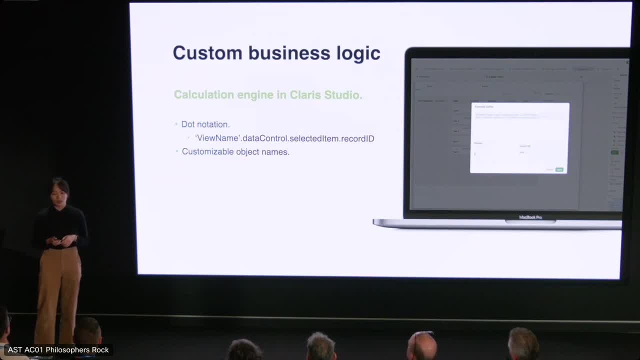 the project type, object type, with an unique index when needed, And as a developer you get to customize the name when you need, As long as the name is unique, so the runtime engine can always find the right object for you And the calculation engine consists more than. 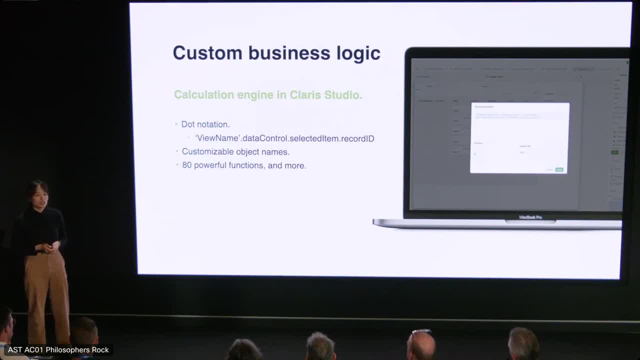 80 powerful functions that you can use. So under the hood, Studio engineering took a subset of JavaScript's functionality and added some new stuff, like specific functions or events, to handle different business use cases. So with this foundation, you get the JavaScript operator that you're already familiar with. 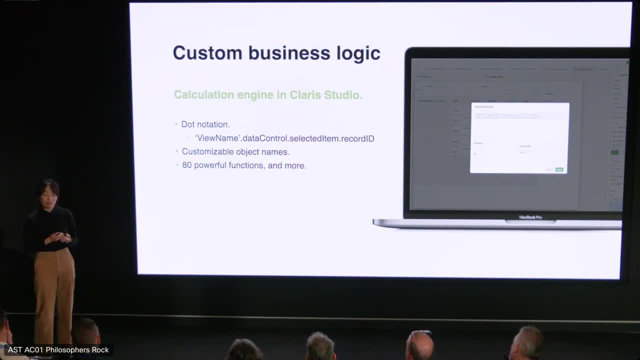 And you also get these powerful functions that can directly reference or talk to your Studio components. And on top of all this, all the functions we support are well documented for ease to reference and use, And we are adding more and more functions to the list. 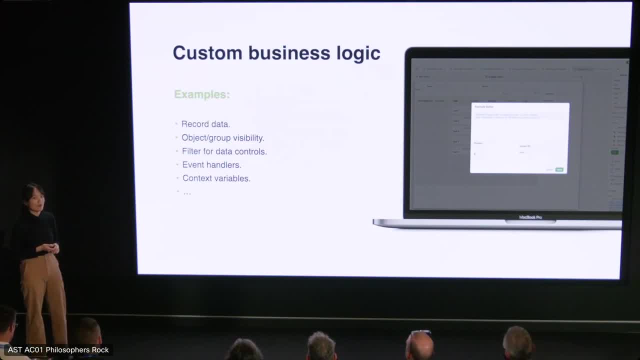 So here are some examples of the areas that our calculation engine are exposed to So you can use calculations for record data, like how we use it to associate a compound in the record form group. You can define conditions for showing and hiding an object or a group. 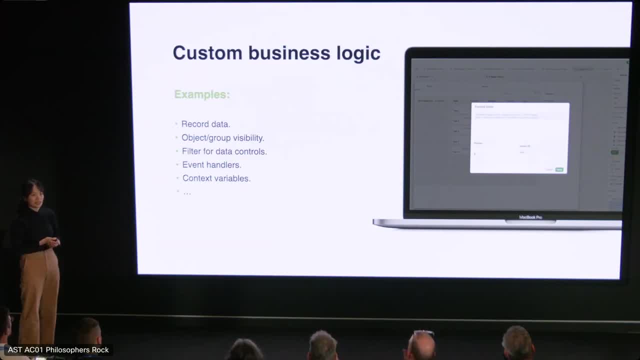 You can filter a table for your data control objects using calculation, And you can handle events with calculation. You can also define some context variables that can be accessed globally, across objects or even across views, And beyond this list, there are still a lot more for you to discover. 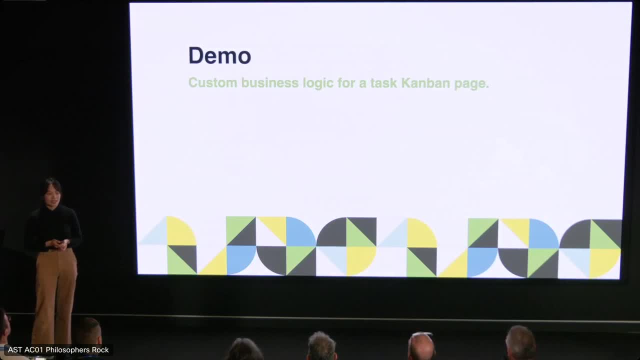 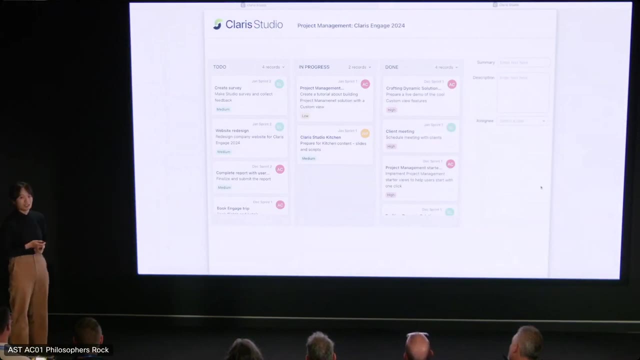 So for the next part of our demo, we'll be focusing on using calculation to control the form group visibility and the data filters for our common objects. Okay, so now let's look back at our common app in Studio. So first let's make a quick improvement together. 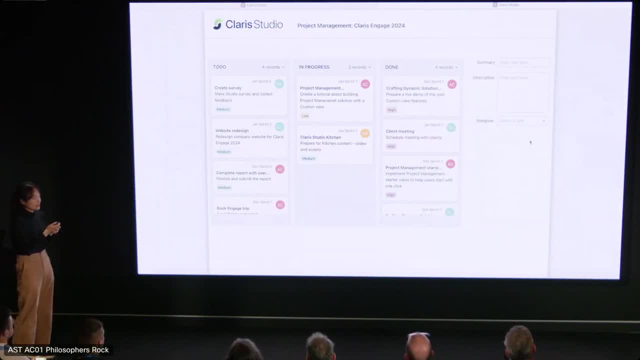 So in this screen, when there is no record selected, we notice that the empty form here might confuse our end users of what they can do. So let's say we want to hide the group dynamically when there's no record selected. So let's go back to the developer mode. 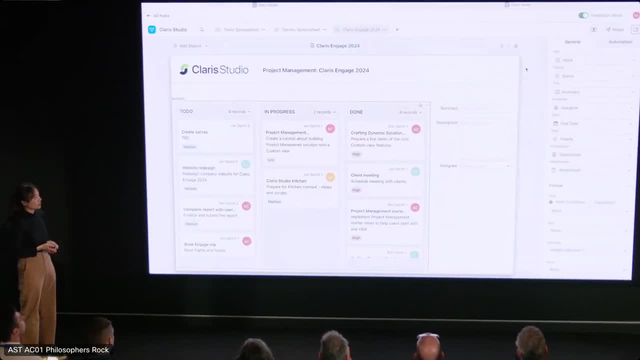 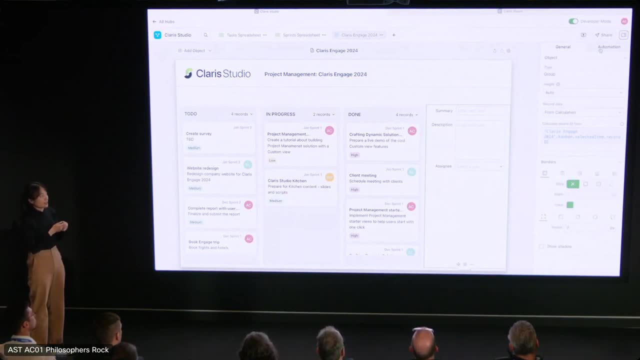 And we want to focus on the group. So in the top of the problem list we have a list of all the objects that we want to control, And on top of the properties pane there's also an automation tab and from where you can customize your object names. 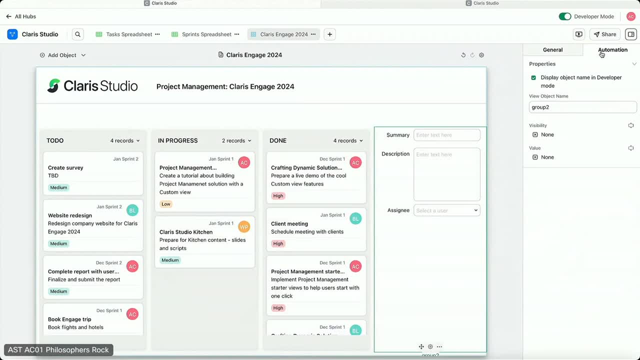 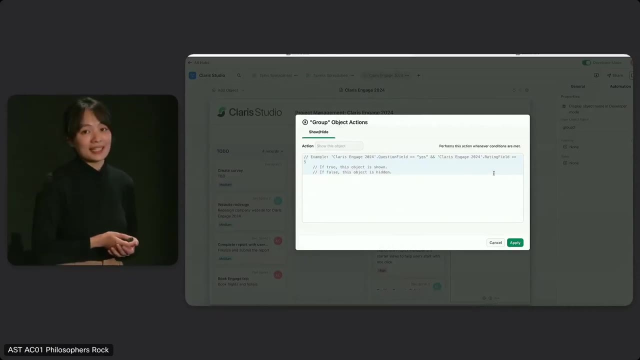 like we talked about earlier, And we also support you to create automation events, so like setting visibility or setting the value for a field. So for our case, let's open the formula editor for the visibility. So basically, here we want to write an expression that returns: 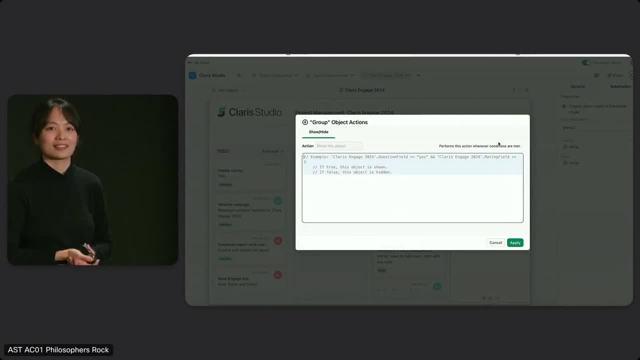 true, Only when the selected record ID is not empty. So we can do the same exact same thing to access the selected record ID, Select the item record ID. cool, And from here we're going to use a function called isBlank. 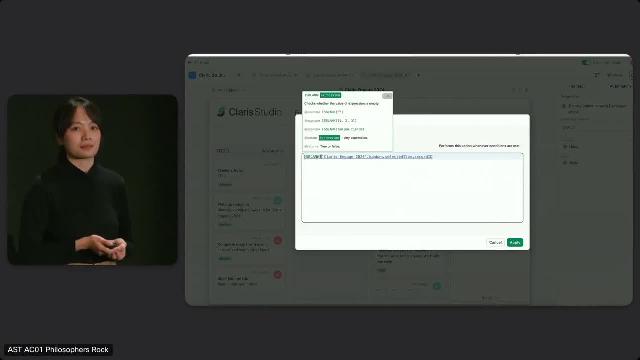 to help us check if the record ID is empty, And, however, we also want the functions to return true only if it's not empty. So we're going to just add a not operator, which is from JavaScript, And then, yeah, we can apply the expression. 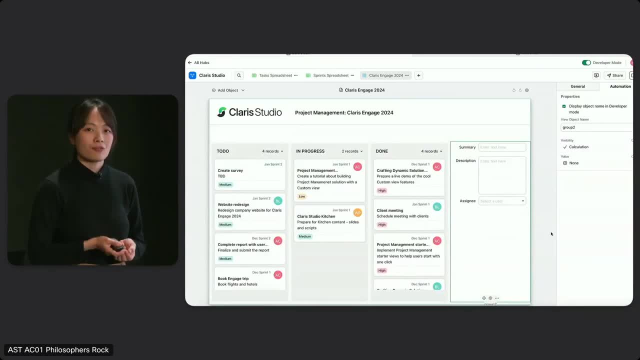 And that's it for the group visibility And for our next use case, I want to help my team member easily find a test through a custom filter mechanism. So in our team's use case, we used agile developments, which means that we would like to focus on the sprint to. 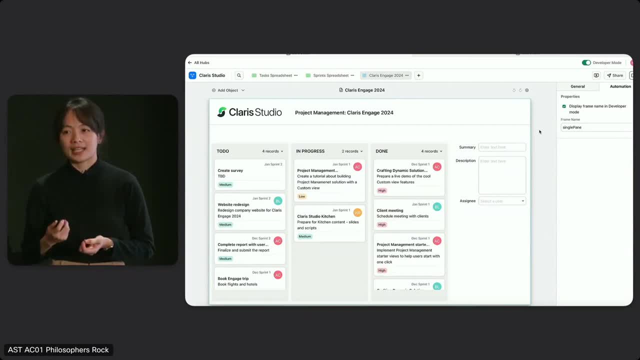 understand the team's day to day progress. So we'll be doing that utilizing the future calculations and future calculation for data controls objects. So let's go ahead, and so, first of all, we want a UI element to allow the team member to select a sprint. 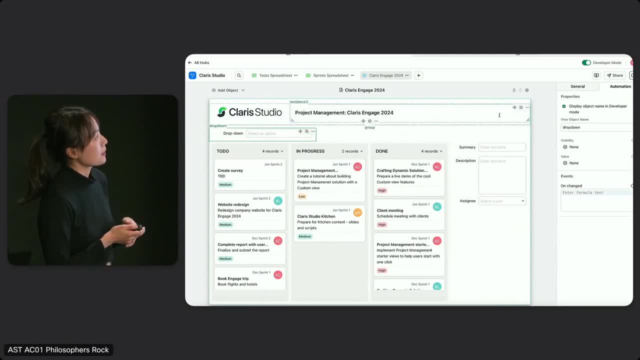 So we will just add a drop-down object And from here we will associate the drop-down objects with the sprint field existing in task table And for the record data we're actually going to leave it as empty. So this is exactly the use case when we want to use. 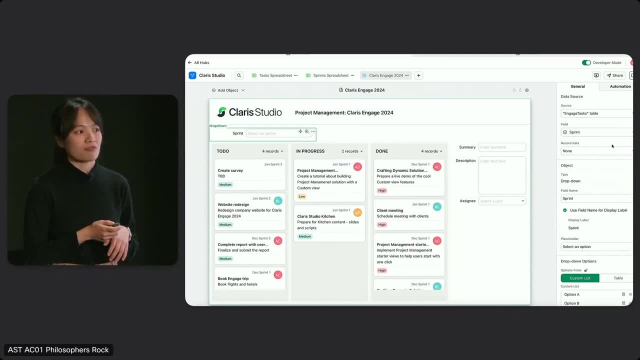 a field objects as a UI control and not associated with any record data. And then I want to do one more thing. this time, Let's go to the Automation tab and gave the objects a customized name, So let's call it SprintSelector. 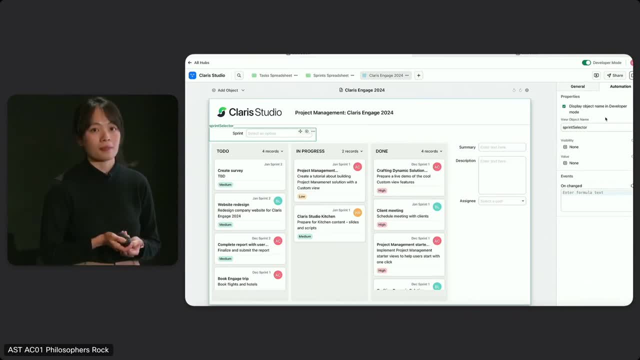 So it's easier to identify in CalcEngine. Okay, cool. So what we still need to do here is to link these two objects. So we want to come on to filter its data based on the selected value inside the sprint drop-down. 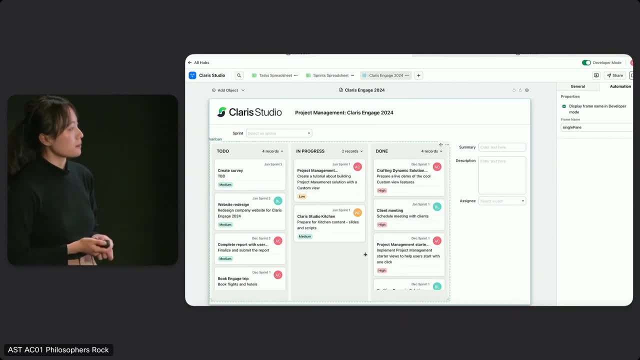 So let's focus on the combine again And from the properties pane we want to go to where we saw earlier: the filter settings. And instead of doing a fixed filter, we want to do something more robust and we want to introduce our own business logic. 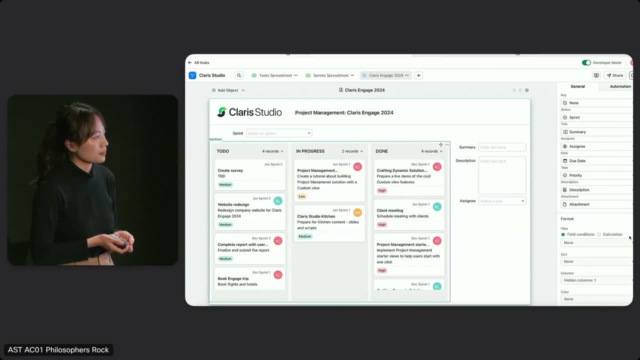 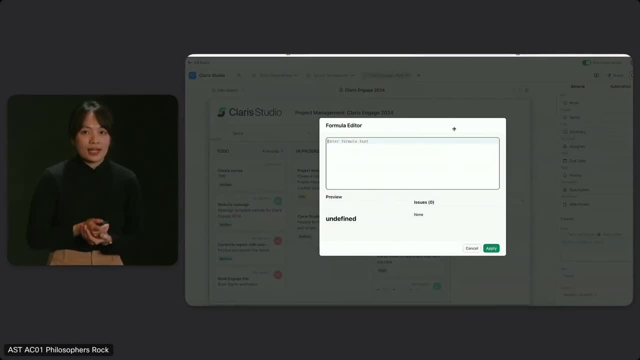 So let's switch to calculation, Calculation And again let's open the formula editor. So what we need to write here essentially is to compare the sprint column data with the sprint drop-down value from the field. So we mentioned earlier that you can call. 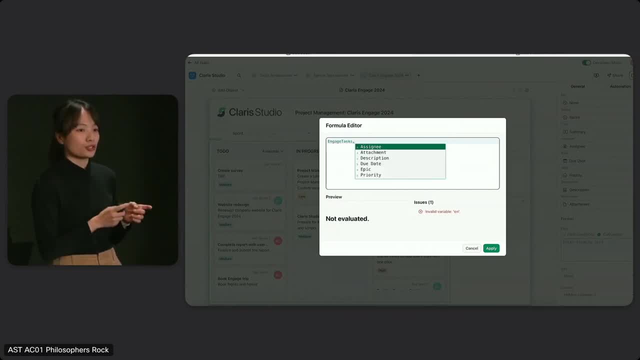 a view directly inside the calculation engine, and that is also true to a table. So here I'm calling the EngageTask table and access the sprint column. use double equal for comparison, And then I want to assess the value from the SprintSelector. 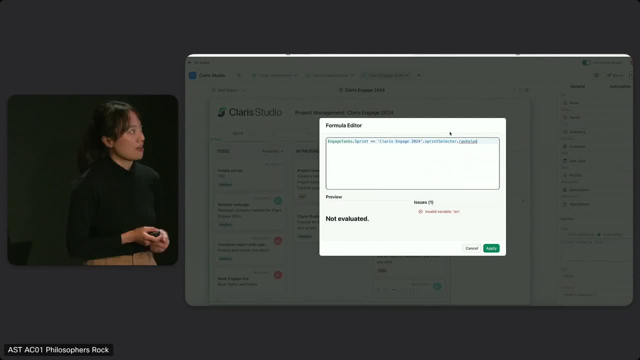 which we just gave a unique name so it's easier to find, And for our case, we'll use the raw value property. And, yeah, this is the core expressions that we need, But, however, we also want to handle the case when 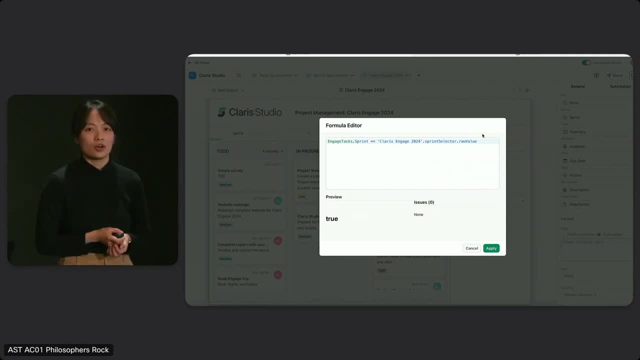 the sprint drop-down is empty. So with this expressions when no sprint is selected, it will actually returns the tasks that are not assigned to any sprint. But that's not what we want. We actually want to show all the tasks by default. 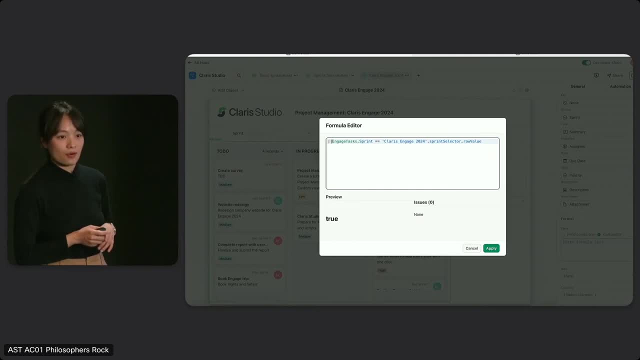 So to do that, we just need to add a OR operation and we'll use the isBlank function again. It's a really useful function. So this time we'll be targeting the SprintSelector component. Okay, cool And done. 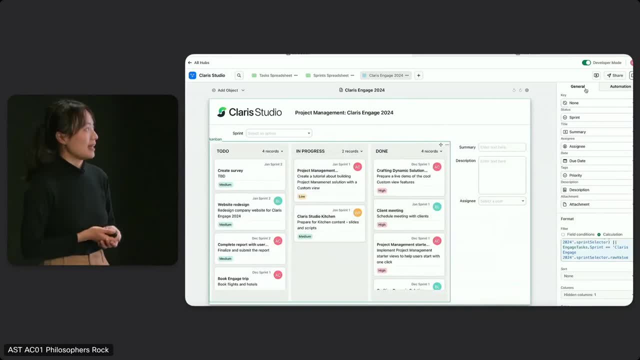 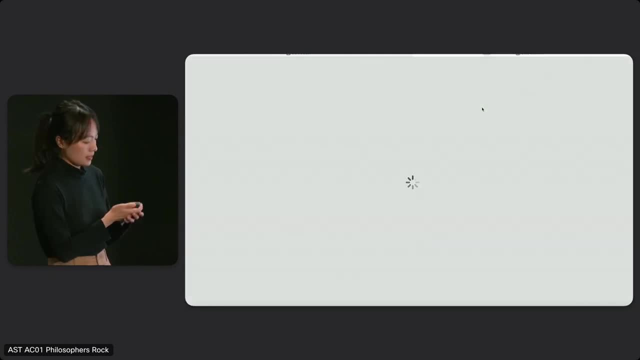 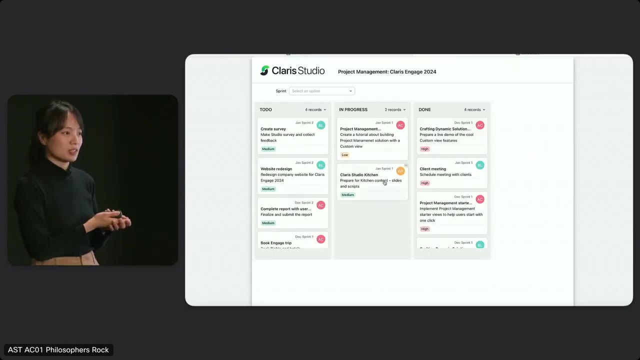 This is the expression that we need, And let's go test our app again. We'll refresh it this time. Okay, cool, So we see that by default, we only see the task come on board And when I select the record. 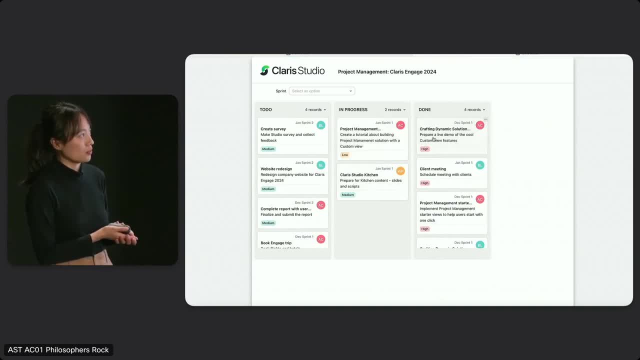 the group will show up And when I deselect it will goes away. Perfect. And also I can choose the sprint to focus. Yeah, So when I choose a sprint, it will only show the task for that sprint And with that context. 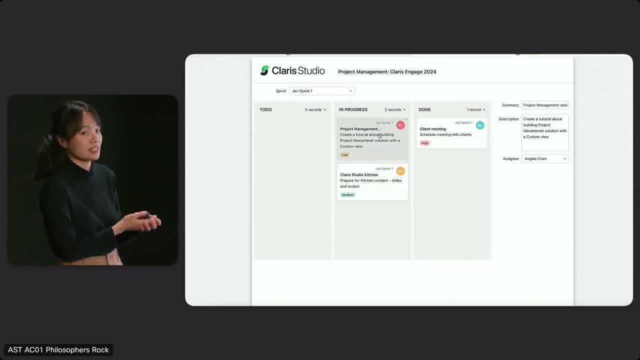 I can still focus on the task, to see the detail, modify the detail, And I can always clear the sprint selections to see all the tasks again. So, yeah, all of these happen on the same screen and we just build this beautiful, dynamic task. 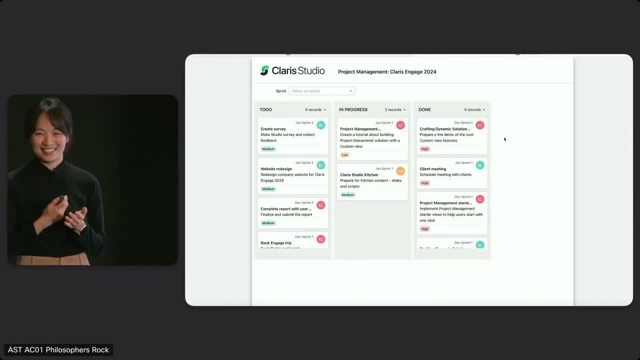 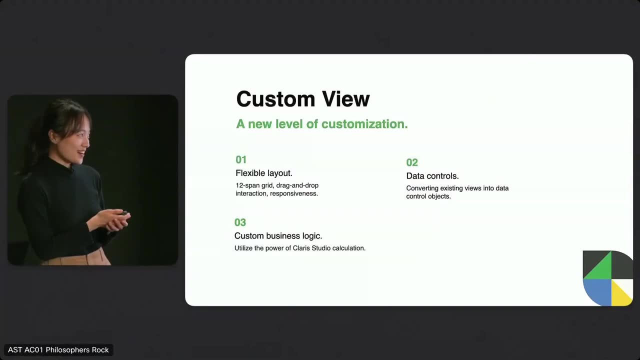 come on page within a few minutes. Cool, Yeah, Thank you. So yeah, here are even more cool stuff about Studio Custom View that we can't wait to give to your hands. And next I will hand it back to Bridget. 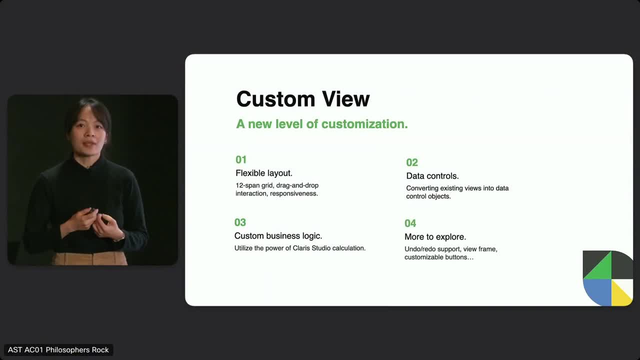 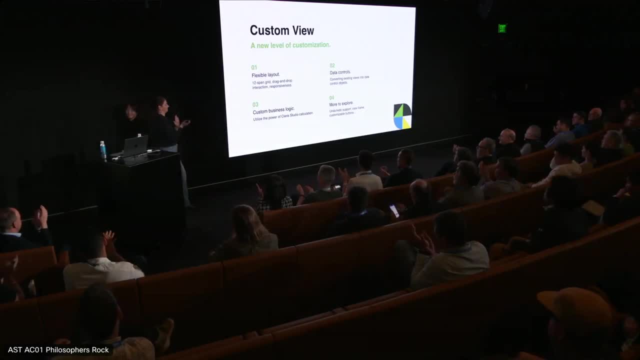 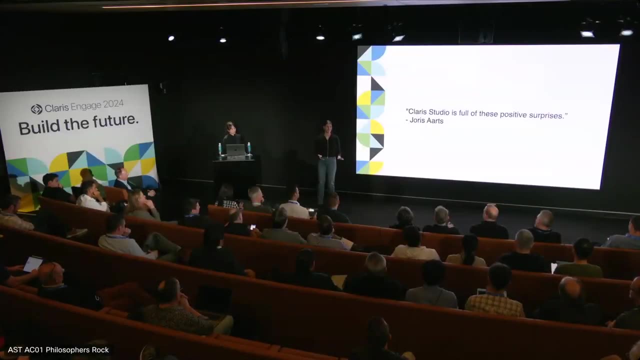 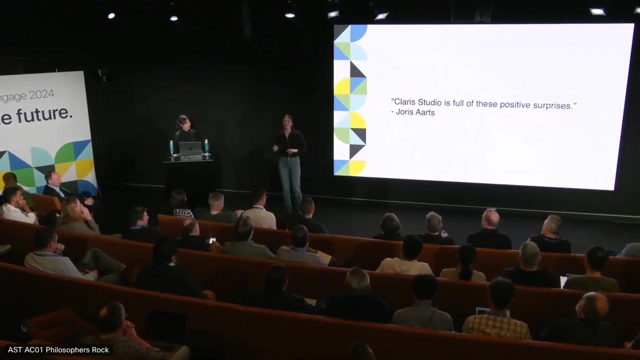 to talk about ways you can get more exposure to Studio and play around with all these new cool features. Thank you, Angela. Okay, Let's take a second to process all of that information And, as you take this in, let me show you a few more examples of how all of 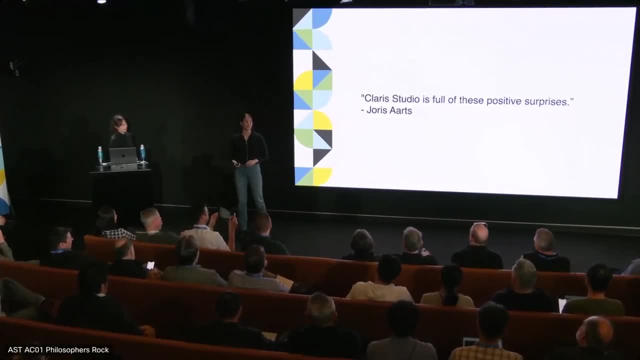 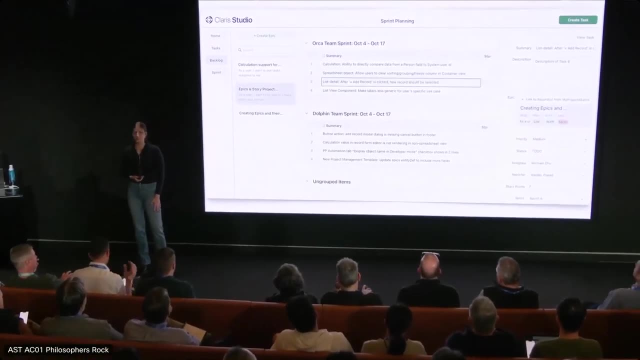 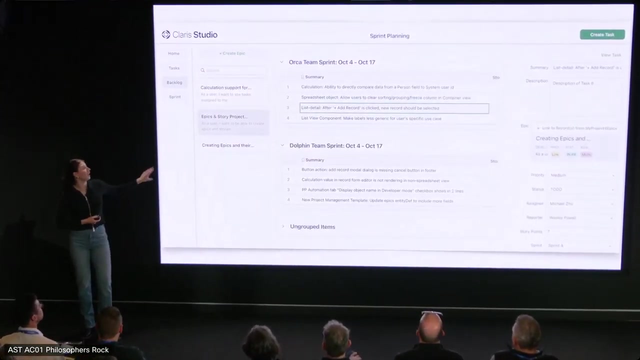 these cool new features can and are being leveraged by some of our partners today. Like I mentioned before, we wanted to use Studio ourselves for our project management, And this is a snapshot of what our Studio front-end teams are currently using. today, I would love to take a deeper dive into this. 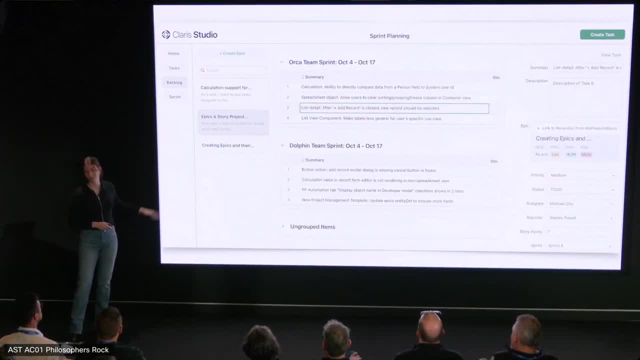 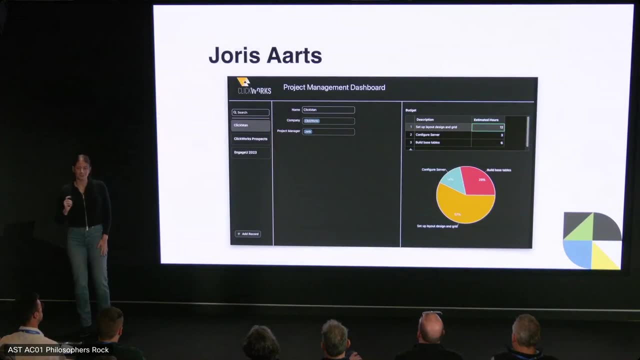 but please come visit us at the product booth to show you all the cool features that were set up in this project management template. Yoris Arts from ClickWorks, who's sitting right here, is working on building a project management dashboard to leverage internally that he might be able to. 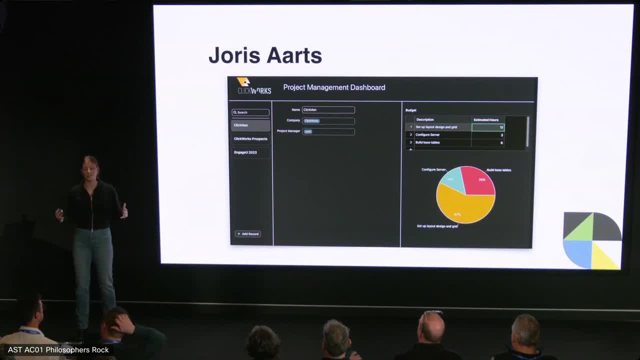 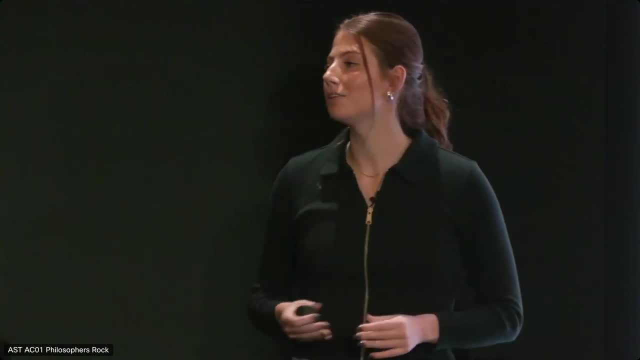 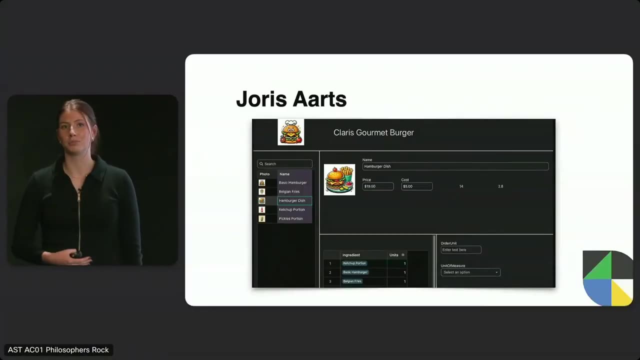 replace his current tool with so that it's all in one platform, But in playing with all the exciting new features that Studio has to offer. he found a real-world use case for his restaurant and hotel clients, taking about three hours to build a proof of concept for. 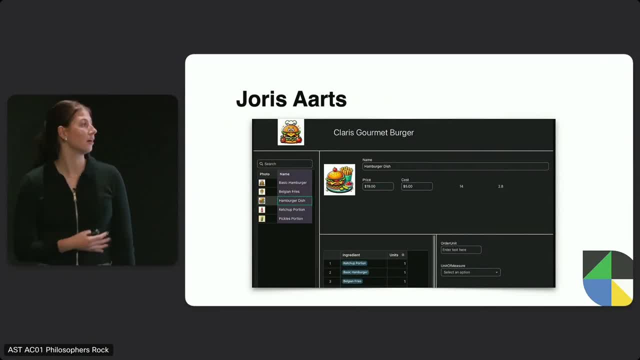 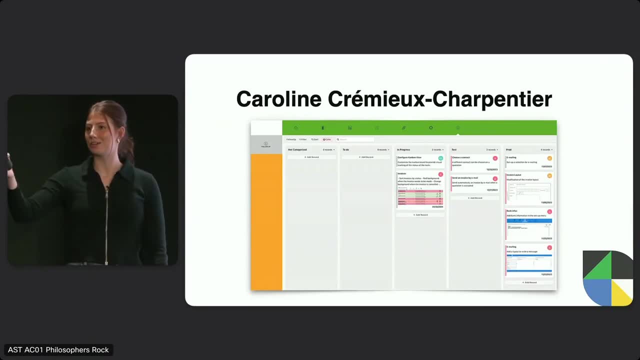 a food cost dashboard that calculates the cost of preparing meals using a recursive element that he can leverage for his clients. Caroline, who's also here today from Aqua, uses the Studio Kanban view embedded in her FileMaker solution to track the status of her projects with her clients. 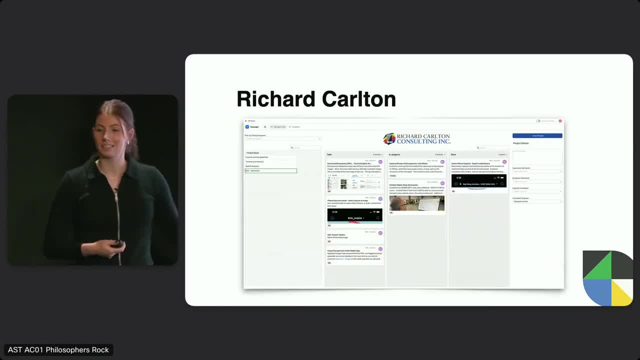 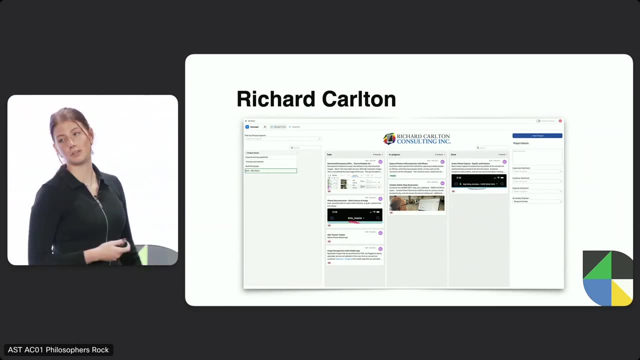 So it's all in one place. And lastly, as I showed in the keynote, Richard has a solution to extend his current project management solution to his clients. Now we got to meet with Richard in person, which I found extremely valuable. 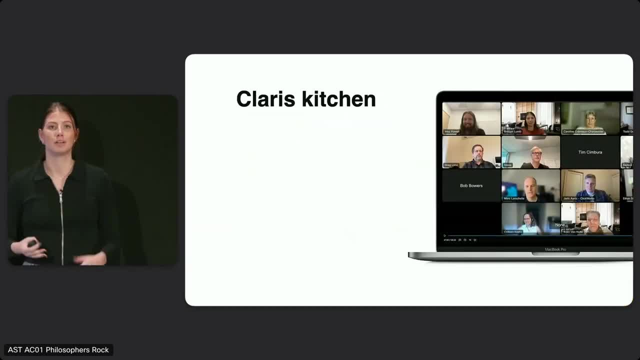 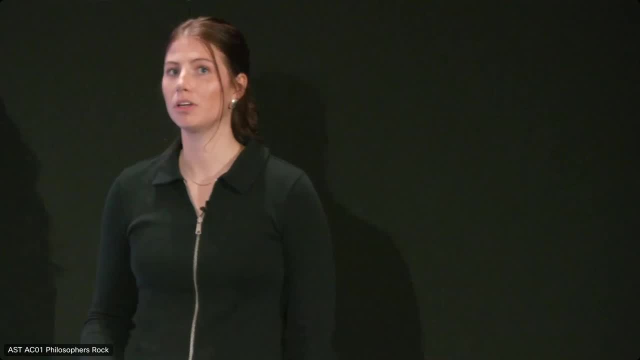 just like being with all of you here today. In fact, your feedback is invaluable to us, which is why we created our Claris kitchen. We gave a group of about 15 partners early access to a custom view and asked them to build something of. 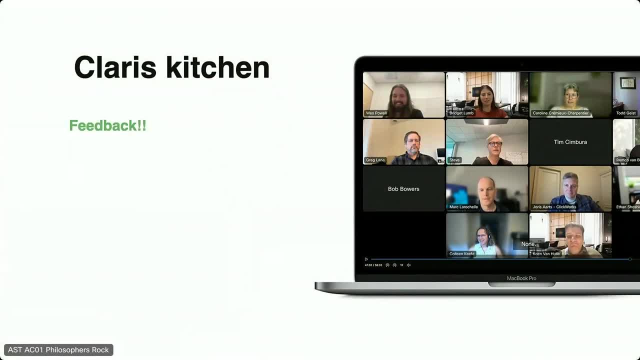 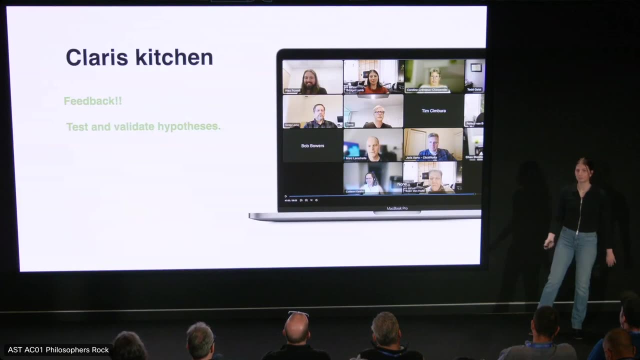 value and work closely with us to provide feedback. We wanted as much feedback as possible on what we were building, And we wanted it early and often so we could test and validate our hypotheses and ensure that we were delivering new value, And we wanted our partners to have a community to build with. 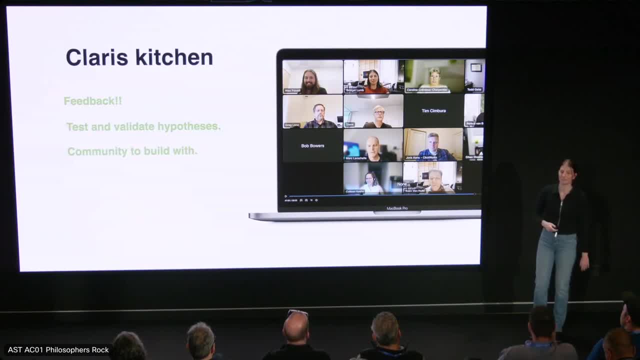 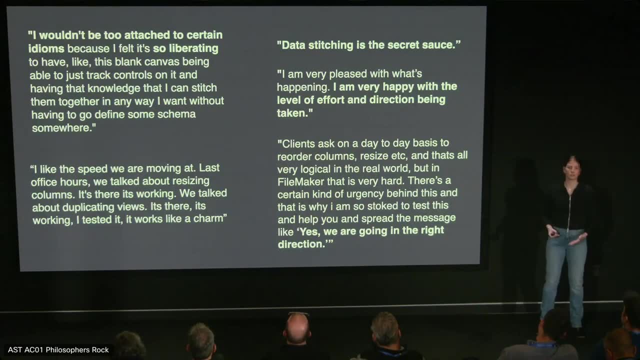 And our partners took off running. as you can see from the examples, We host office hours about every two weeks and this is an optional time for the partners to come and ask questions, give demos, feedback or just to listen. The time is theirs and the office hours is actually. 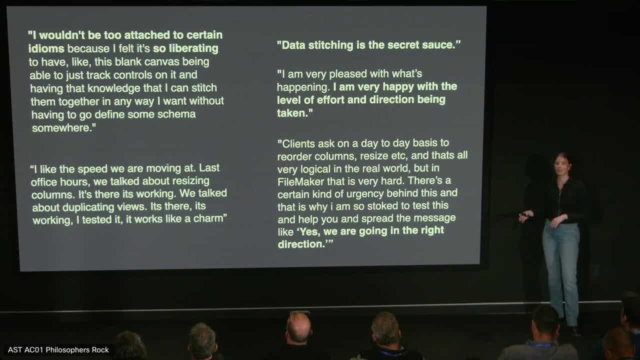 I would say my favorite meeting as of late, Even though the meetings tend to be early and I'm not a morning person. everyone is so eager and excited to chat and I love hearing all of the partner stories and feedback and use cases around this that even we didn't think of. 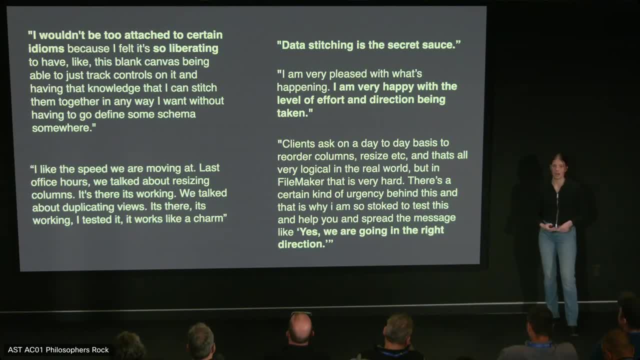 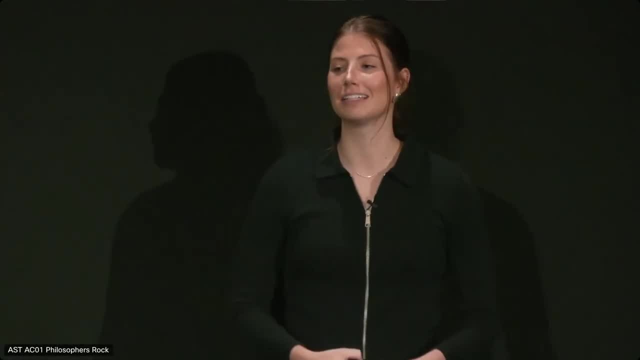 So with the kitchen, we've created a community of partners to build together and interact with one another. In fact, for example, Remco is clearly a studio champion and he will beat me to answering questions that are posted in our Claris community group before I can get to it. 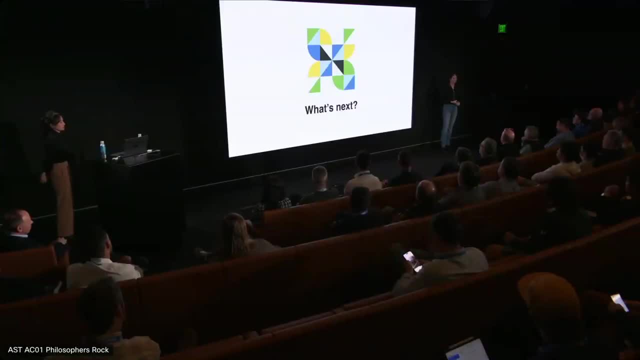 Now what's next? As Giuliano mentioned in the keynote, we are currently working to get a free tier of studio available to all of you. And so, as Giuliano mentioned in the keynote, we are currently working to get a free tier of studio available to all of you. And so, as Giuliano mentioned in the keynote, we are currently working to get a free tier of studio available to all of you, And so, as Giuliano mentioned in the keynote, we are currently working to get a free tier of studio available to all of you. 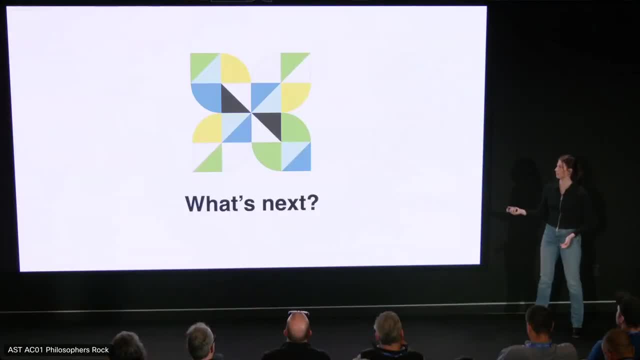 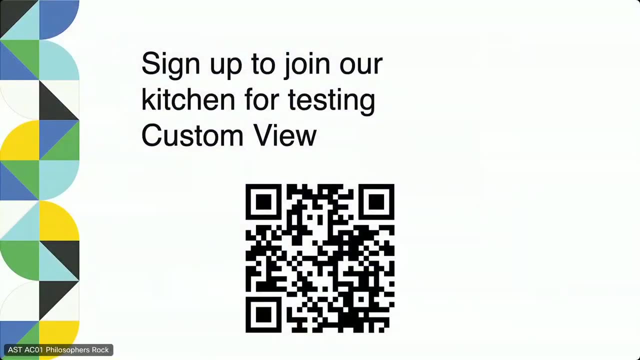 And CustomVue will be coming with this, But as we continue to scale testing, I want to talk to more of you, So please scan this QR code to sign up to get early access to CustomVue and join our kitchen. Please note: we're going to work with developers that have a lot of experience with custom view. 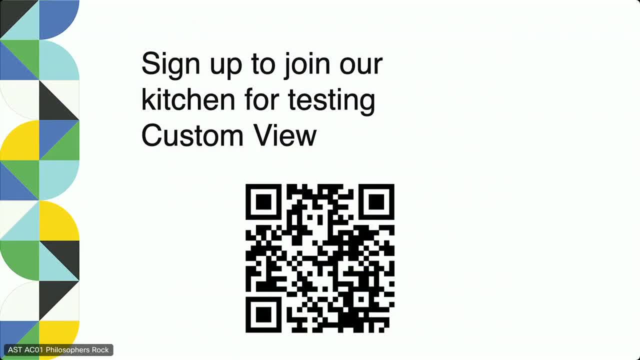 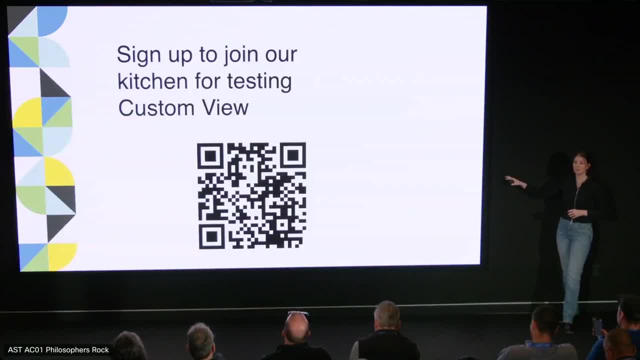 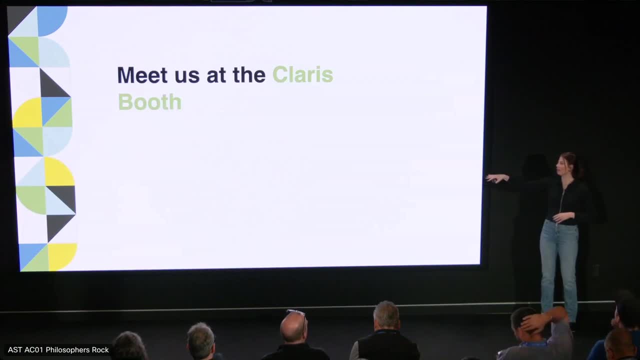 have a use case. we hope we can leverage and have the time to build. Luckily it's not that big of a time-ask. I will also have this QR code at the product booth, So please stop by. Angela Remco and I will be hanging around the product booth at these times. 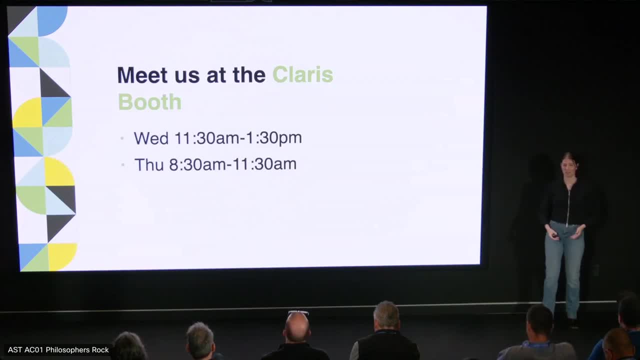 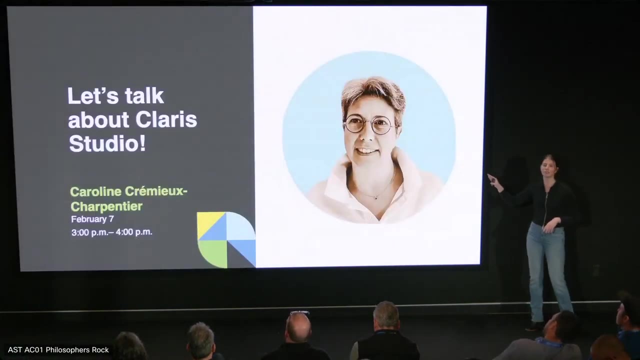 Like Angela mentioned, there's a lot more features that we did not have time to demo today and we would love to show you And do live demos for you. So please stop by our product booth. But that's not it. Caroline has a session later today on Klerus Studio and what's in market today. 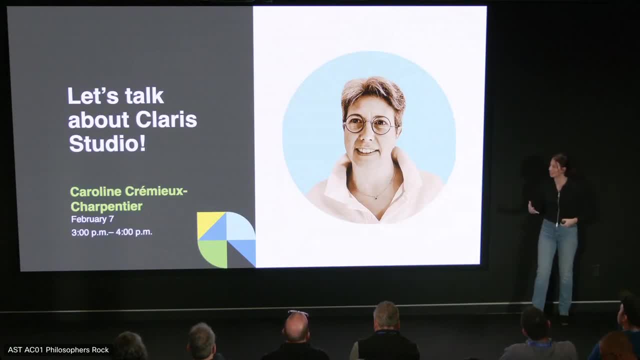 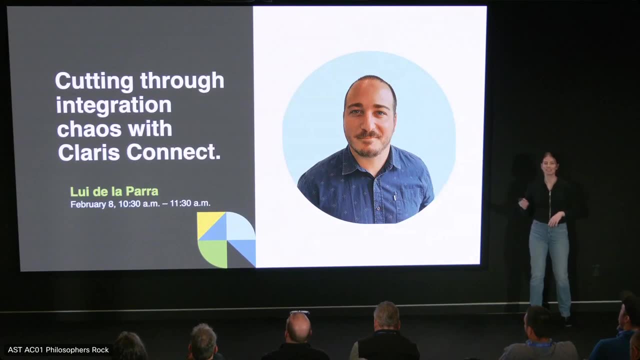 to help give you guys a fundamental understanding and help orient yourself with the new product. Willy de la Parra also has his session cutting through integration chaos with Klerus Connect where he's going to talk to you about how you can do this. 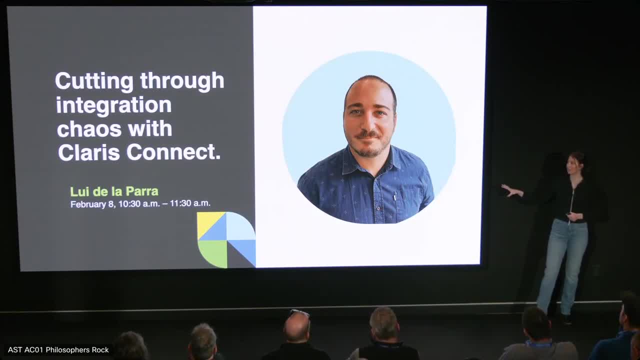 And he's got some pretty exciting things. We have connectors relating to Studio so you'll be able to programmatically create things in Studio, And he'll be demoing some of that as well, and that will be a part of our kitchen. 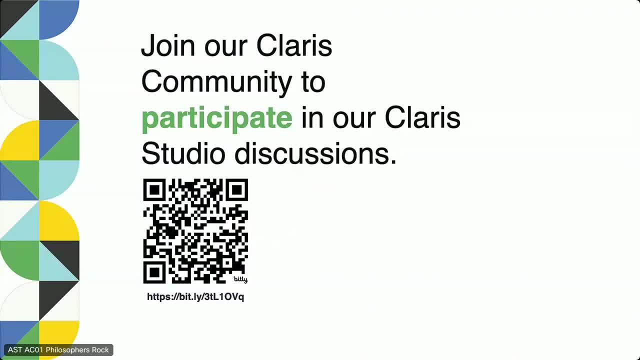 Lastly, join our Klerus community- if you haven't already, to participate in our Klerus Studio discussions. I'm excited, I'm beyond excited, about where custom view and Studio as a whole is going, As you can see from our partners. 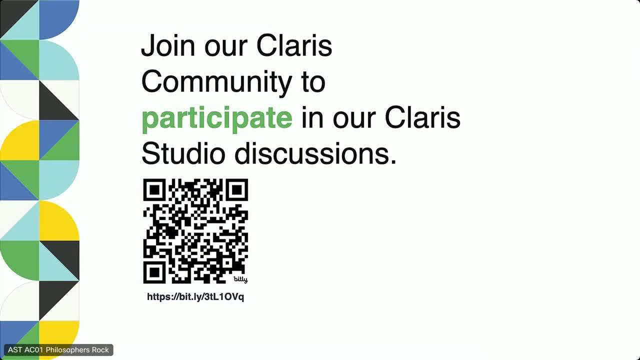 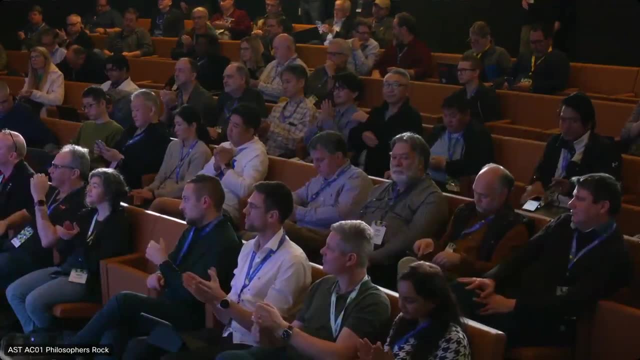 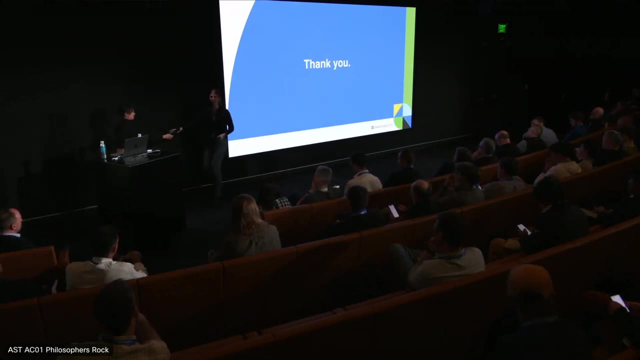 there's a lot of excitement around it, and I hope that you all feel my excitement and can join me in this journey with Klerus Studio. Thank you. Now we have ten minutes for Q&A. I have a microphone too, Uh-oh. 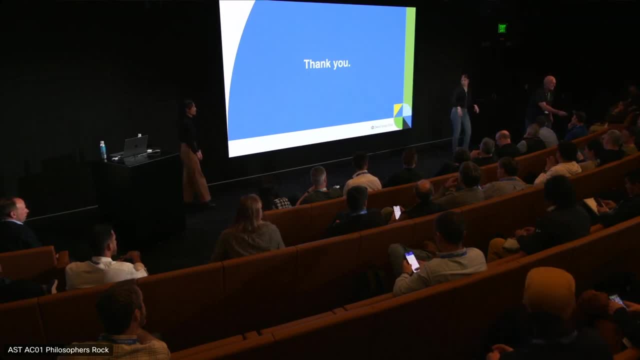 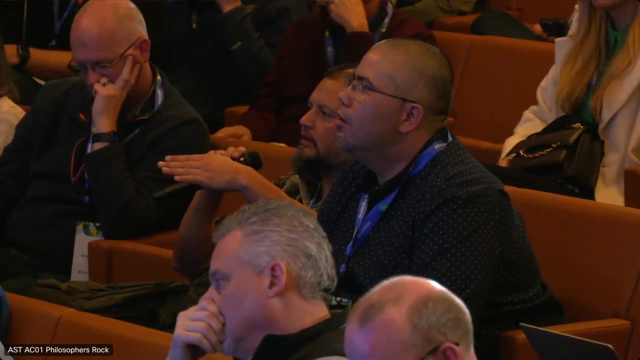 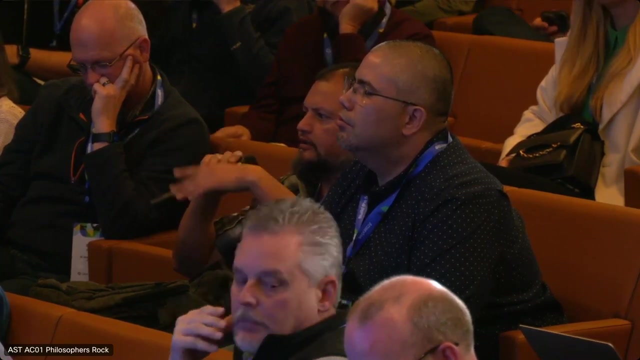 Hmm, Oh, okay, As far as the access, the user actually logging into this new Studio, is that still following the same authentication that is set up in your server, like using some form of IDP, or how is access to this view? 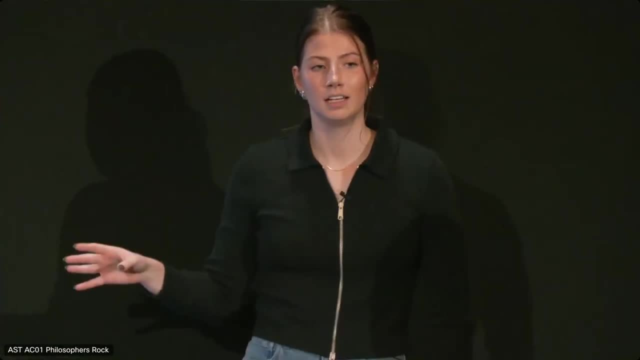 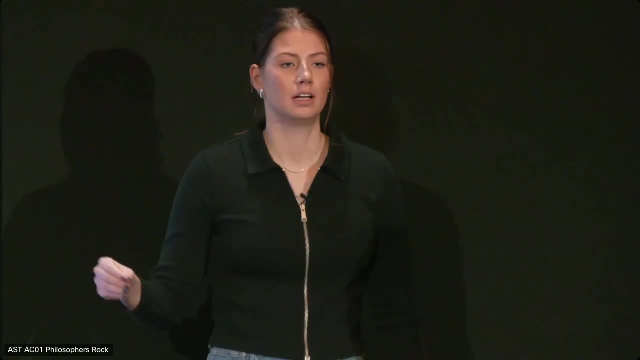 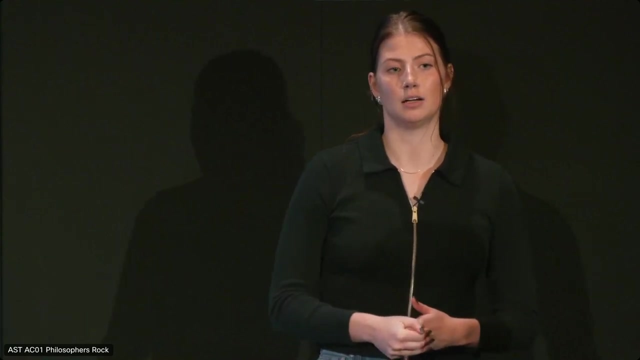 Good question. So currently Klerus Studio is supported with Klerus ID, So to develop in Klerus Studio you need a Klerus ID. That being said, like I said in the keynote, we're working on getting those views. 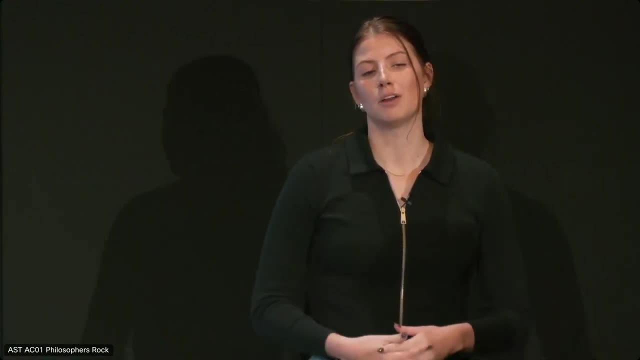 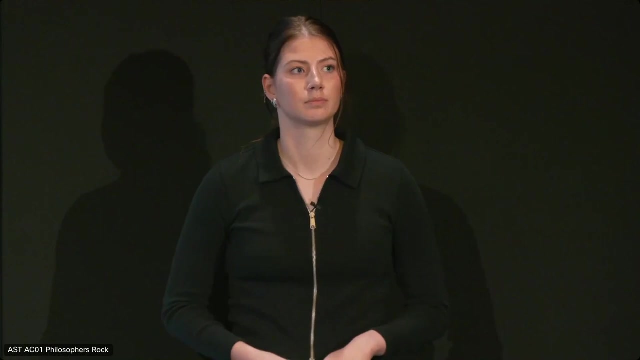 You can share views publicly with a URL and we're also working on groups and permissions. that's an external auth with Studio, As we know that's important. Going back to that, on my use case, we have about 4,000 providers all over the United States. 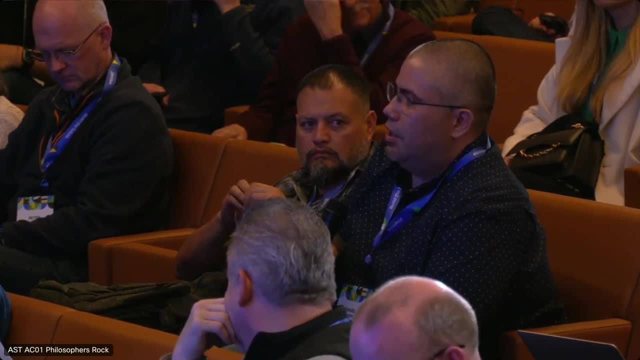 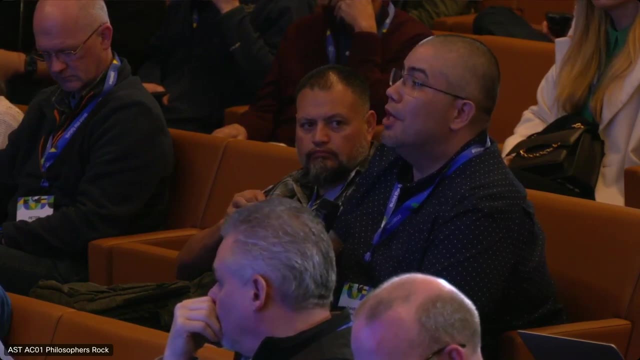 If I decide to use Klerus to build a dashboard for them, what kind of license are we talking about here? I'm going to have to pay per user per session. What's the deal? So we're currently working on the licensing. 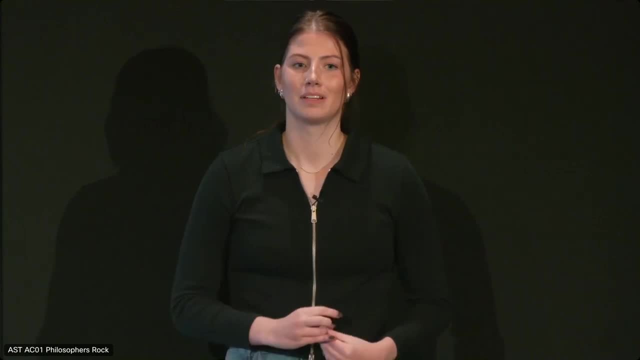 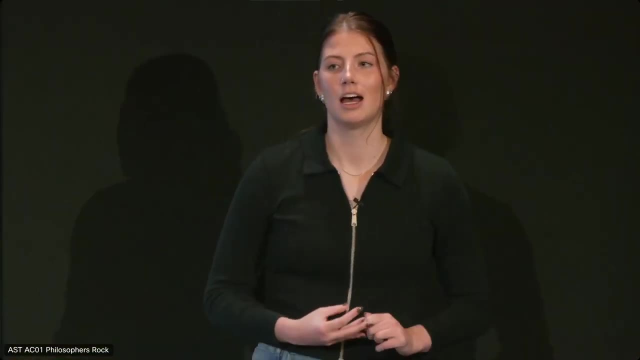 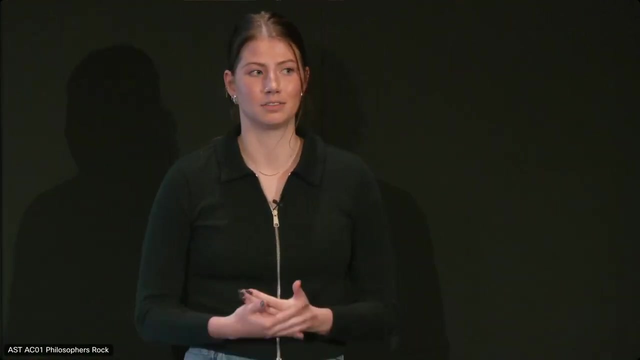 for that right now. So this is not a mature solution at this point. So in my case, right now we're not even exploring, because I think you should explore. It is becoming mature. We are working on the licensing and we are looking to not make the same kind of mistakes. 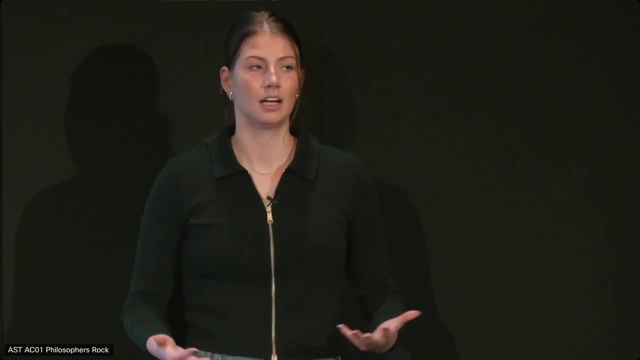 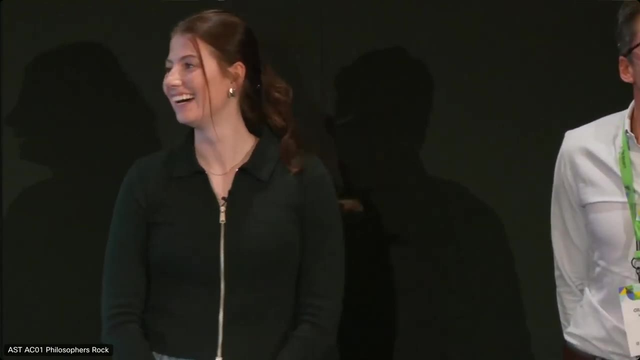 we made with WebDirect in that licensing and restricting data collection. Juliano is also the one currently working on the licensing so he can speak to that. Can you say again the size of the deployment? We have 4,000 providers all over the United States. 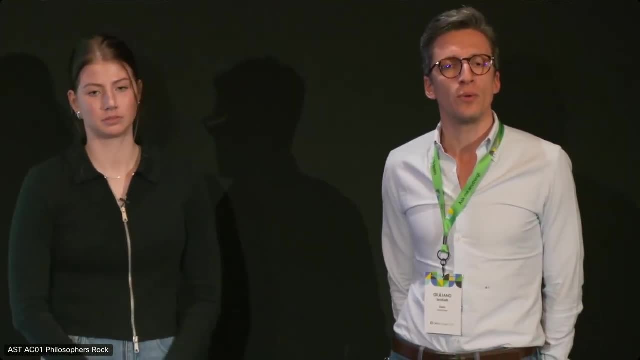 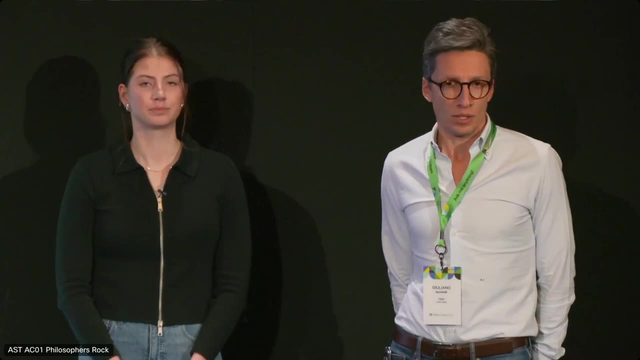 and the network is expanding on a daily basis. We are projecting probably for 6,000 by the end of the year, by the end of next year. But you're talking about external users. External users In a way, so people that wouldn't need a name. 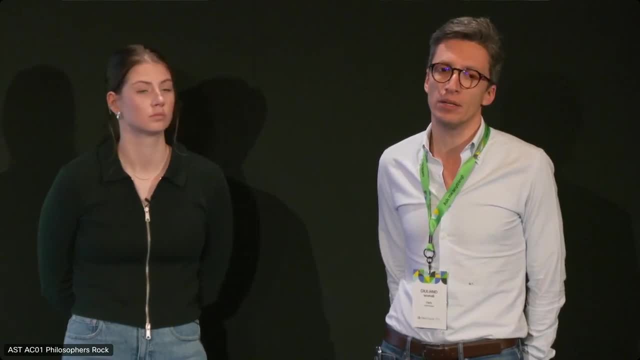 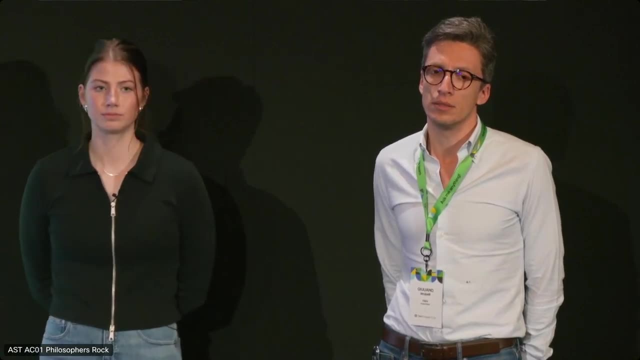 account the way you would- No, they do Right now- you would do it in FileMaker. So how the work is. I'm going to give you a simple user case. So we schedule appointments with providers all over the United States. for a reason today, 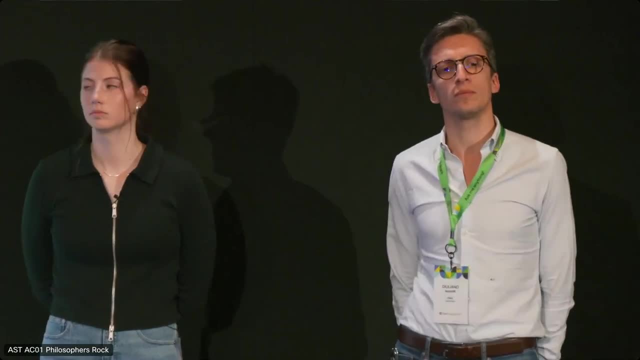 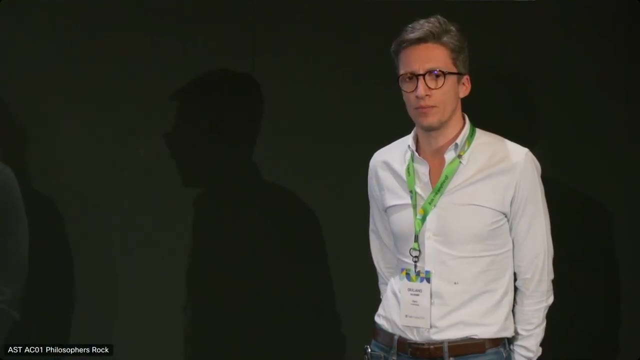 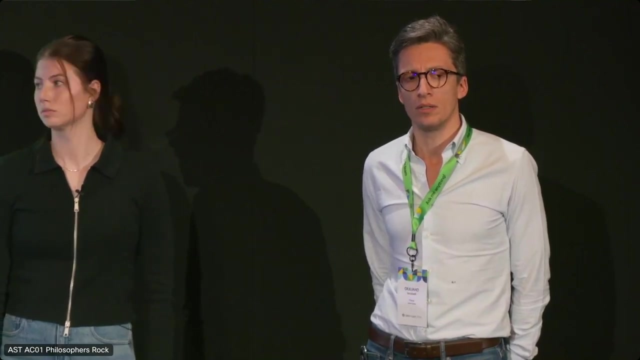 So sometimes the provider has to reschedule that appointment. If you give them a dashboard, it can go ahead and just cancel. It's a simple deal For appointments. Okay, So I have 4,000 providers, So you still. That information is still behind a set of credentials. 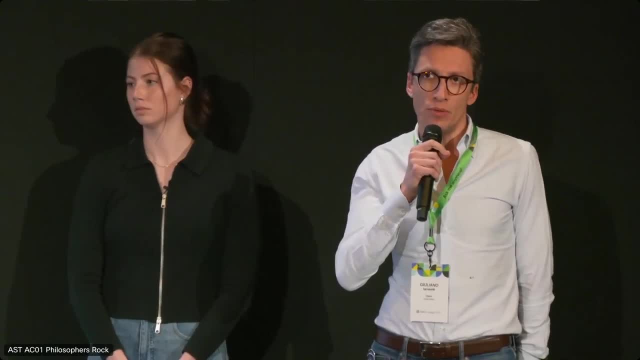 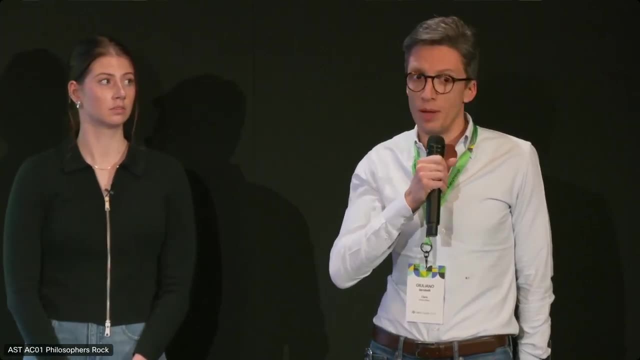 Okay. So on that aspect, if that's not what would be a traditional name user on FileMaker, from that aspect, that would be a product of Studio that would not be available right now, Not as a get-go. really, The view that 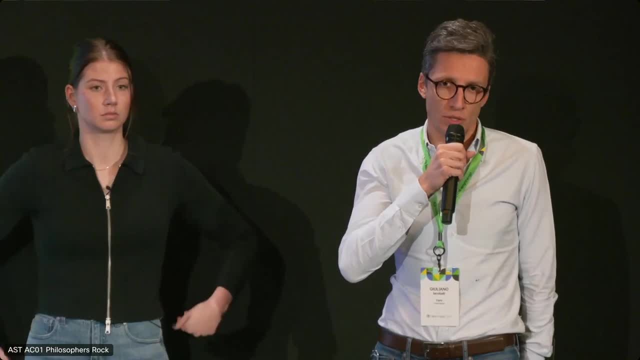 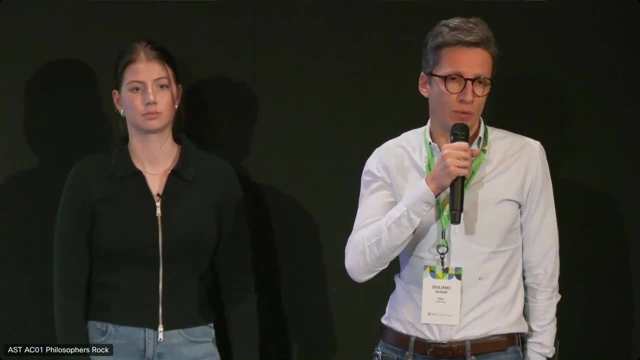 has shown, are for now designed to be for public consumption only, So they won't be gated by credentials yet. The moment we'll get there, that will become a more structured approach. We're going to have a more structured approach there, But right now. 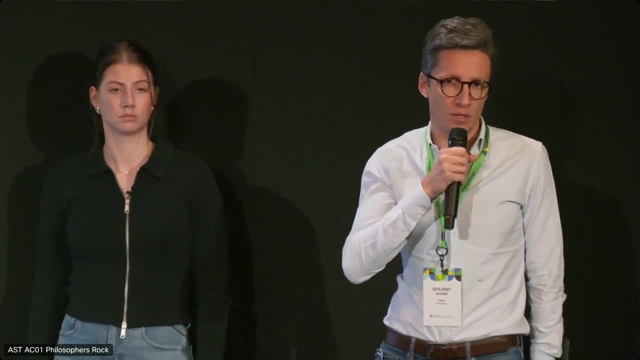 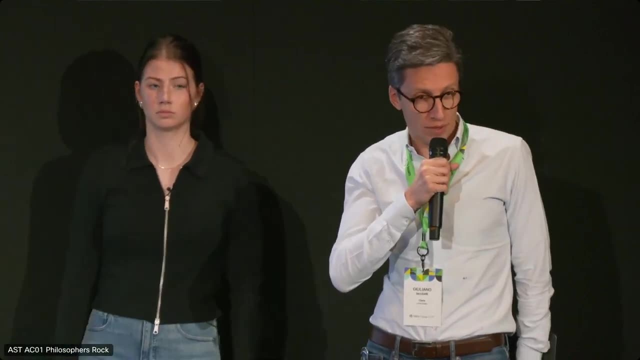 if you have any use case where you don't need somewhat of an identity that needs to be recognized in order to access to a view, we won't be metering that based on my number of users. if we're talking about external-facing people. 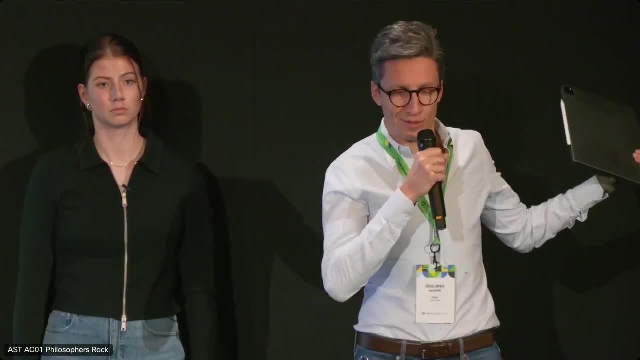 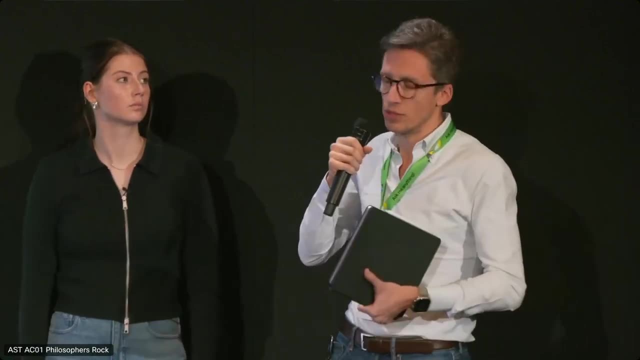 I know that yesterday the table about licensing has been up for a few seconds so you probably couldn't grasp all the details, But primarily what we're going to meet their studio around to begin with, because they're not going to have a separate user pool. 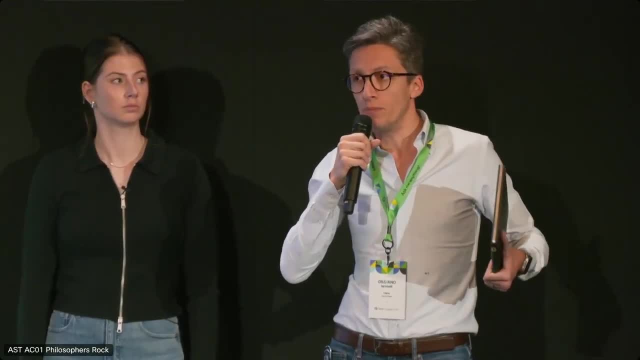 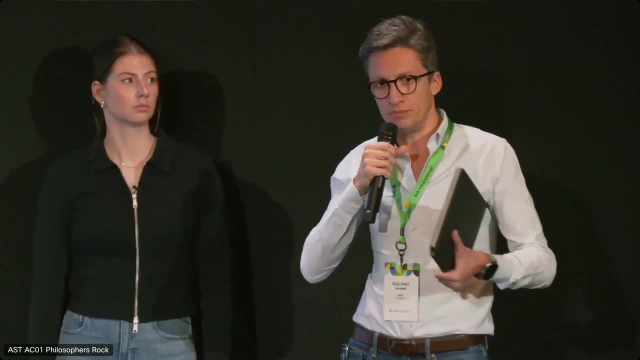 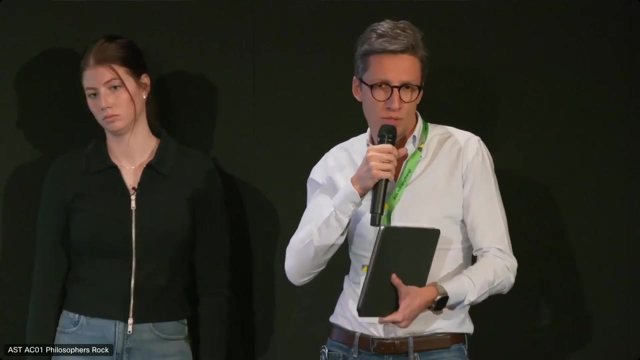 compared to FileMaker will be just an amount of actual views that you build with Studio that are shared for consumption with end users, Whether those are users that are already licensed on your FileMaker license, as you have right now, or they're anonymous guest users from public internet. 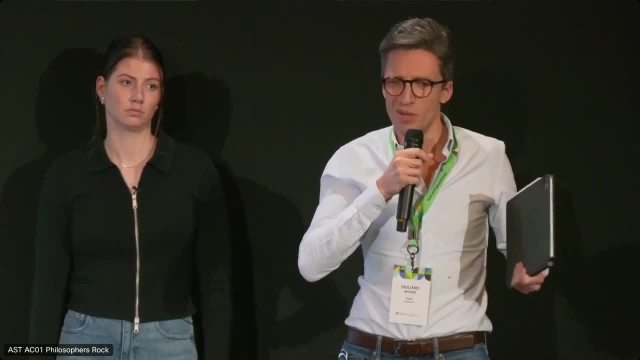 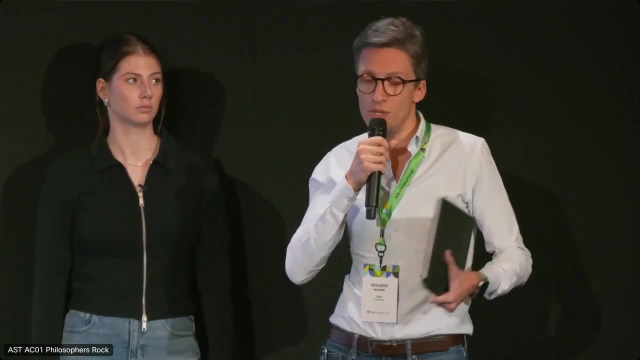 that doesn't matter to us right now. We want to make sure that we don't make the thought process of figuring out how much is going to cost too complicated And the benefit of Studio is built on an infrastructure that is multi-tenant is way more cost-efficient. 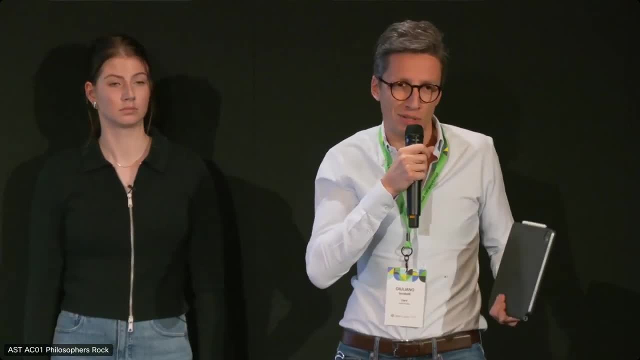 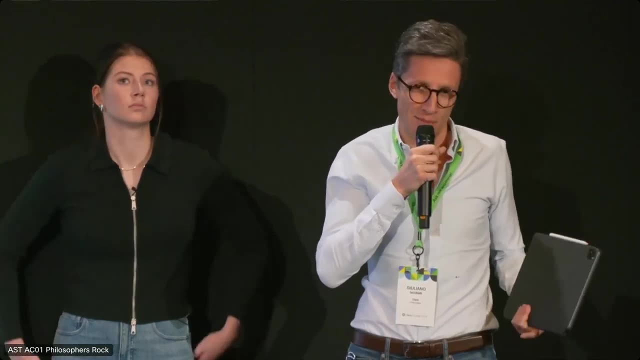 So managing traffic of thousands of users that makes a handful of access to read-only, or making some small operation by API interacting with web pages is not going to break the bank, So that's not a concern. So we have the opportunity to be a little bit more loose there. 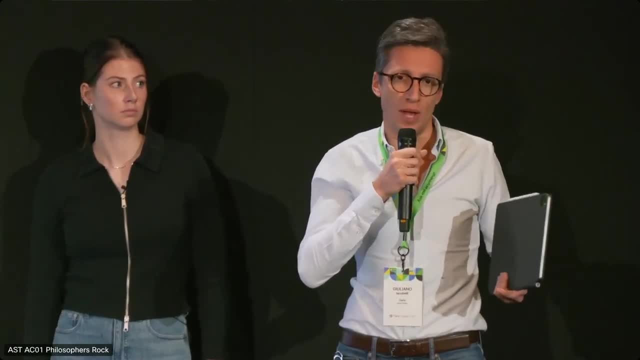 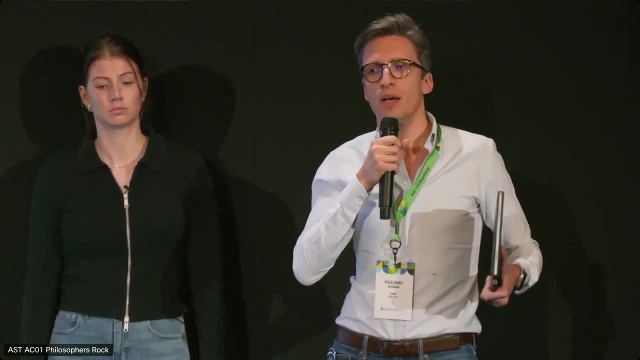 And then, based on the pattern of adoption that we're going to observe, we might fine-tune how we can best license that. But right now we'd rather keep things simple. The more we're going to get closer to a place where you can issue identity, so to speak. 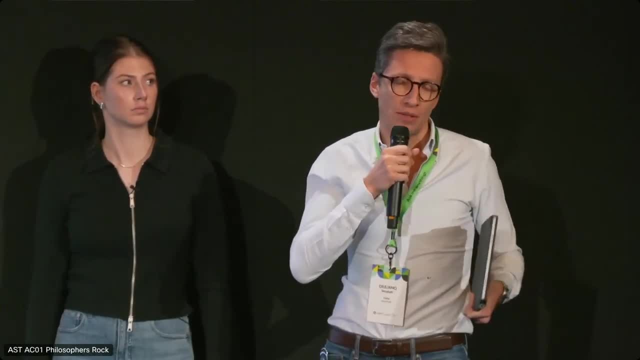 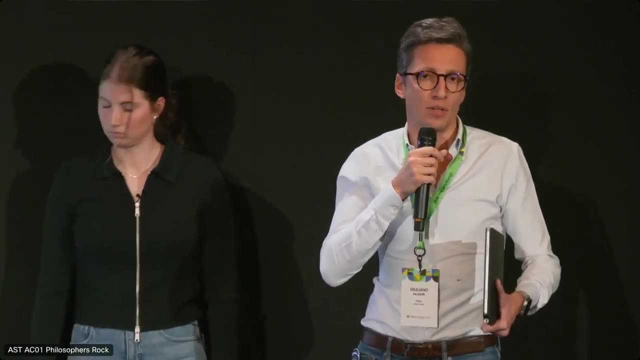 to external people, to your organization. I might expect that to be factored into the licensing maybe in some ways, but that's not there yet, So I don't have, I can't give you an actual projection right now, but hopefully they will become also more visible. 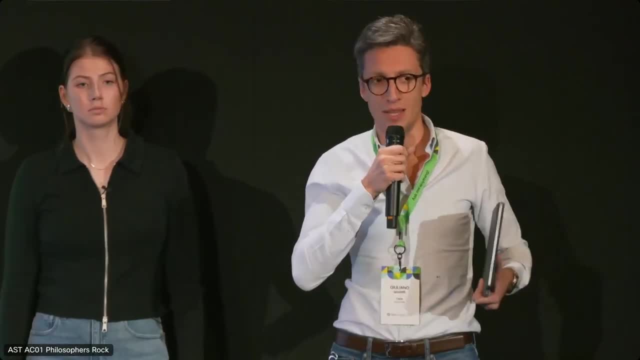 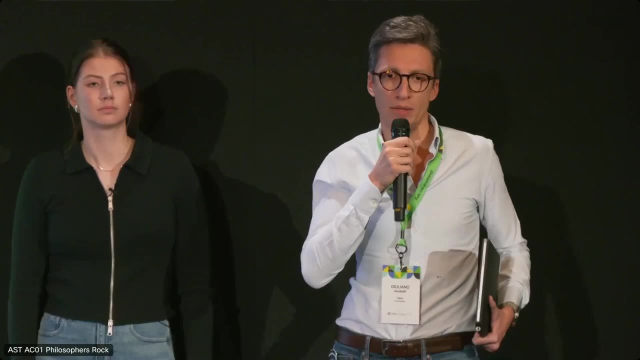 through the initiative that we have, Like the visible backlogs. As soon as that thing becomes more scoped by the team, it will become visible in there and all of you can engage in conversation with us to learn more about it, Because right now I'm on a turning point. 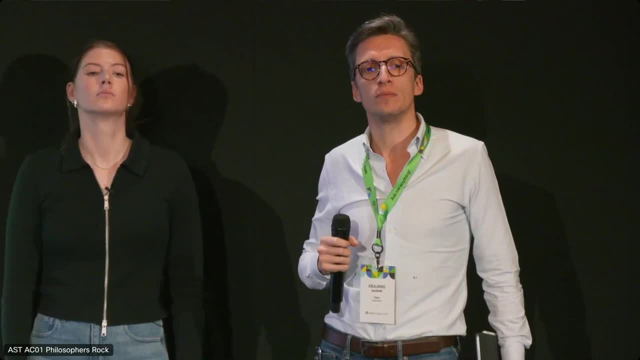 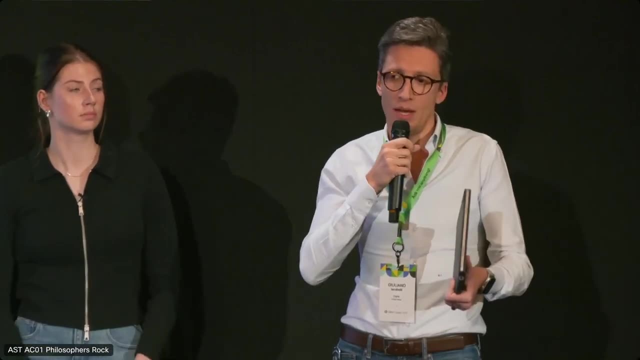 We have an efficient solution running PHP right now. I was trying to figure out if the studio can come in place for you to place this PHP solution halfway. Yeah, it might, And often with development in general, the answer is always it depends on how you develop. 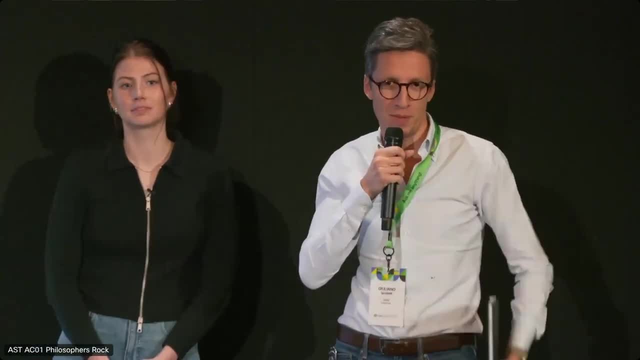 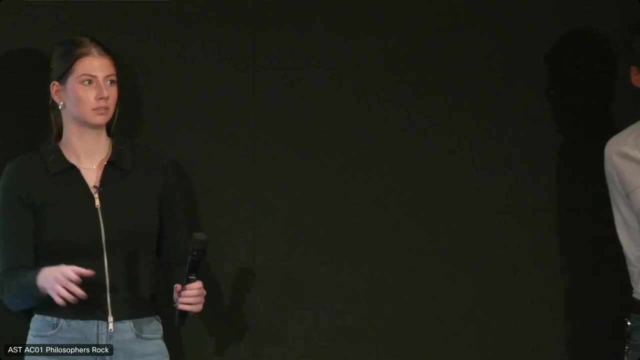 how you build the solution. I'm happy to swing by the boots and maybe get a little bit more into the weeds of a use case and talk through it. Thank you. Question: Could you speak to how and if it pushes data back and forth with FileMaker Pro, please? 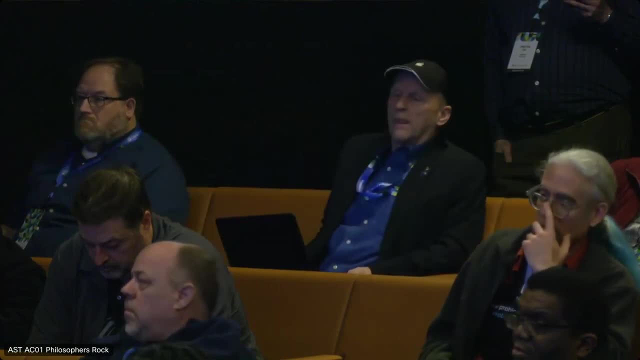 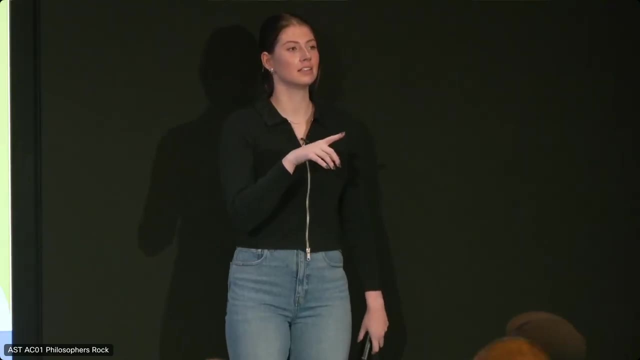 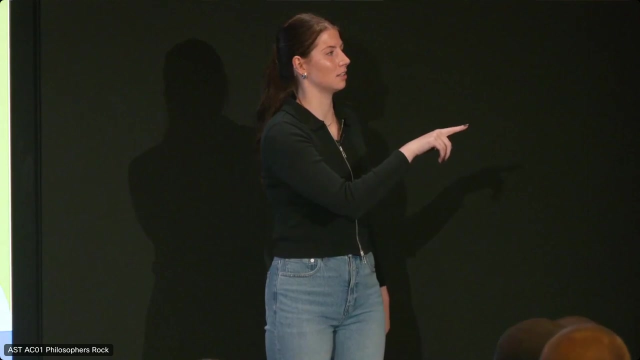 Yes, so Is my microphone on, Oh, okay, Yes, so the data from studio is migrated to FileMaker, and I think Louie demoed it in his session in the keynote and we'll be talking about it more in Connect. 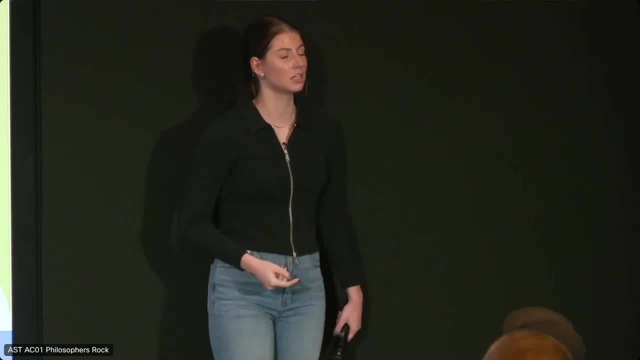 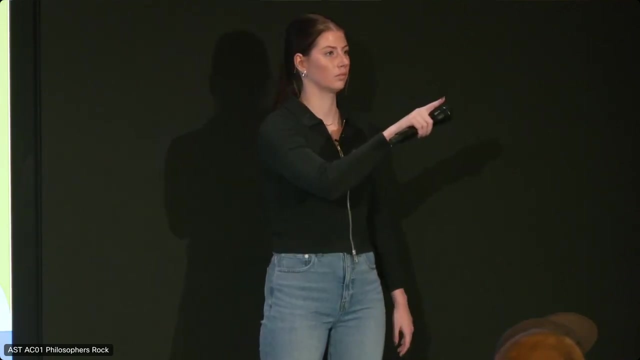 But you can add an external table, an external data source within FileMaker. that is your studio table and we're making that connection stronger as well with Querence Connect as we continue. Okay, Thank you, I just wanted to clarify something you said earlier. 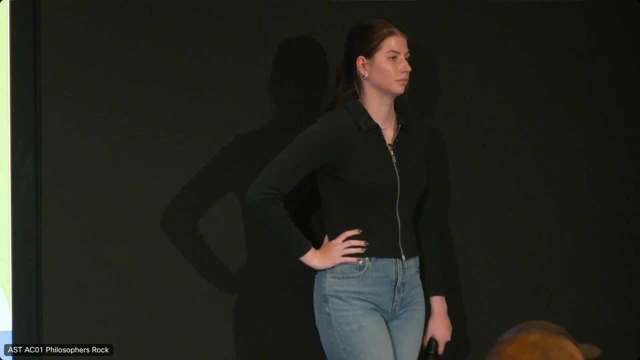 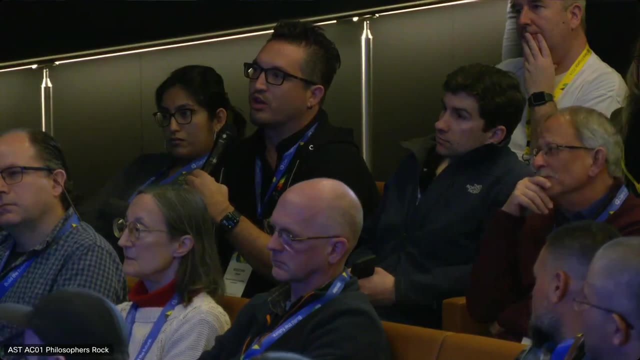 to make sure I understood it correctly: So if we have people that want to access these custom views that are external to the system, we could generate some sort of public IP so they don't have to go through the ClarisID login? Yes, exactly. 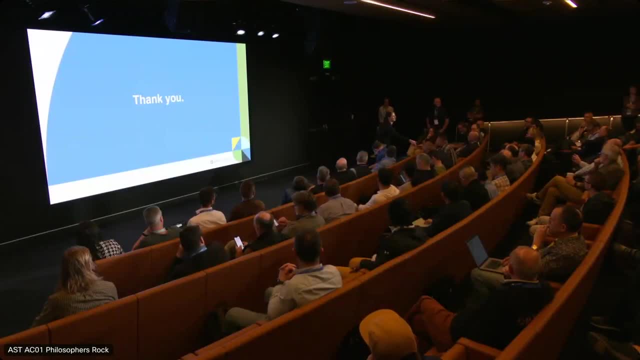 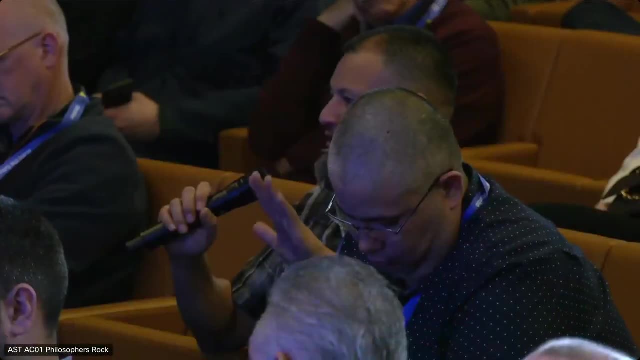 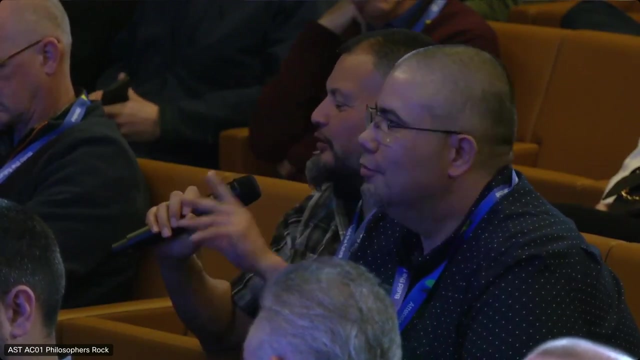 Here I got one. Sorry, You're next. So there's like these small little blurbs of Mongo right, MongoDB Mm-hmm. Is it using MongoDB in the background? Or like how? What's the connection between the MongoDB? 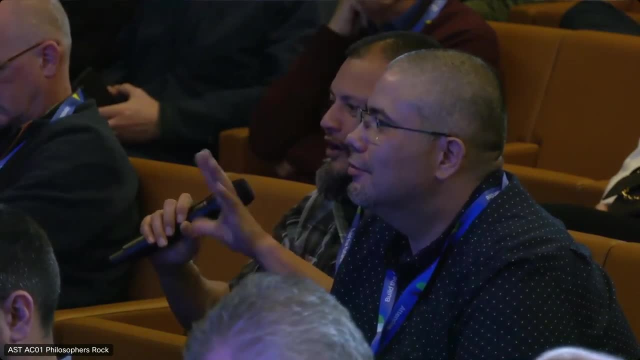 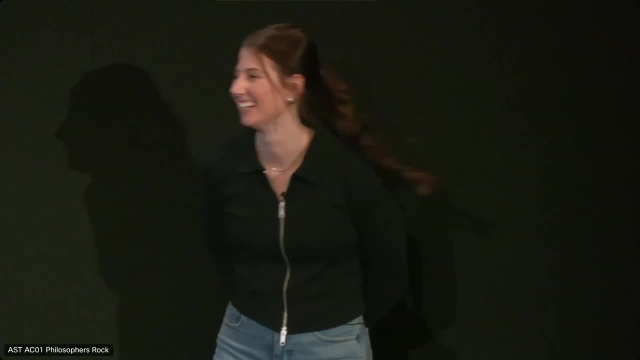 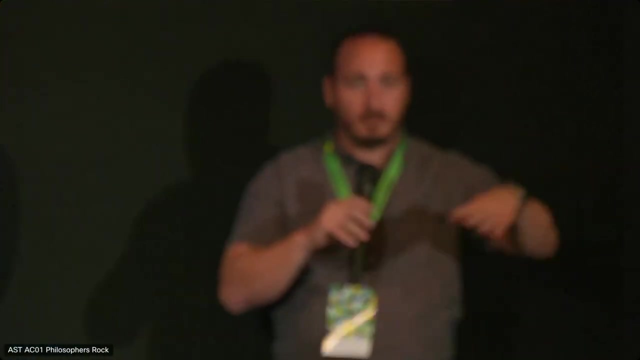 I've heard it a couple of times and I just want more on how they're using that. Yeah, Louie's going to say it more eloquently than me, so So as far as MongoDB, you've heard Peter talk about it. 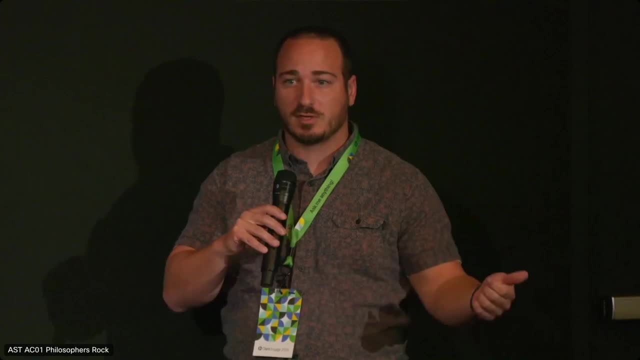 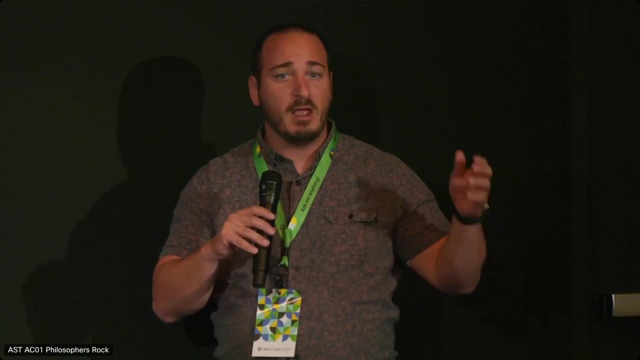 One of the things he gives us on studio, which is based on MongoDB, is the eventual consistency, As you saw in the keynote. it also gives us event-driven access that we didn't necessarily have before. So studio is supported by MongoDB. We do have an abstraction layer. 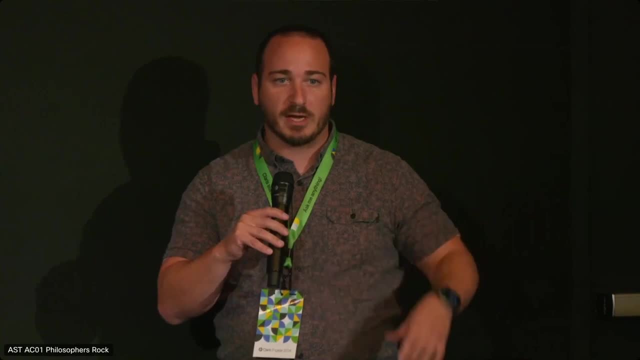 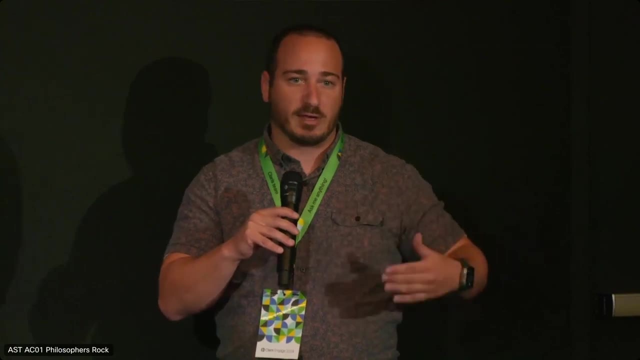 so we can swap out that database as we need drop out the storage layer. But MongoDB gives us the advantages of both scalability and then also being able to read in events right and act on things in real time. Will we be able to access that MongoDB directly? 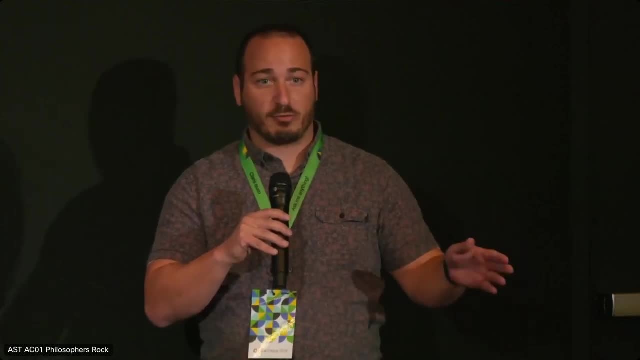 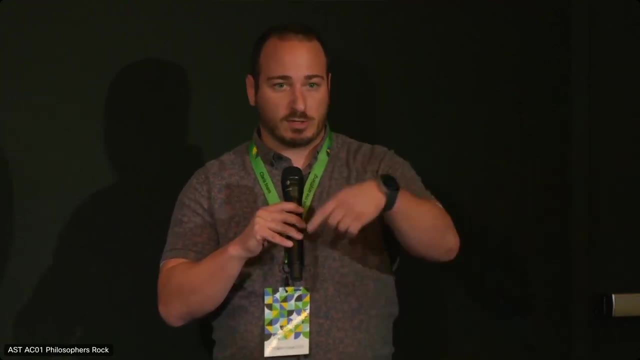 At the moment, I would say no, You can access it through either Connect or FileMaker. right, You can run scripts on your external tables, like you can today in ESS. You can also, if you come to my session, use a studio connector to actually access that data. 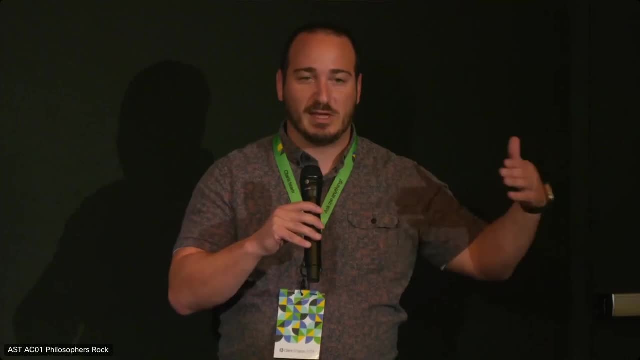 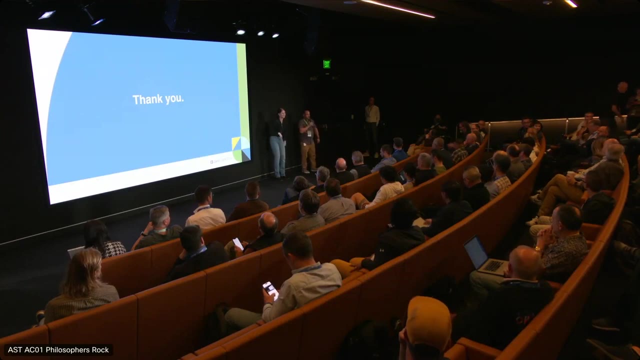 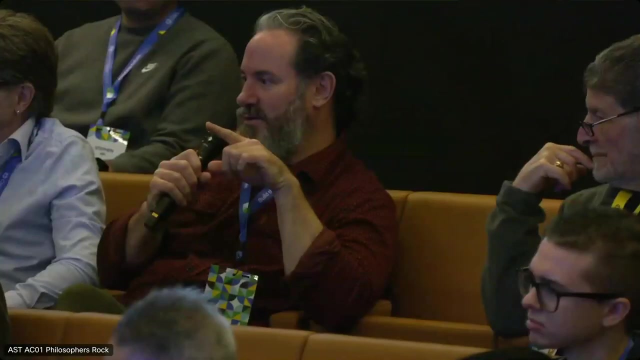 But, as Giuliano says, it does depend. The use case is long and we'll see where we go from here. Okay, Two for one, Love it. I was meaning to ask: what do you have in the CI, CD area and versioning to be able to control? 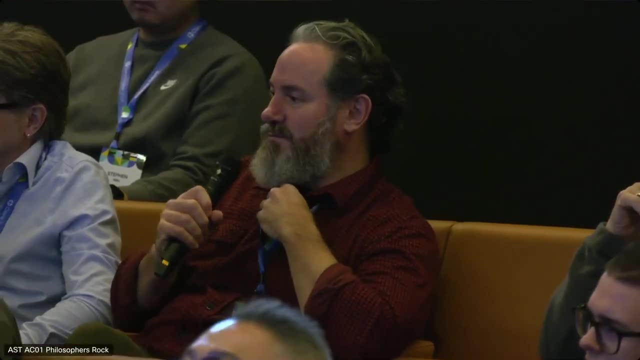 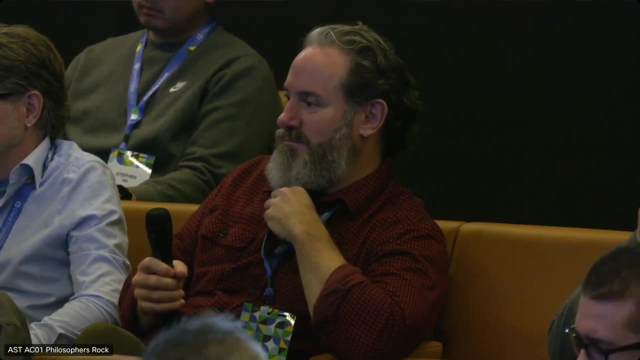 when you build these solutions. So the question was on CI CD, how do you control kind of development and rollout? I don't want to keep going back to my session, but for that I will as well. We do have some things in the works with the studio connector. 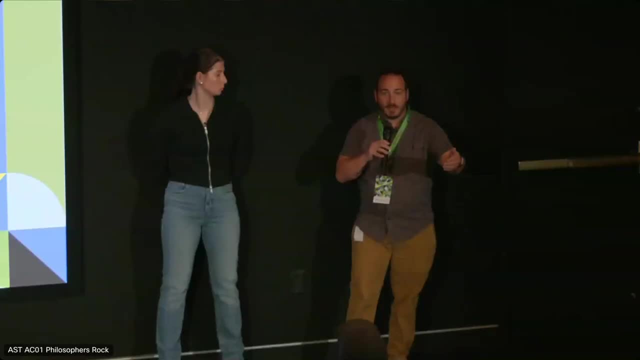 that helps you do that. I wouldn't say we're complete by any means. We are kind of iterating as we go, But there are things you can do to mock up a layout, make sure it works the way it works and then push it out as you need. 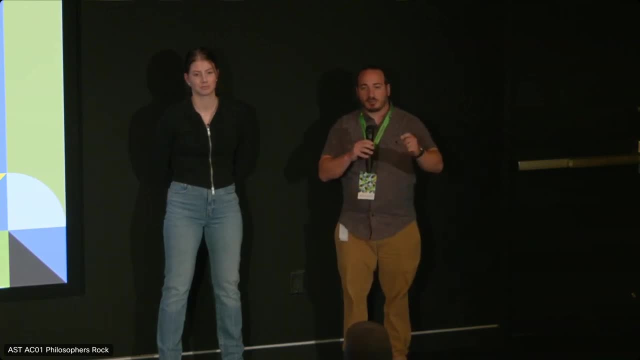 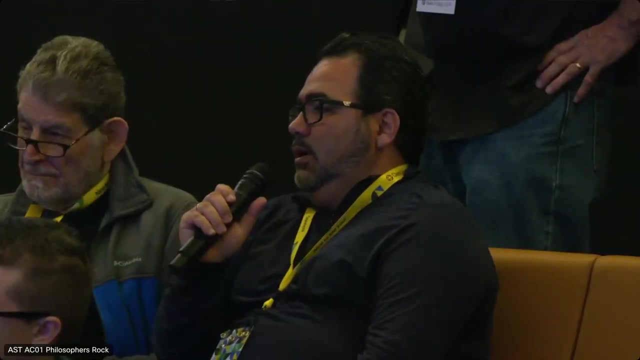 What is your session name? Cut Through the Chaos with Klairs Connect Thursday at 10.30.. Got a couple questions. One of them is related to: can you add data sources for multiple FileMaker servers to the platform? You can pull a dashboard that actually. 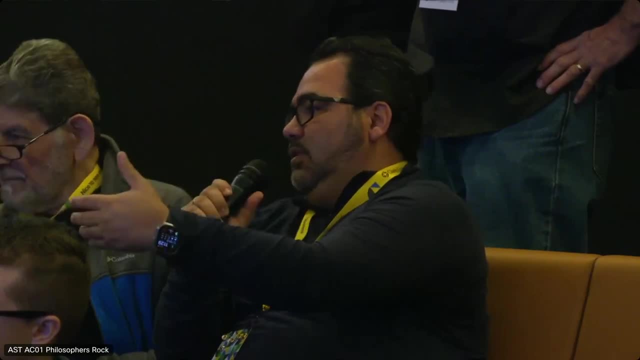 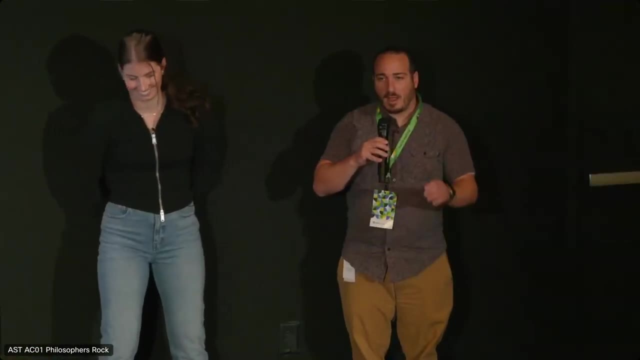 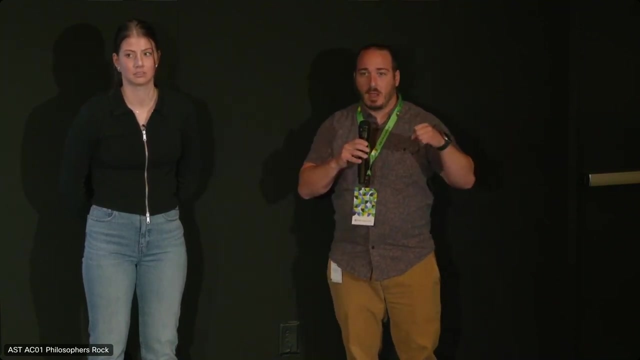 pulling data from one FileMaker server and the other data sources from a different FileMaker server. Sure, I'll answer that. I think pull might be not the right term to use. I don't know if it would necessarily reach into FileMaker and pull the data out.